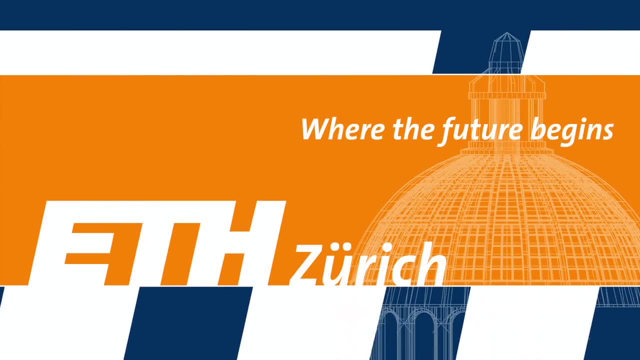 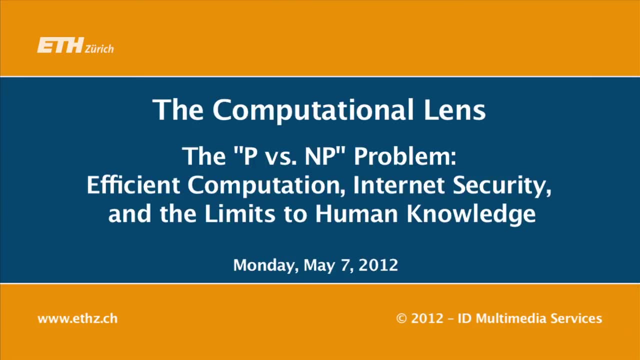 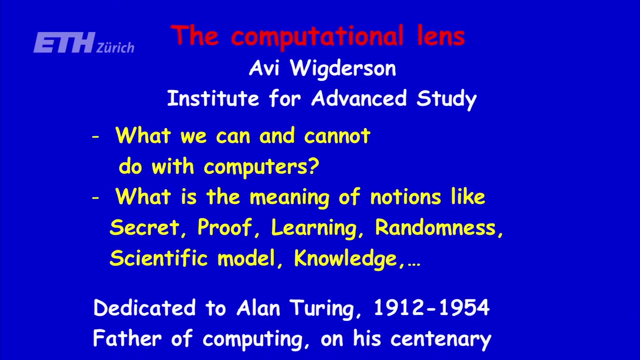 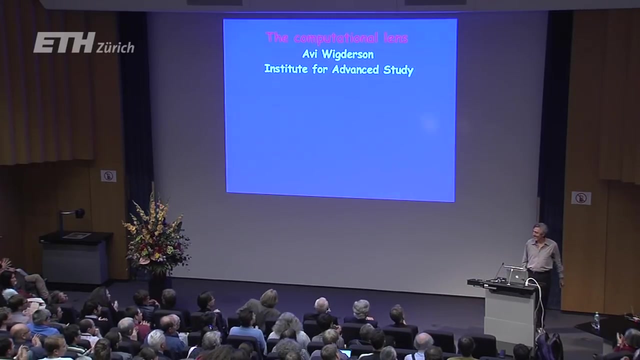 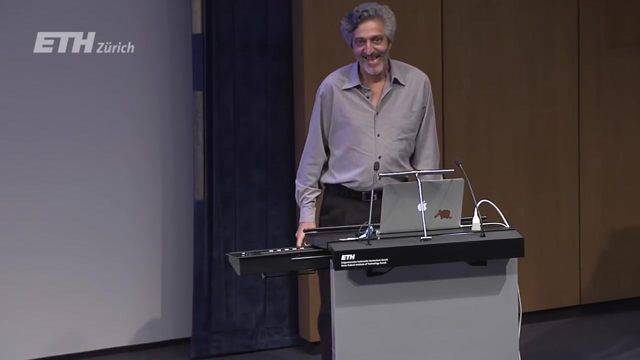 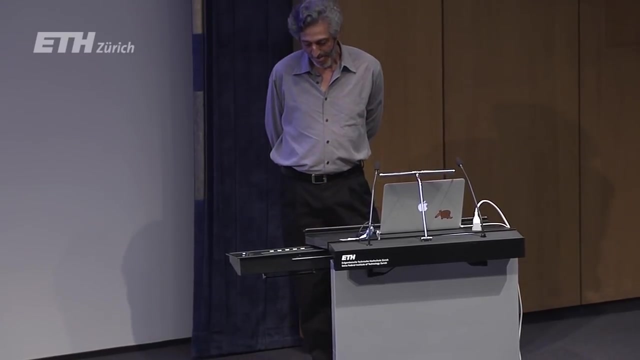 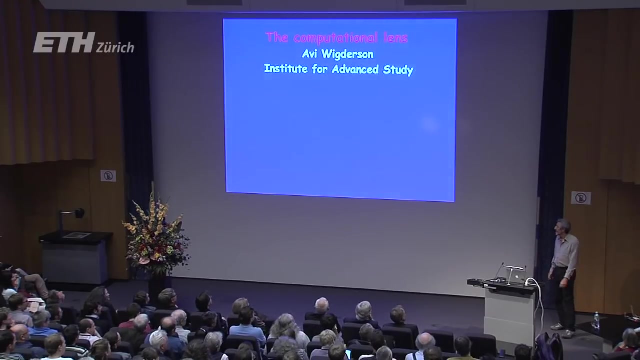 I will also speak in English. Hi, The alternative is Hebrew. of course, I'm really happy to be here. I'm starting today a series of three lectures on the computational lens. I remind you what was in the poster. I remind especially those who are not here that the three lectures, even though they 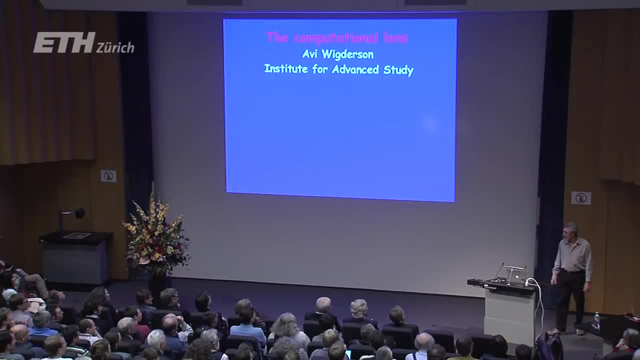 have a common theme. they are independent, so I will try to at least make them fairly independent. The basic question from which everything starts is what can and cannot be done by computers. but as you will see as this week unfolds, even today, that these 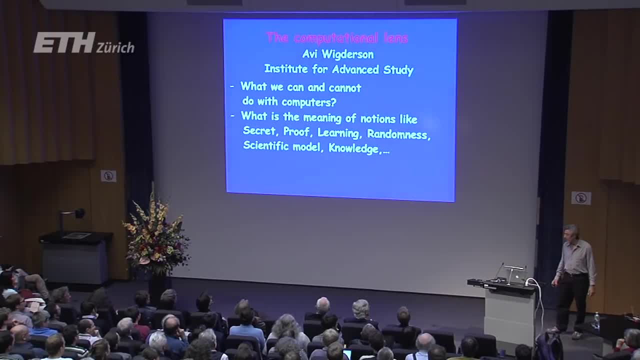 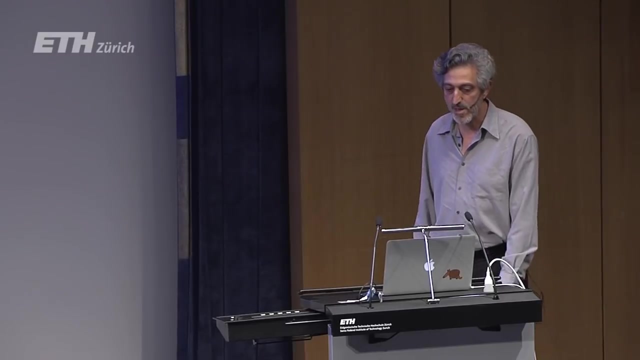 questions lead us to very different, much more general questions in understanding the meaning and providing the meaning, Providing meaning to lots of very basic concepts that people looked at for I don't know: millennia, Secrets, proofs, learning, randomness, basic scientific models, knowledge, And we'll see. 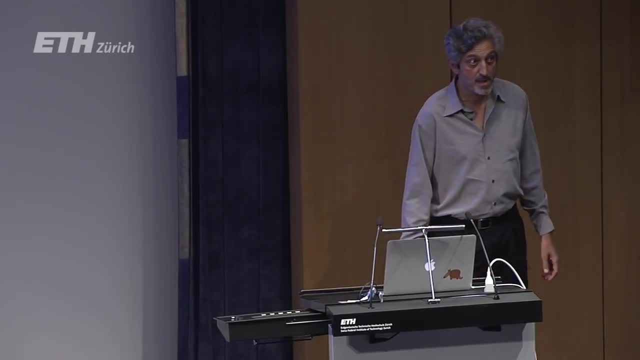 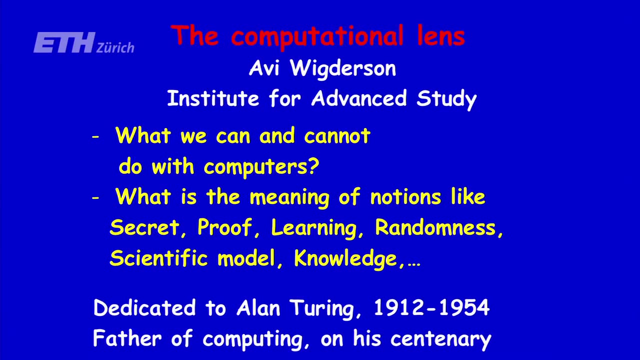 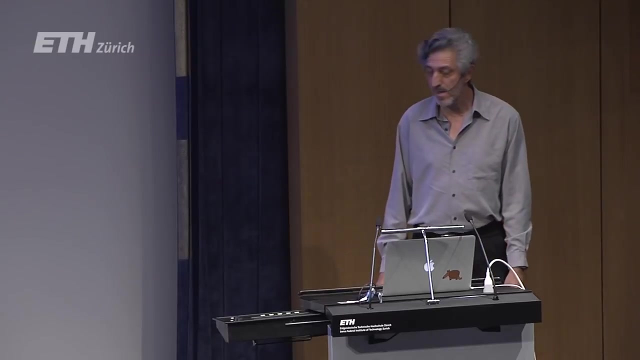 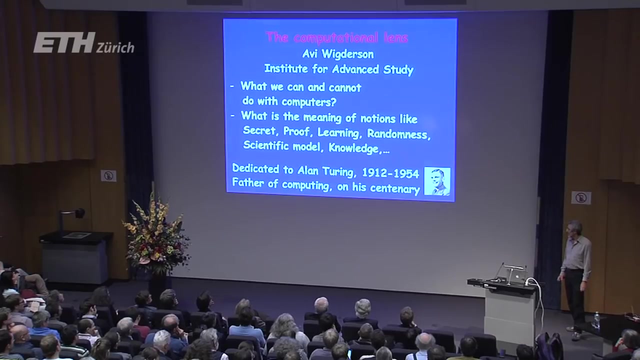 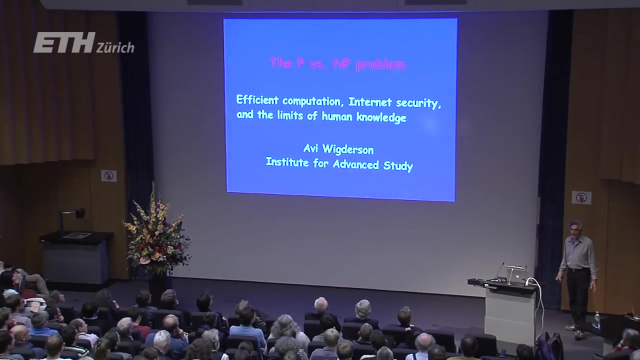 how the computational lens offers this new viewpoint. This year marks the 100th anniversary of the birth of Ellen Turing, and I would like to dedicate this series of lectures to him. He's the father of computing, as we'll also see, So let me try to start today's talk. Today's talk has a very bizarre title for those of 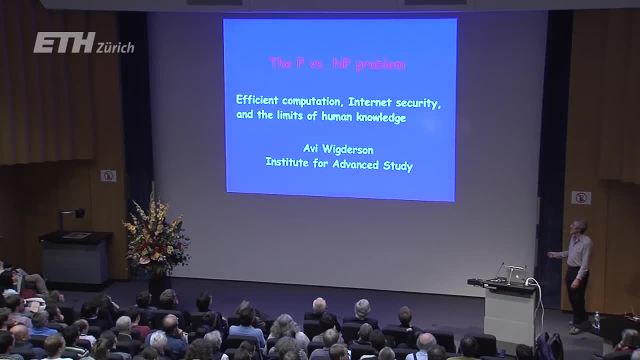 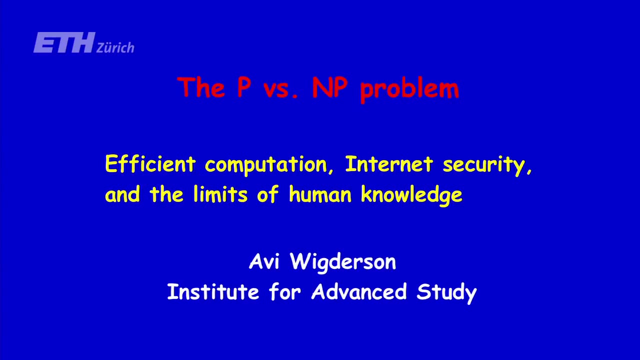 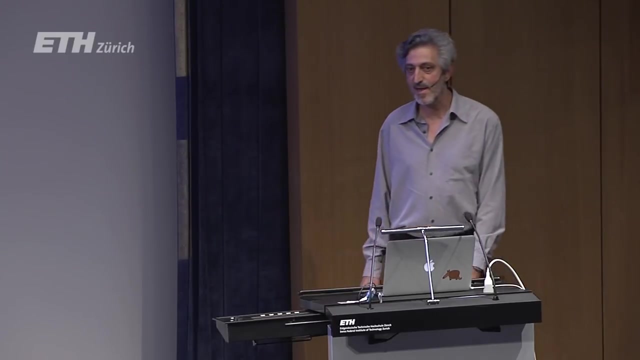 you who are not computer scientists. It has two strange things there: the P and the NP. It's about the P versus NP problem and that's what I have to explain to you today. What is this problem? But you can see from the subtitle that at least it tries to touch a lot. It's about 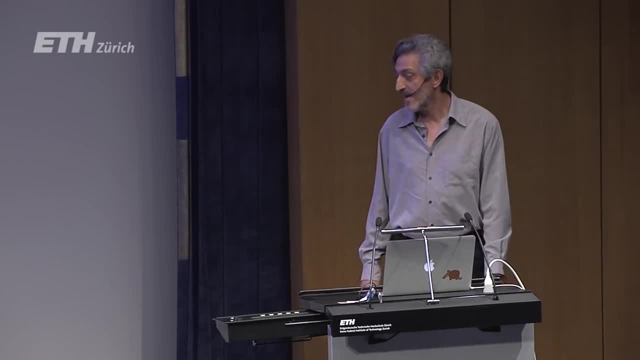 efficient computation, internet security and, believe it or not, the limits of human knowledge. You can later confront me of that if you need that. Okay, so I'll try to explain it all, But let's start from the problem itself. So the problem. 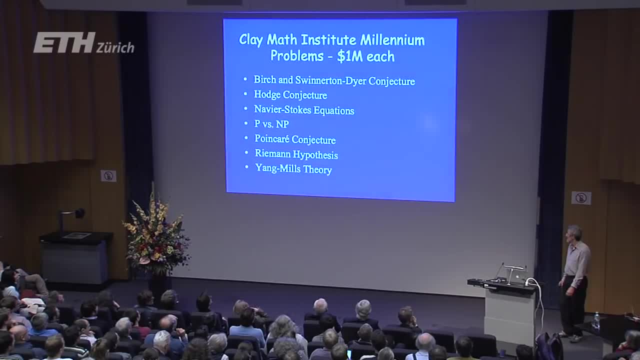 itself is that the technology and technology can be used to create new problems, new solutions and new solutions, And you can imagine that this technology has been used for such a great many reasons. In the research, there have been many experiments where the technology has been used to solve. 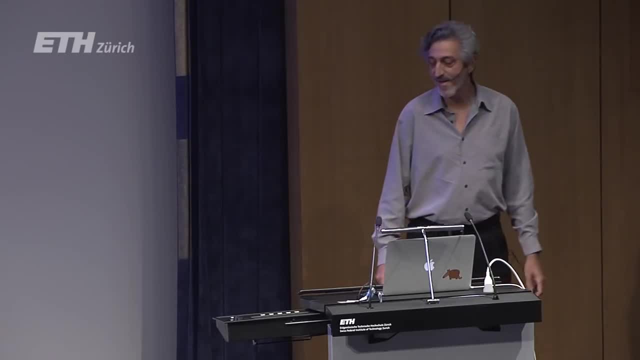 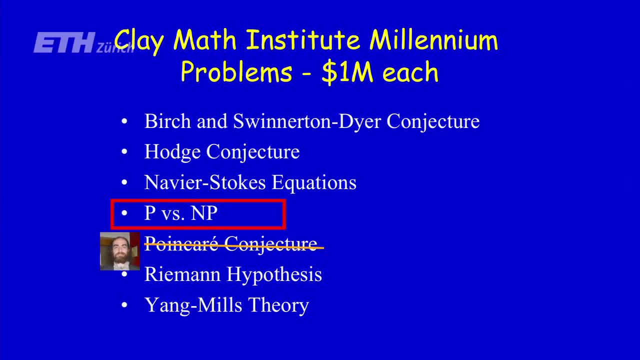 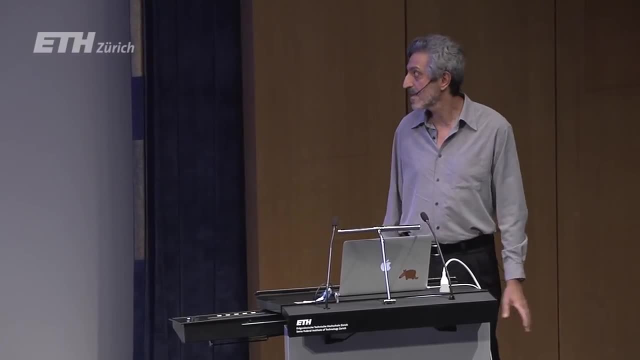 If you want to do it you better hurry, because one is already done. But you see that our problem is here smack in the middle. So mathematicians somehow deemed this problem, which is a computer science problem, to be one of the seven most important problems of mathematics. 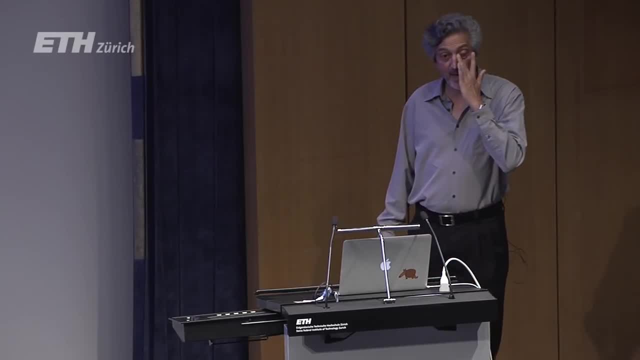 for some set of people. I'll try to explain why it is important to me, to computer scientists and to scientists in general. So, to do this, I want you to read. I'm going to give you now the slide, after which you can go to sleep. 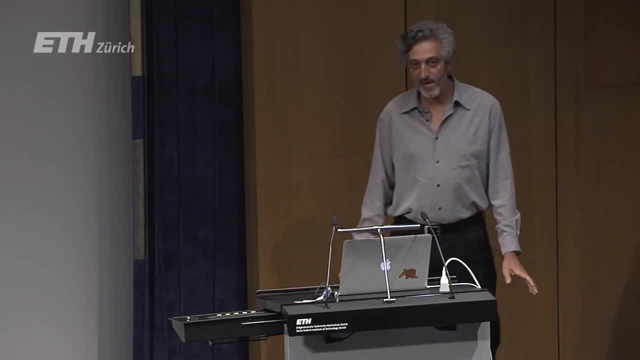 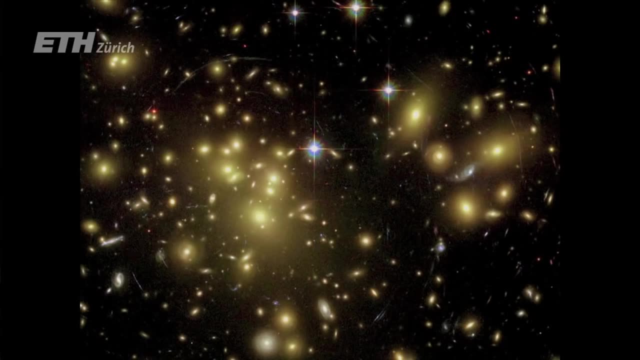 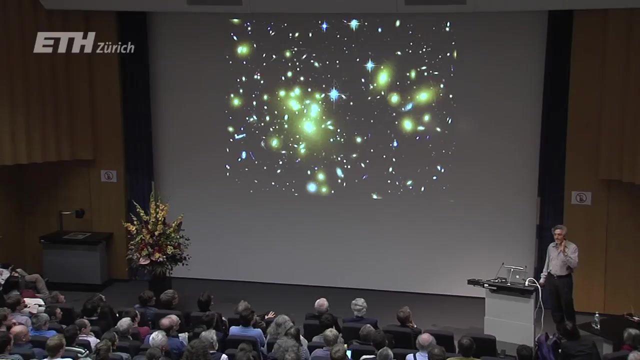 So I'm going to just in one slide, explain what P and NPR are and what is the question about them. So, this night sky, this view, you should take the stars here as representing computational problems, your favorite computational problems, And we are doing it. 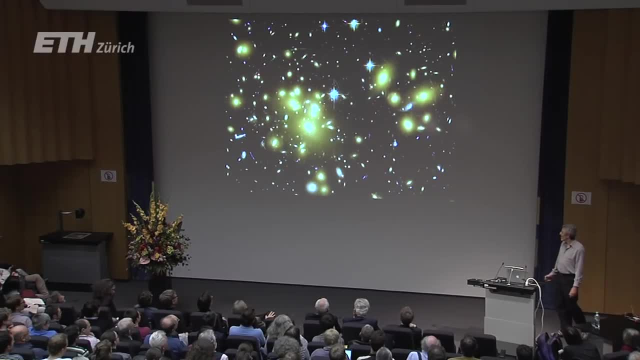 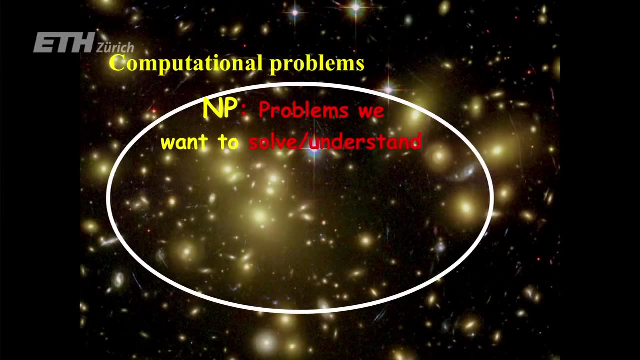 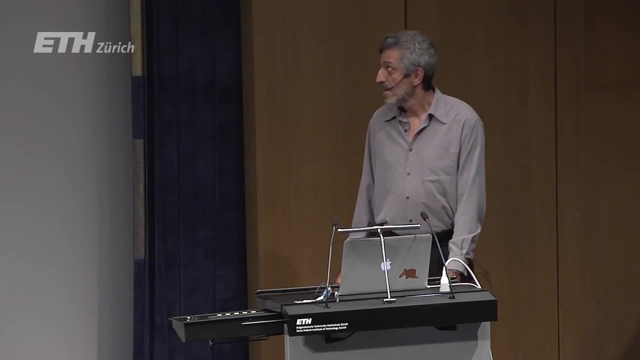 And we are doing it. We are trying to make sense of this world And in this world there are the problems. NP represents the problems we want to solve, all the problems that we want to solve and we have a chance of solving or understanding. 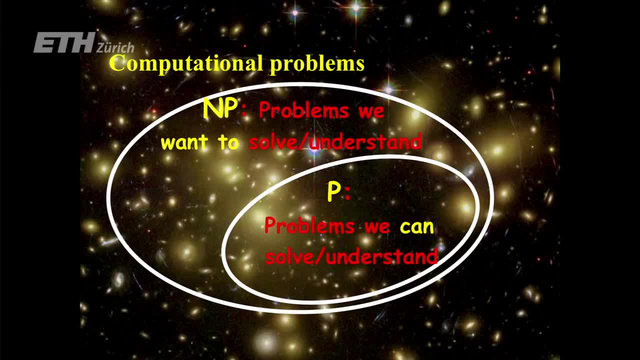 And within it there is a subset P. we call it P- of the problems that we can solve And in fact you'll see in the In the talk, the computational problems actually capture lots of other scientific, mathematical, intellectual problems. 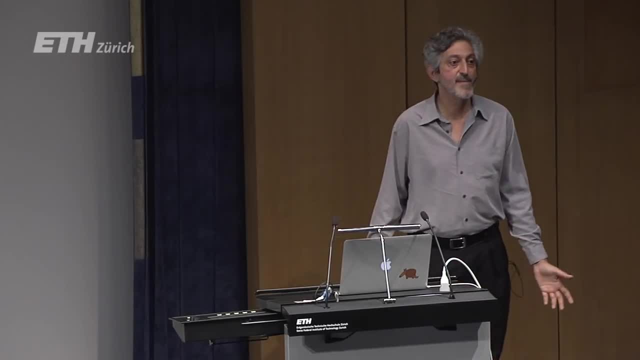 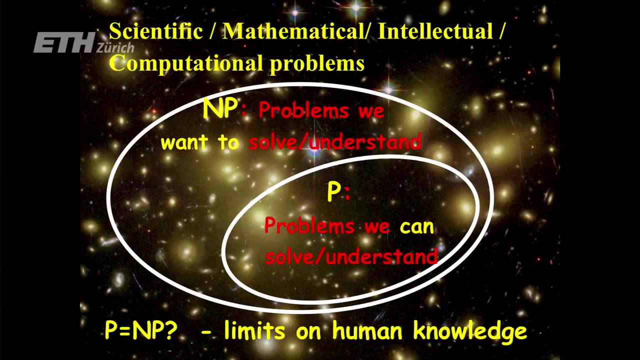 So the question of whether P equals NP is whether we can solve all the problems we want to solve. So that's the P versus NP question. I'll try to explain why it's, you know, even though it sounds maybe philosophical or undefined. 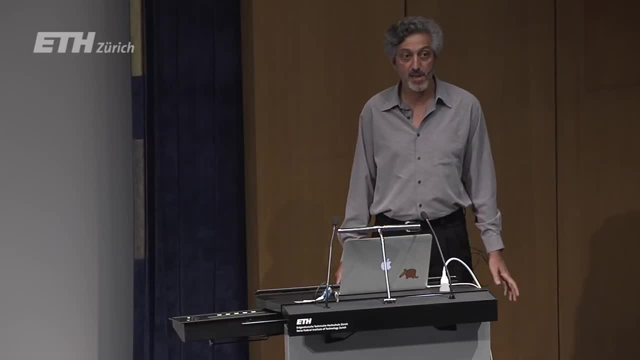 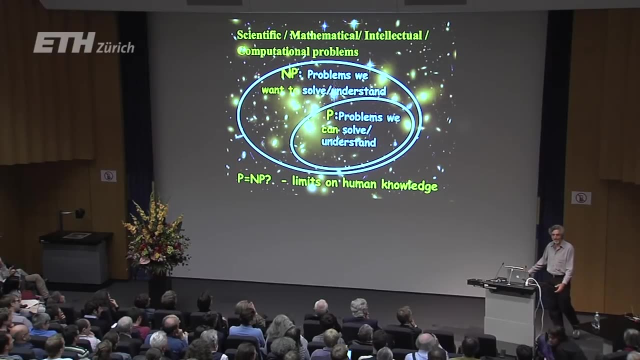 this is a mathematical question, well-formulated mathematical question, So you can make sense of this In mathematics terms. then you can well prove either that they are equal, that they are not equal. We don't know how to do it yet. 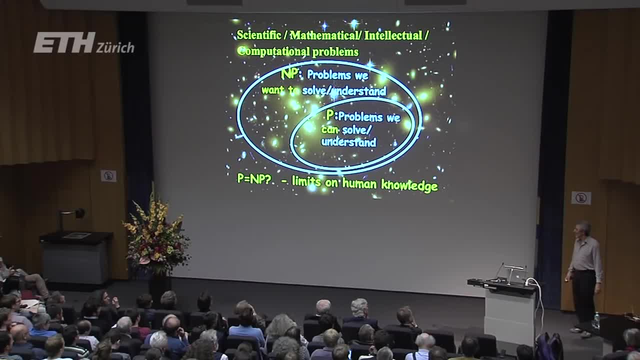 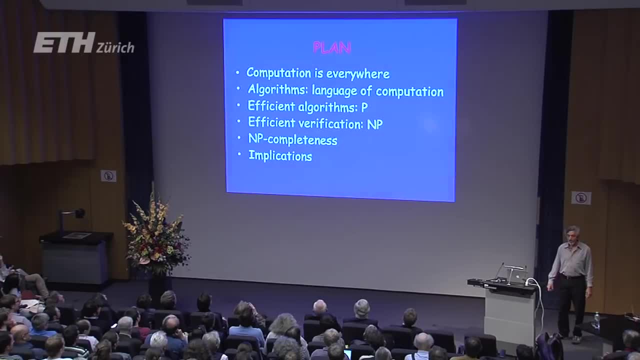 That's why it's a problem, But hopefully you'll understand why. you know what it is and why that's what it means. Okay, so it's a full hour. It's a full hour. It's a challenging hour And I'll try to go through it. 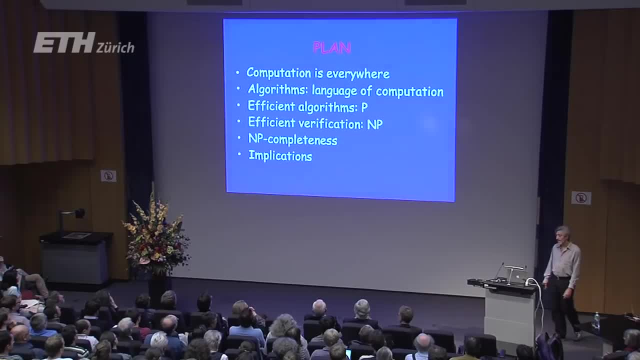 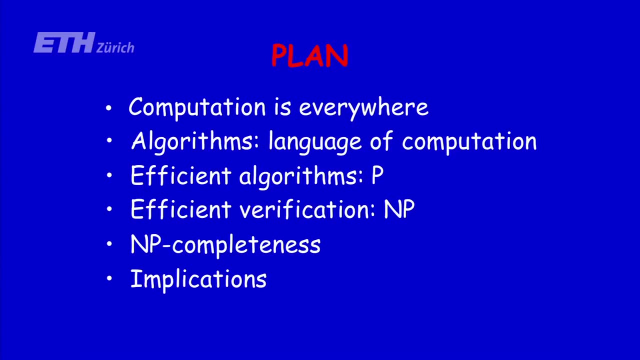 Hopefully things will be clear. I'll start by. I'll start by talking about understanding computation much more generally than maybe you are used to, than things that happen in your computers, And then we'll move to definitions and Turing definition of the algorithm. 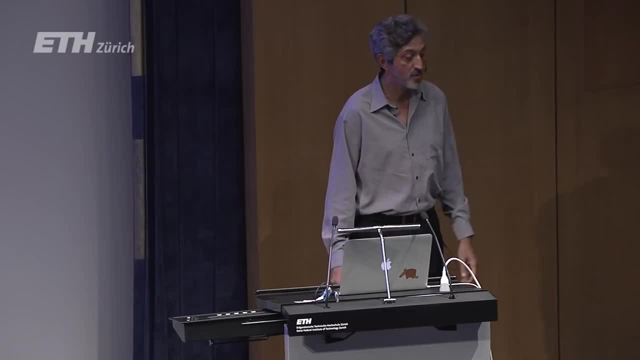 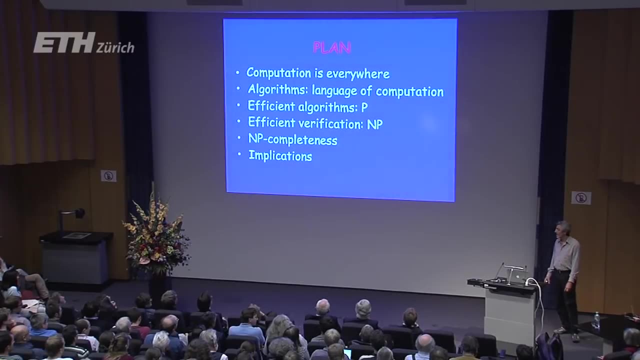 which offers a language, a mathematical language, to talk about algorithms and to analyze them. And then we'll define these two classes: the class of efficient algorithms- P- and the class of efficient- verifiable- you know problems- which is NP. 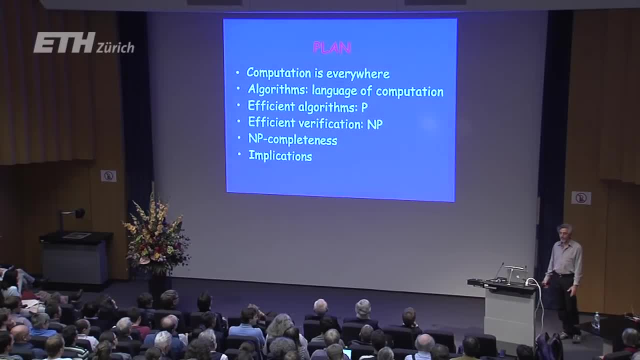 And then, as we don't know how to solve the previous NP question, we'll talk about our currently only access to it and actually to understanding the importance of the problem, which is this notion of NP completeness. I'll explain this and then we'll talk about implications. 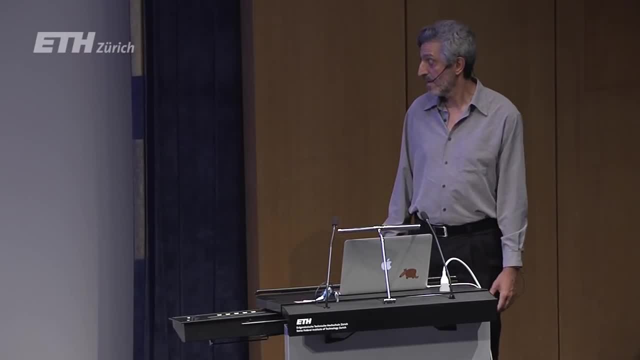 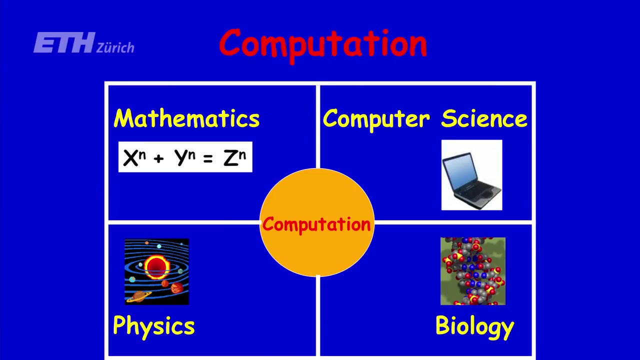 and of the question and what it means, what it means for our life, in fact, and what it means for scientists. So that's the plan. Let me start with talking, just very high level, about what we mean by what you should, I think, really understand. 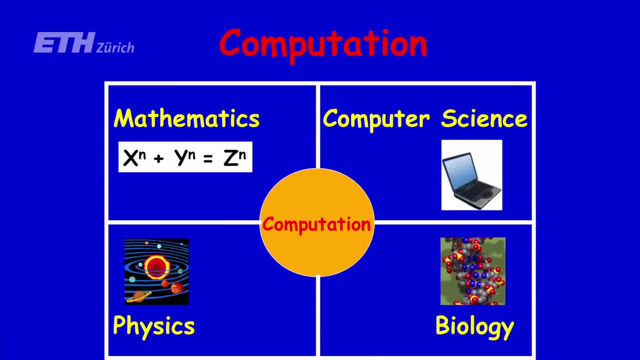 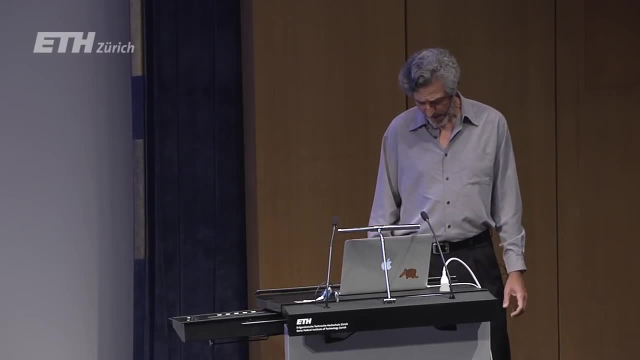 when the word computation is meant. So it's not just this, but it's things that have happened in very many other disciplines. So I'll just give you a bunch of examples, and they will all follow the following definition: You should think of computation. 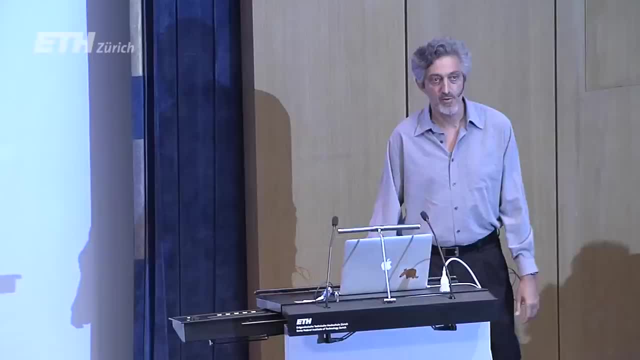 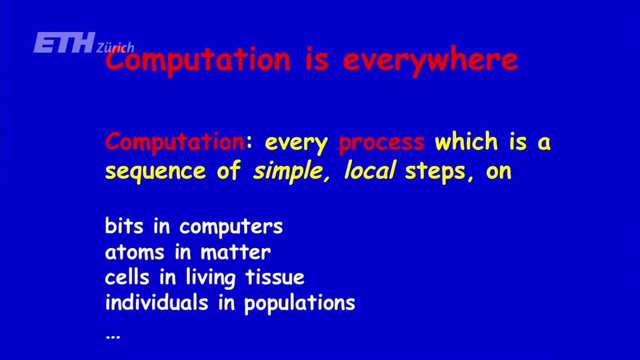 just sort of abstract away from what actually is happening in your computers as a process in which there is just a sequence of simple local steps. And in the computer these simple local steps happen on bits, on binary digits, on digits. It's a digital computer. 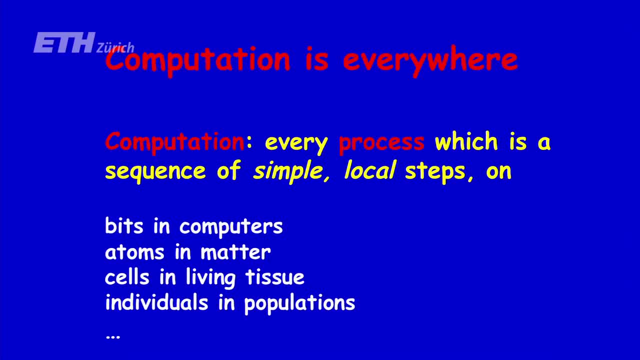 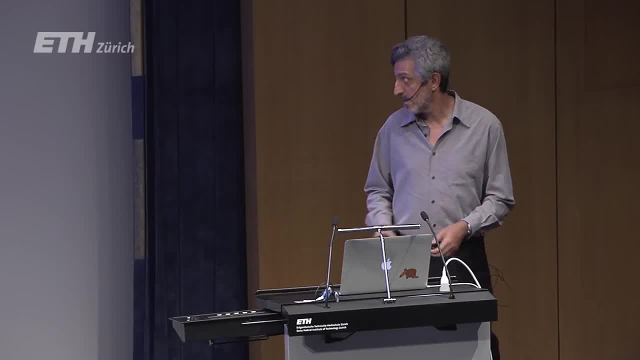 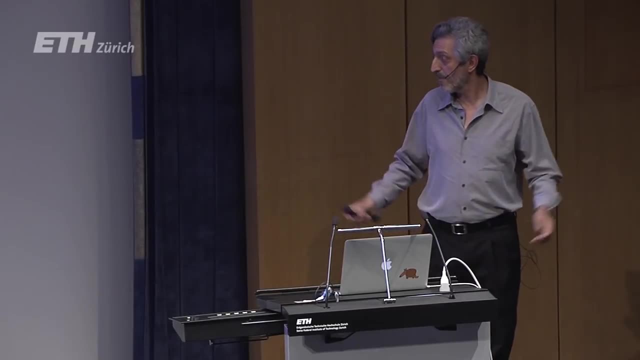 But you should just extrapolate and think about local interactions of atoms in matter, or interaction between cells in living tissues and life forms, And you can think of interactions between individuals in big populations. So you can see where I'm going, but I'll just give a few examples. 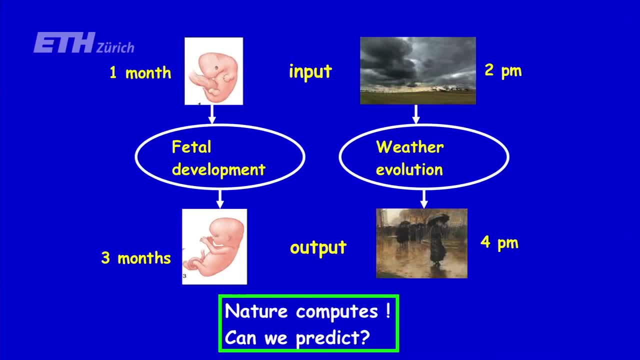 So one example is just natural phenomena. So you can really almost any natural phenomena you can cast in this term. that is the way we humans are trying to understand Natural phenomena. we are trying to understand the laws that transform a baby evolving in his mother's uterus. 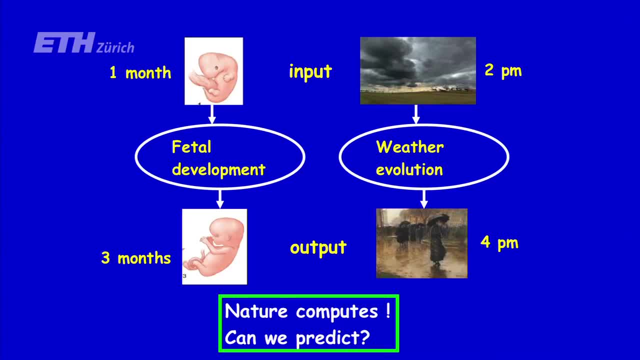 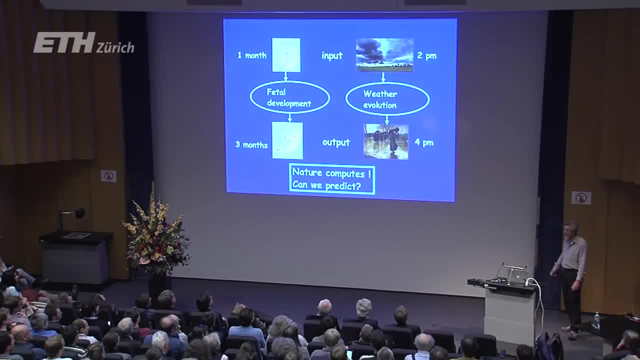 that produces these enormous changes: global changes through a sequence of very, very small interactions, like cell division or the way weather evolves and how we can predict it. So when we look at natural phenomena, there are actually two computations: One that's actually taking place in nature. 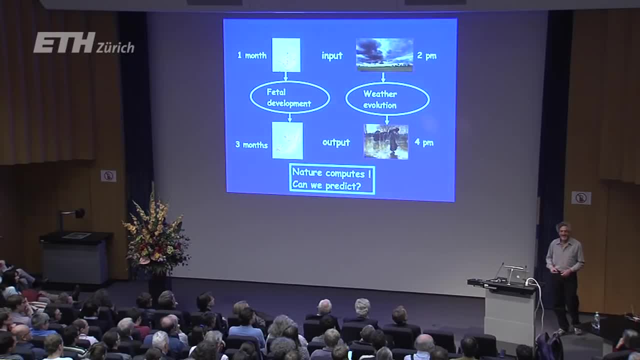 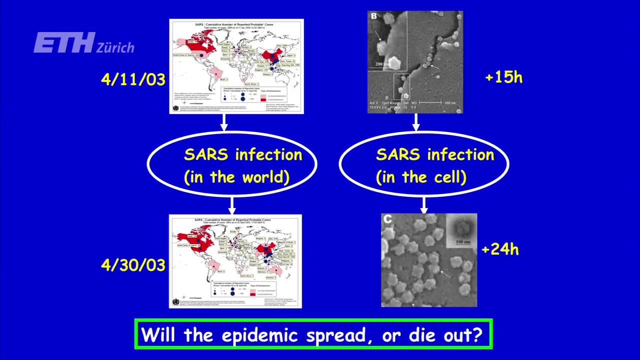 and the other computation is maybe our computation of the model, trying to explain it and predict it. When I say local, simple rules, you know, of course it depends on your scale- The same phenomena, like some epidemic, like the SARS epidemic. 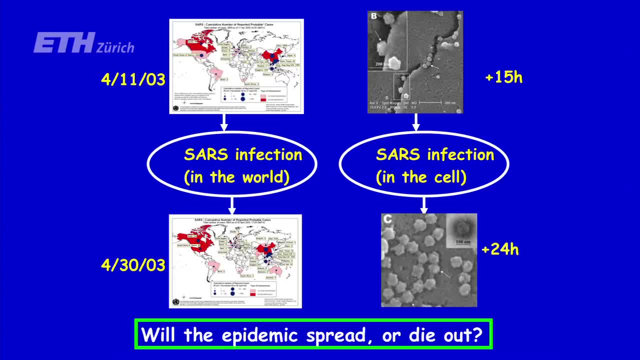 so swine flu or whatever can be understood at many levels, including the examples in the previous slide. You can see you can view how people infect each other on the left or how the virus you know develops inside a particular cell. 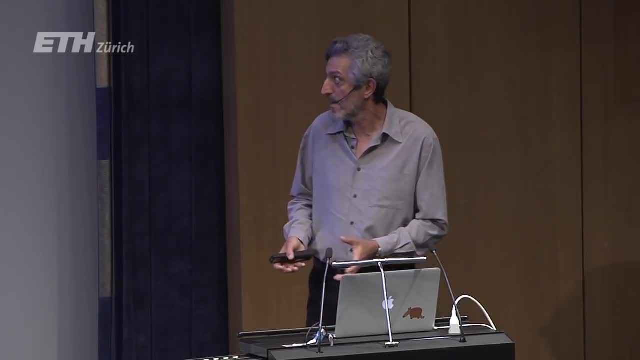 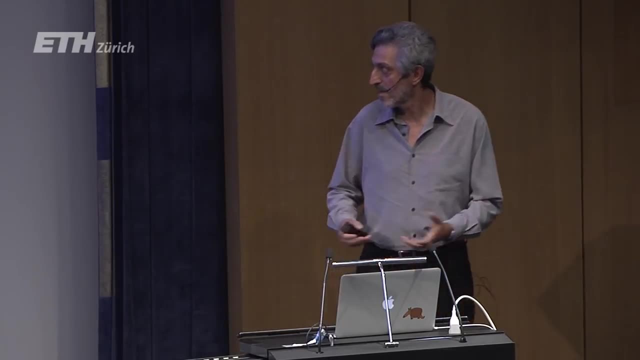 But in all of them, even if you have the basic understanding of the epidemic, in this case you can ask global questions like you know. what's the best medicine, or will it, you know, kill us all or just die out by itself? 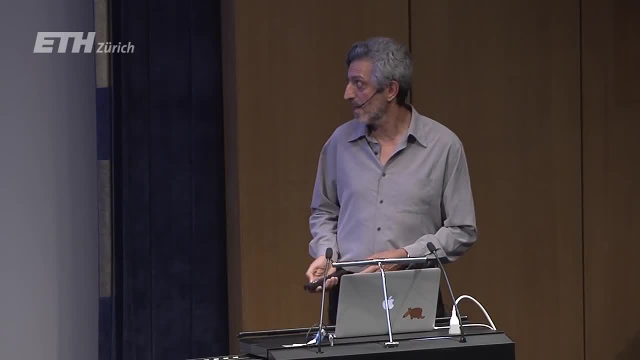 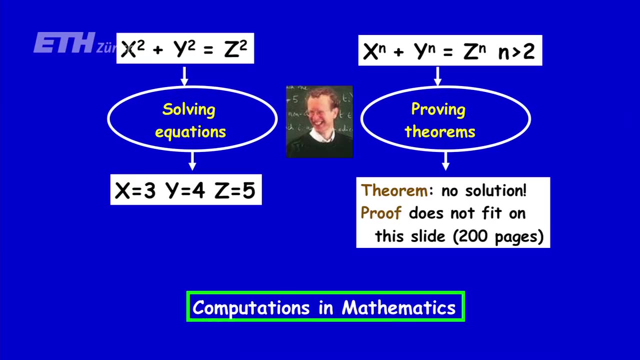 So there are global questions about computations for which you know the answer is not clear and we'll talk about this. Of course there are computations that happen more. you know, when you start learning mathematics in first and second grade, you learn to perform some computations. 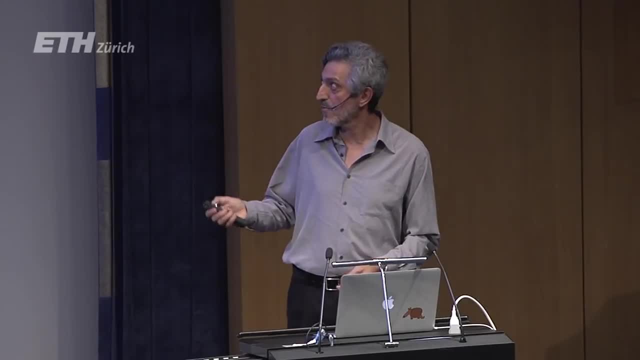 So we have, you know, we add subtract and then we start solving equations. And when you become mathematicians you actually start doing more complex things like actually prove theorems. So there are a variety of computations that happen in mathematics also there. 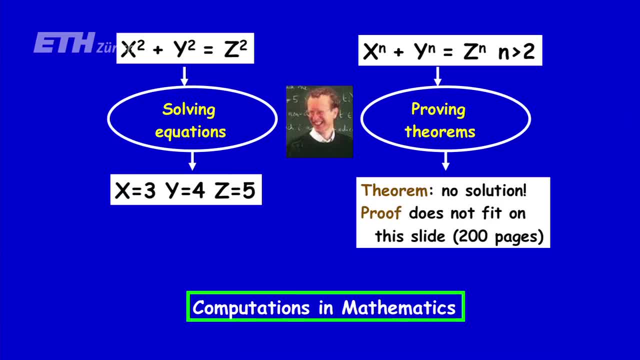 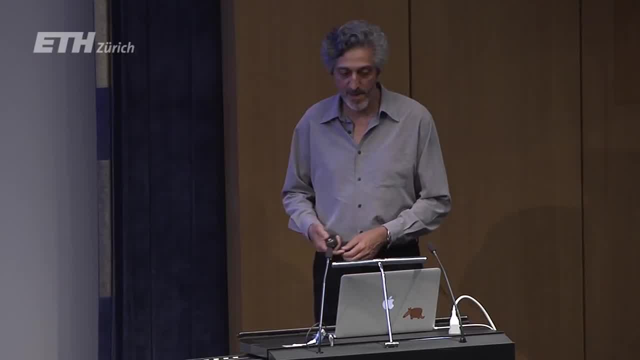 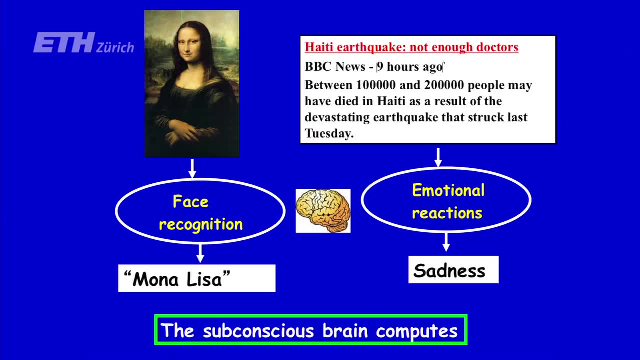 both in the computations and the proofs, There are sequences of very simple local steps that produce these magnificent objects, like the proof of Fermat's theorem, And there are other things that happen in our brain that are more automatic or subconscious, like our ability to recognize faces or our ability to you know. 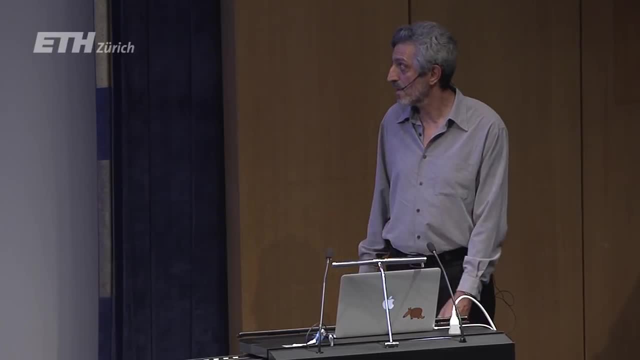 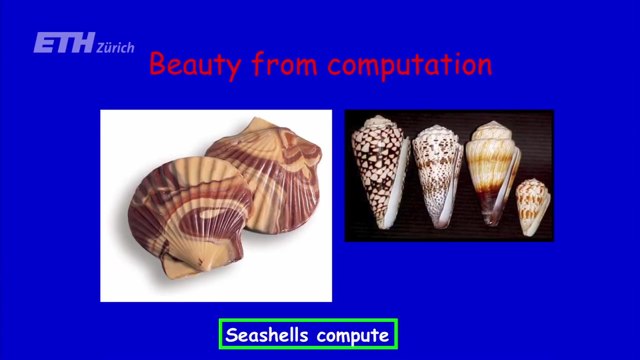 react emotionally to information that we receive. These also are, you know, happening in this collection of neurons under our skull through some kind of complex but local interaction. So also there computations happen. And I can go on and on. Yeah, you get also nice things from very local, simple computation. 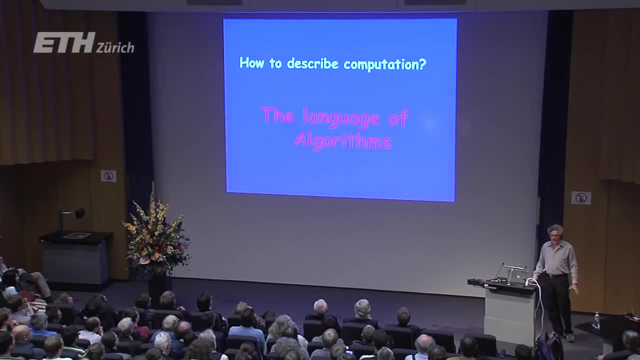 So now that we've seen some examples- and it's such a, you know, universal phenomena, computation- we better have some concrete way of talking about it, arguing about it, you know, proving things about it, And to do this we need the language of algorithms. 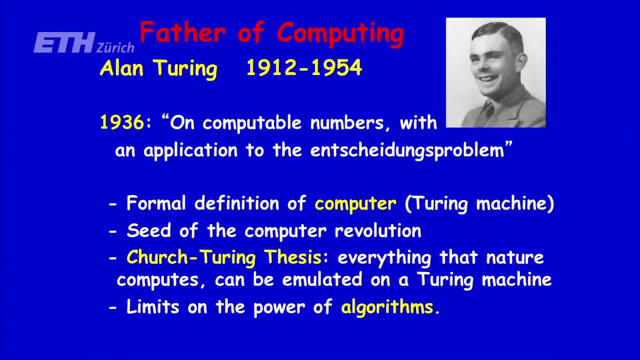 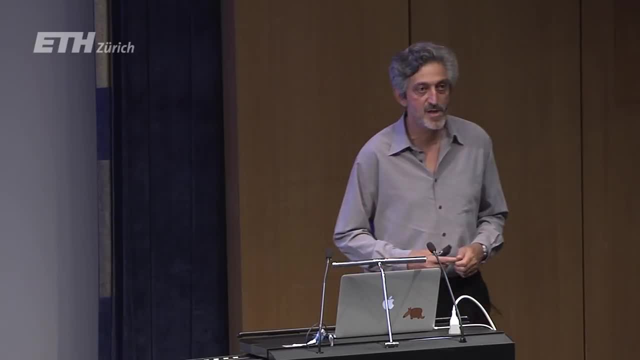 So let me tell you some about this. It really burst into existence in one paper in 1936 by Alan Turing, who was 24 at the time, a graduate student. So for all of you graduate students at the time time, this should be a good model for a PhD thesis, because that's what happened in this. 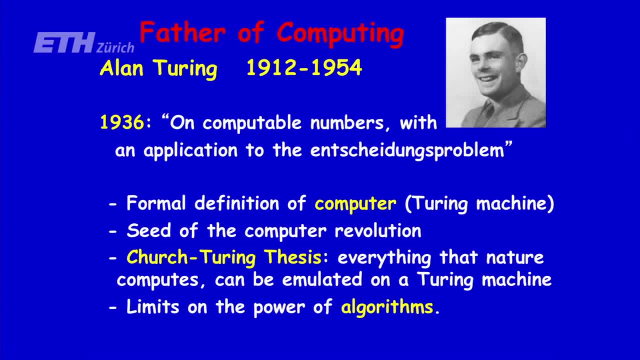 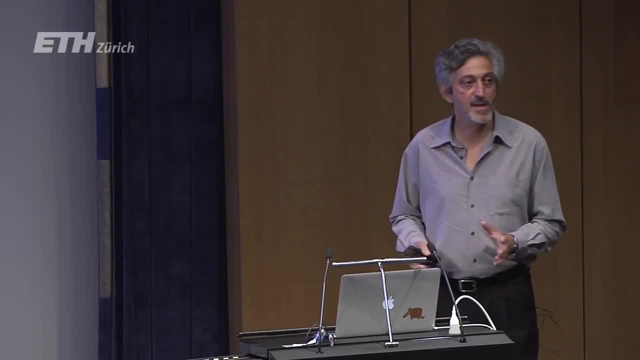 particular paper, Turing gave the formal definition of what a computer should be. Computers didn't exist then. This is another thing that's very important- to stress the importance of theory to practice. Practice didn't exist before the theory was ready for it to develop and 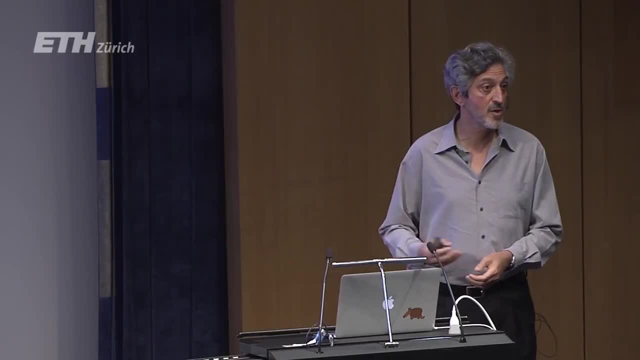 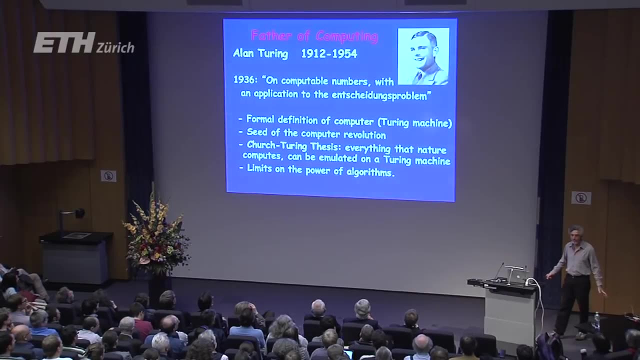 actually set, prescribed how it should develop. Alan Turing went on to build computers- some of the first computers- and this paper was, in particular, the seed of the computer revolution that we all feel today. That's why it's considered the father of computing. But that's not everything. 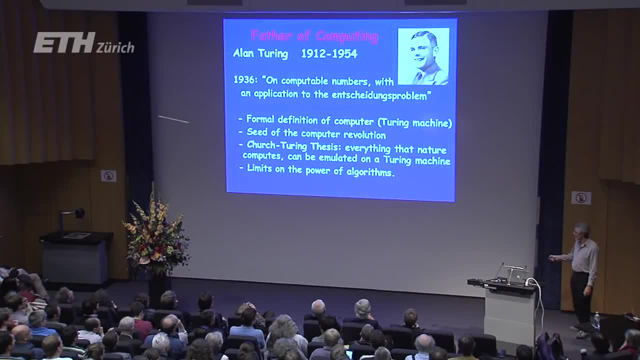 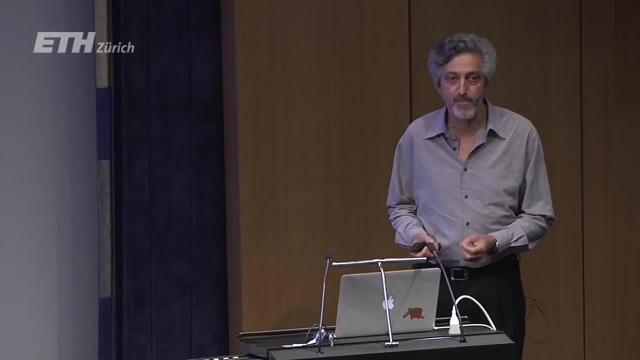 there He already saw in the beginning what came to be known as the Church-Turing thesis, which actually says that his model, which is a very, very primitive model, which is a type of computer, is universal, should be able to emulate any computation that happens. 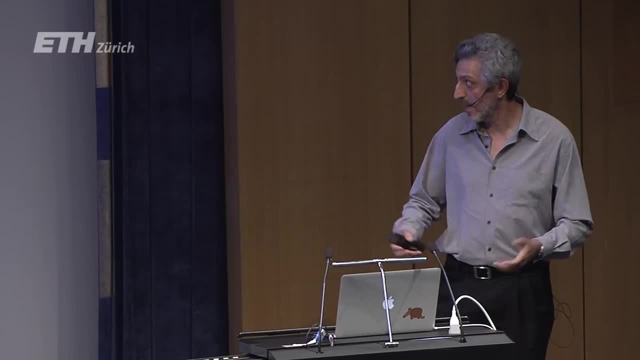 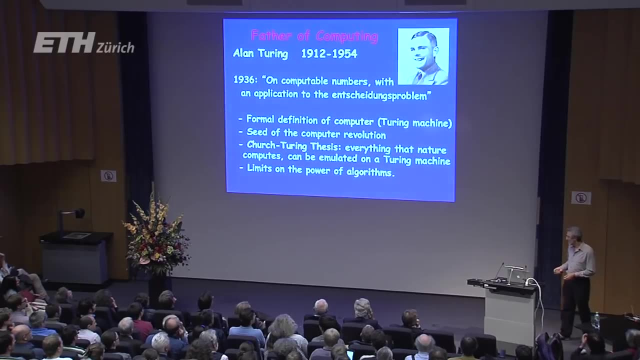 naturally, in particular in nature. That was a claim about his machine. Finally, last but not least, he already proved that computers cannot do everything, Despite. I don't expect that this will be true, but I do believe that it will be true. We're going. 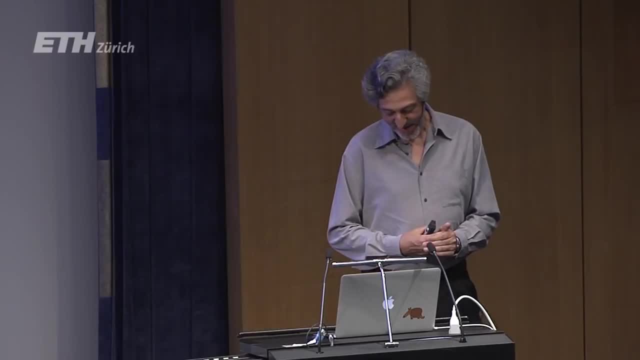 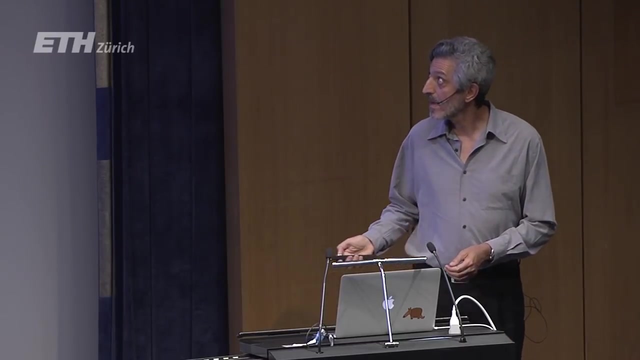 audience is naive, but generally people still feel that computers can do everything. Even before computers existed, we knew that there is a limit to their power. There are certain problems that they cannot solve, and we'll talk about that. So first, what is an algorithm? Well, you know, at this day and age, everybody knows. 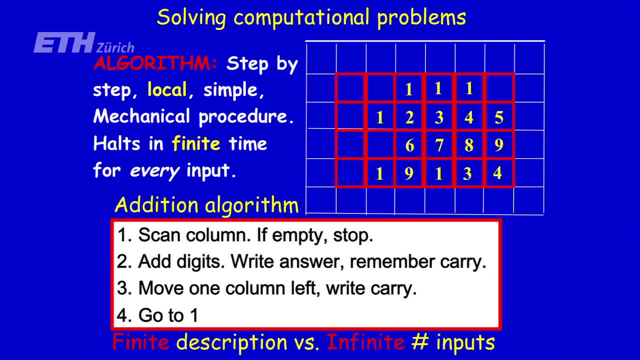 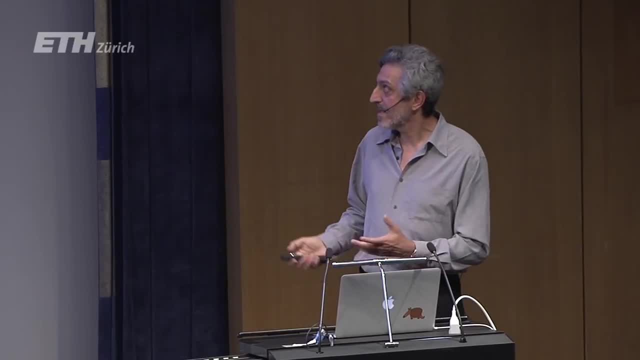 what algorithms are. They are basically computer programs or the ideas for computer programs. I will always use this kind of white background to describe an algorithm, which means you don't have to read what's inside, But in this particular example, this is something we learn. 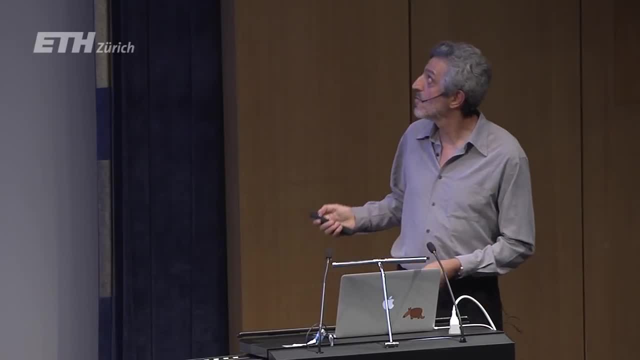 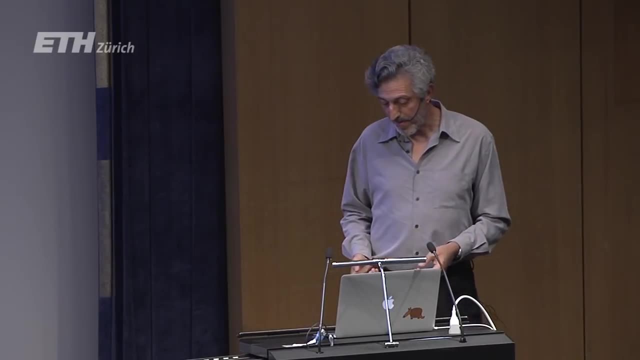 We learn an algorithm. everybody learns an algorithm in second grade- how to add numbers. how to add numbers- And that's a fantastic way to think about how a single algorithm can be used to solve a problem. A sequence of simple and local operations can actually evolve things that are very complex. 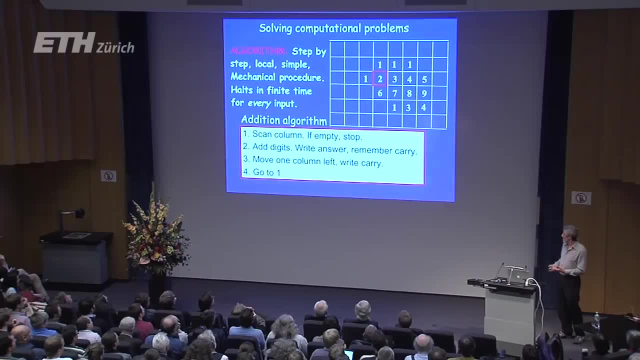 very long, arbitrarily long. It's just a sequence that at every step, your view, your focus is on a single cell and what you remember is another single digit, more or less. So it's very simple to describe, and actually simple to implement, a program which is finite. 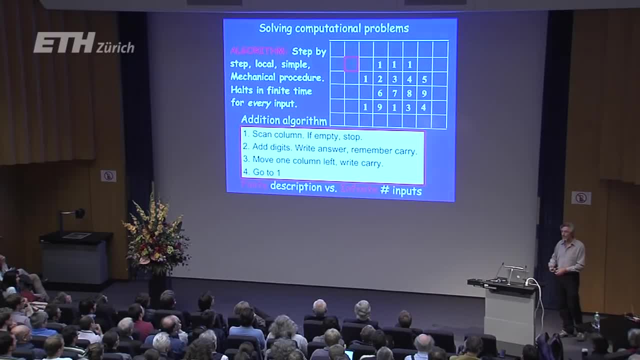 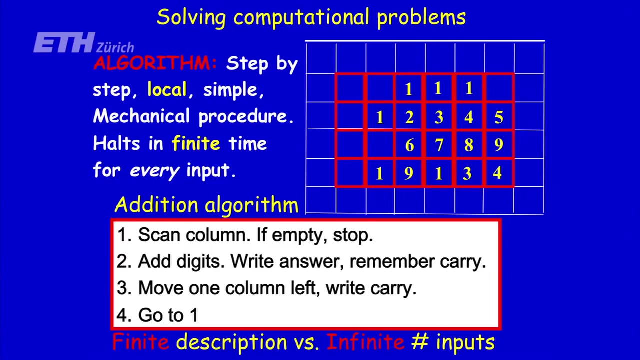 it takes a few lines of code to write, but actually can handle inputs of any length, arbitrarily long inputs, so, in particular, an infinite number of inputs can be handled by this very finite small blurb of white, this piece of software. So this contrast is: 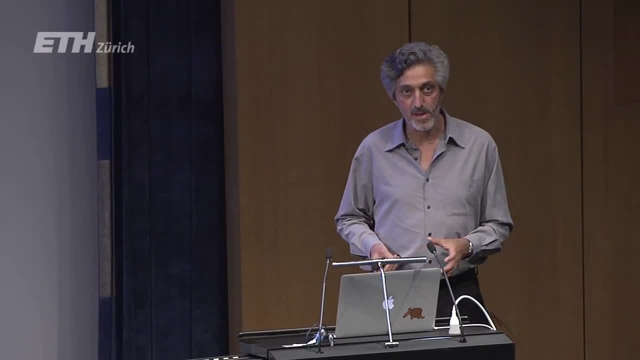 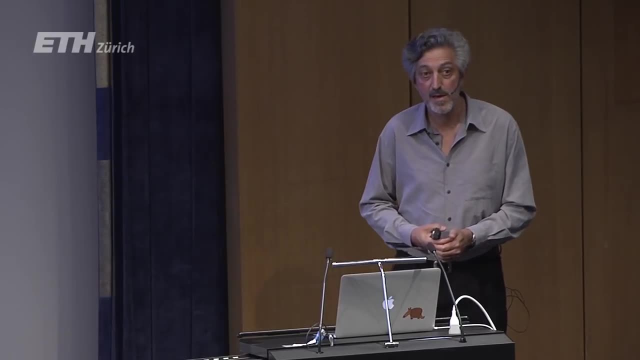 extremely important. It's very important to use this kind of algorithm, and this is what: remember that an algorithm is something small, finite, that can handle, can solve arbitrarily many, infinitely many instances of a problem, In this case, all the problems of adding two numbers, whatever they are, And that's what you want: an 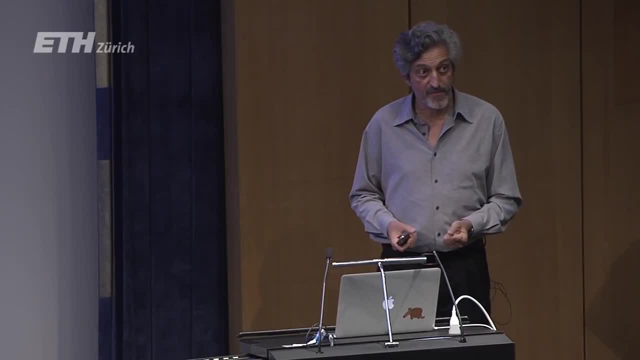 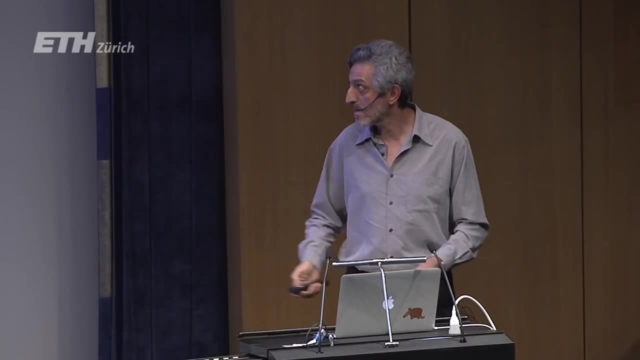 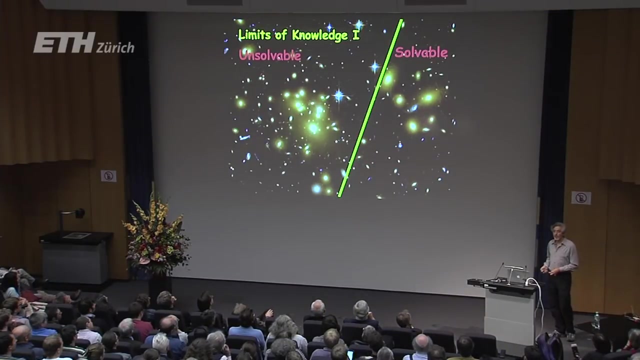 algorithm to be. And the other property of an algorithm is to redefine. it has to halt, So it has to provide the correct answer, and stop so that you know when the answer is ready. So that's an algorithm. Once we have a definition of an, 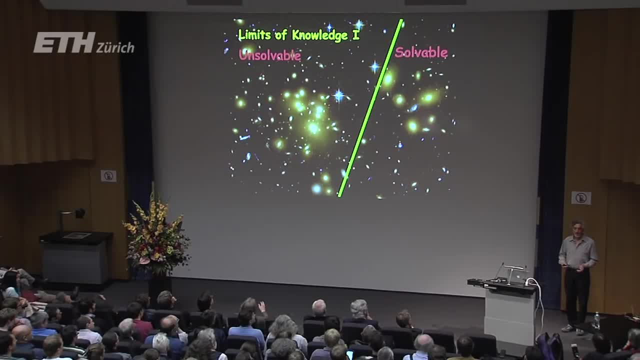 algorithm. we can ask ourselves: what can algorithms do? It's a formal definition. I didn't give you the formal definition, but it's there in the paper and it's a mathematical definition. Then you can say: well, okay, I have all the problems in. 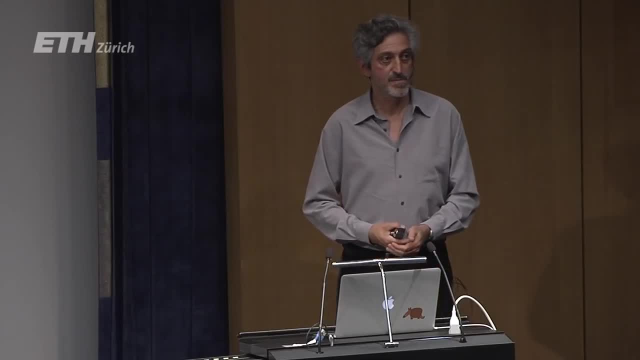 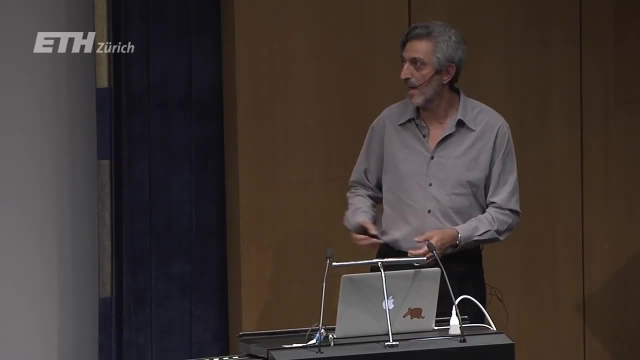 the world. I have all the algorithms in the world. what you know? can every problem be solved by an algorithm? In fact, there were particularly interesting problems that caused this line of research that Turing was part of, initiated by Hilbert, who thought that yes. 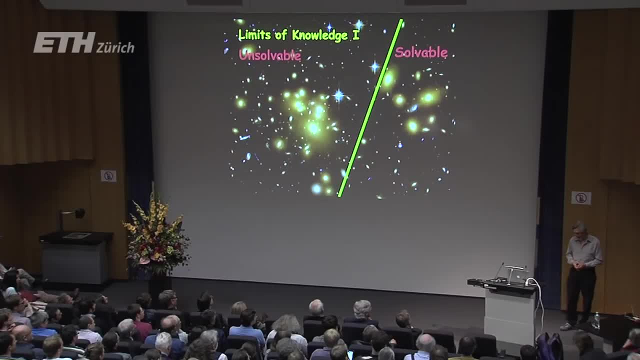 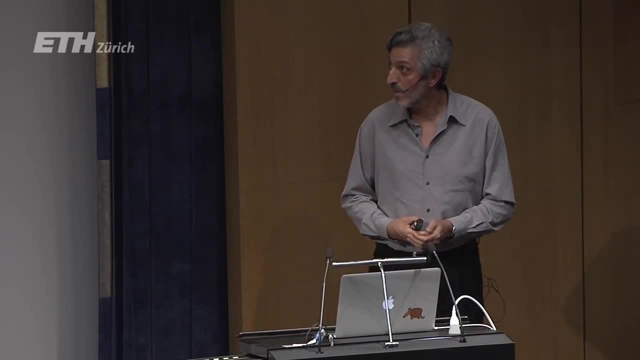 every problem, at least mathematical problem, can be solved by a finite mechanical process like an algorithm. Only he didn't have a definition. Once you have a definition, you can start arguing, formally arguing- about it. And not only was it possible, but it was also possible, And so you know there are a lot of 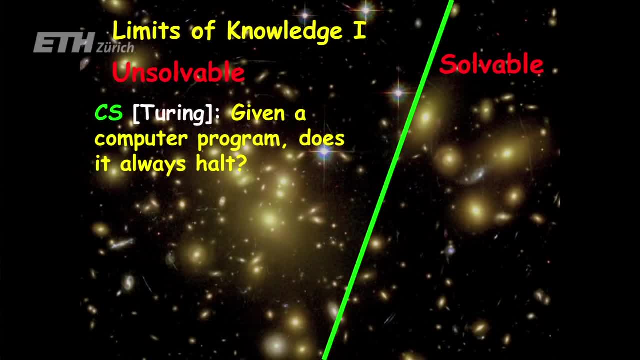 problems Turing in his first paper did exactly that. So he proved that certain problems, in this case maybe the most fundamental problem of computer science today, testing whether your program has a bug or not, whether it you know it will. 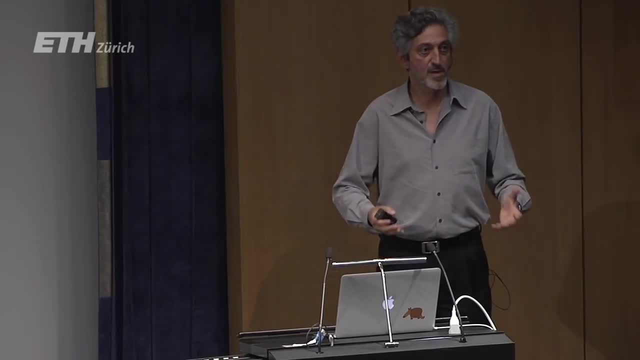 run forever or not. This problem, where the input is a computer program and the question is, does it ever go into an infinite loop, is unsolvable by algorithms. So it was always a problem, And so you know, Turing, in his first paper, did exactly. 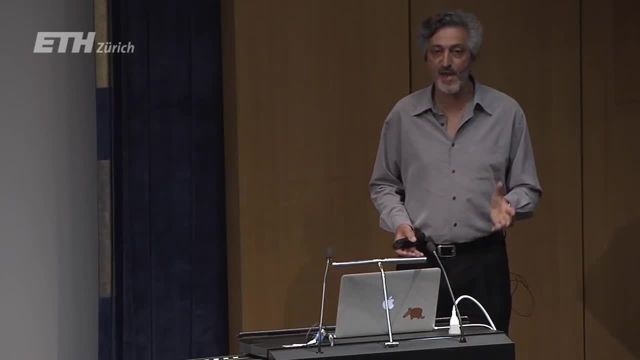 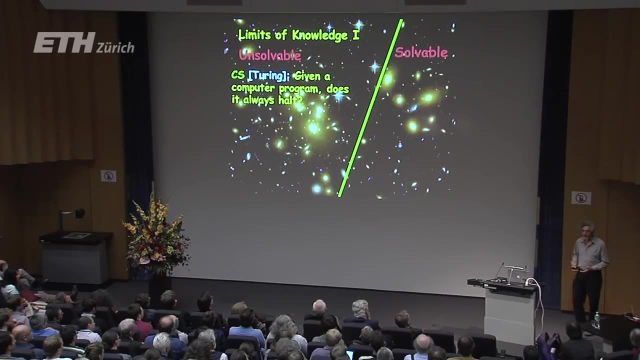 that, But probably already when computer science was born we knew that the most basic problem in computer science cannot be solved by computers. But then it took off and people started to look at other problems in other disciplines and seeing whether they are solvable. 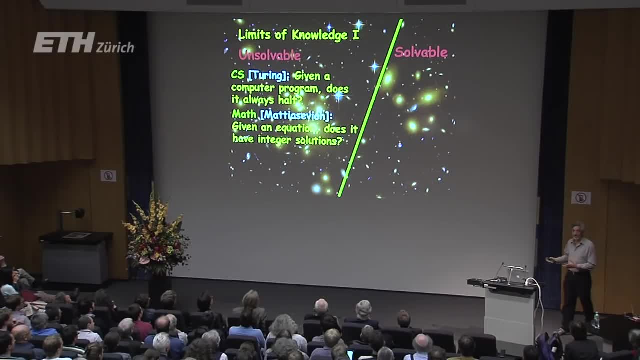 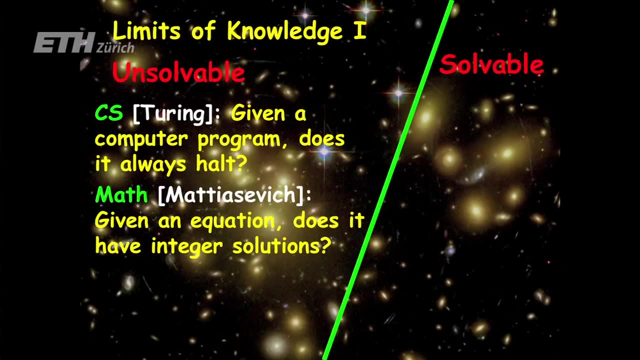 by algorithms, And one of the great successes answering Hilbert's question was the result of vac他是 lon ما, The�� par dep ther yow fiz ajna kyei he salchow Bird. CAO TOO Sandy Matはいg iz tesna Ses��� 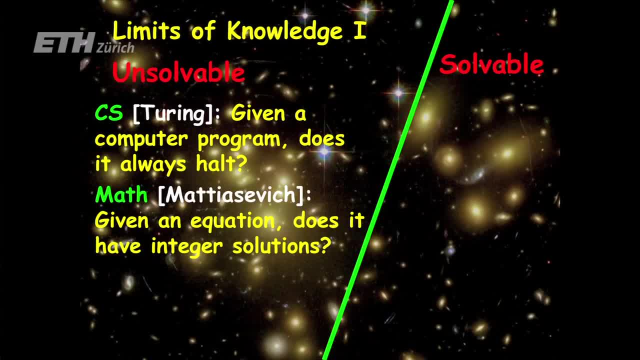 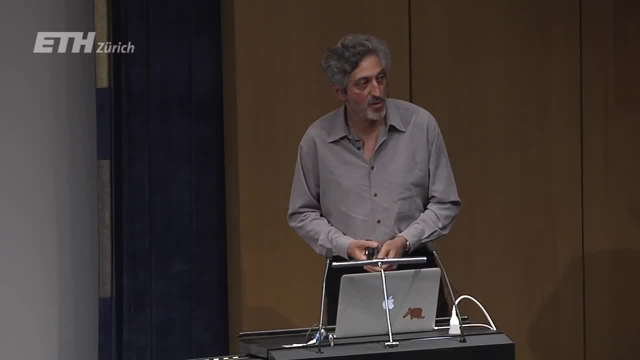 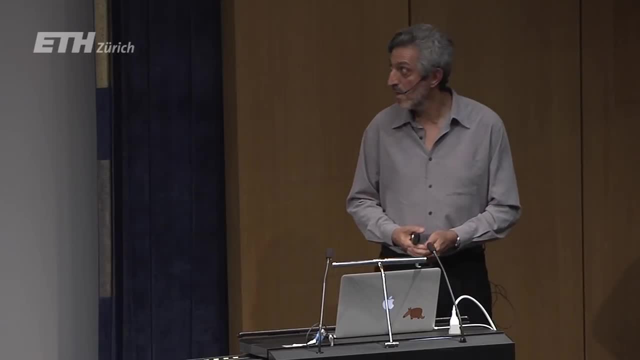 following Partnam, Dav, результатStar Martin and Robinson was that here's another problem that cannot be solved by a computer. I give you an equation, an integer polynomial, and the question is whether it has integer roots, integer solutions. This problem- again Silbert's intuition- is not solvable by algorithms. 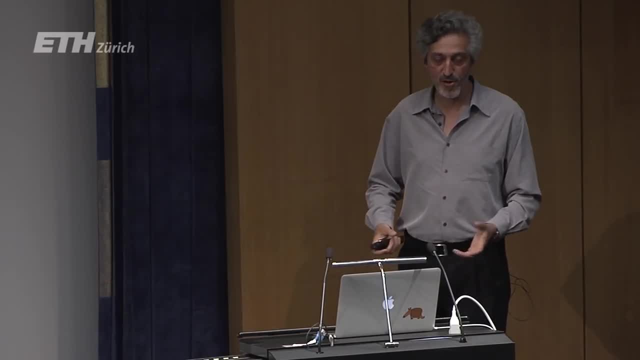 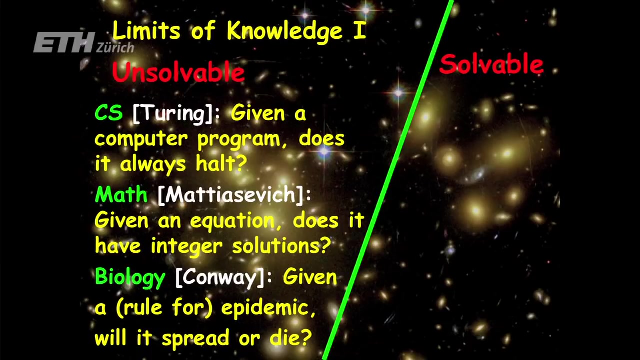 So another very basic. I mean mathematicians study equations. that's perhaps the most basic objects and in general you cannot hope that a mechanical device will tell you whether there are solutions or not. Same in biology We talked about questions like I give you. 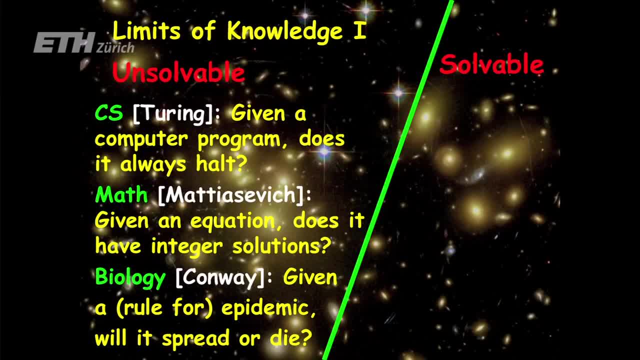 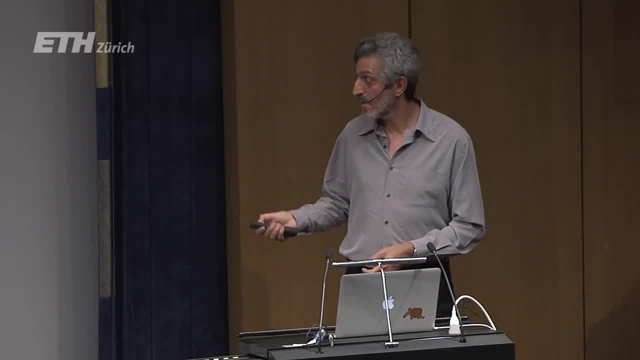 I understand some biological system, some epidemic, let's say, and I ask: will it spread and take over the universe or will it die out? These kind of questions, as shown by Conway in The Game of Life, cannot be solved by computers. 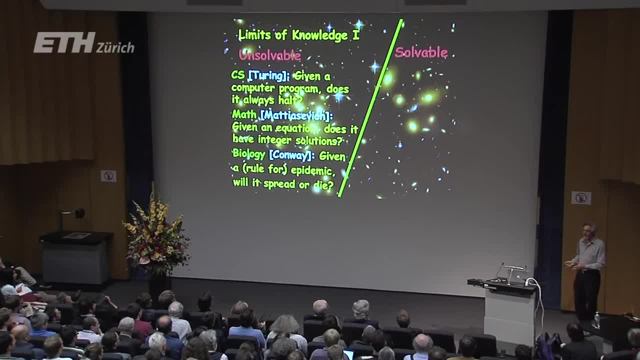 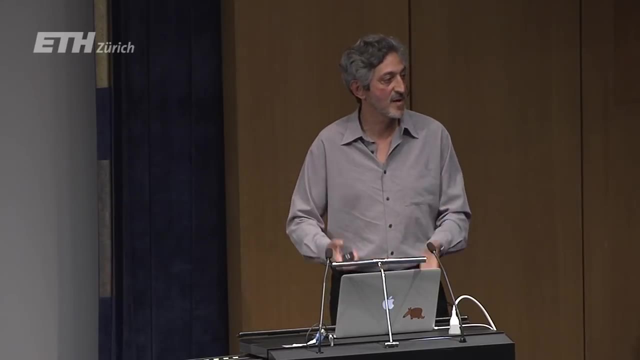 So already we see that in this night sky of problems there's a huge, in fact really huge- collection of problems that just cannot be solved by computers. So that's great. but of course we are interested in the other side. We have computers, they are doing some things. 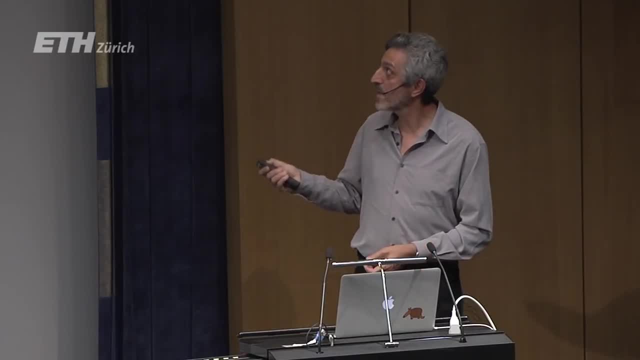 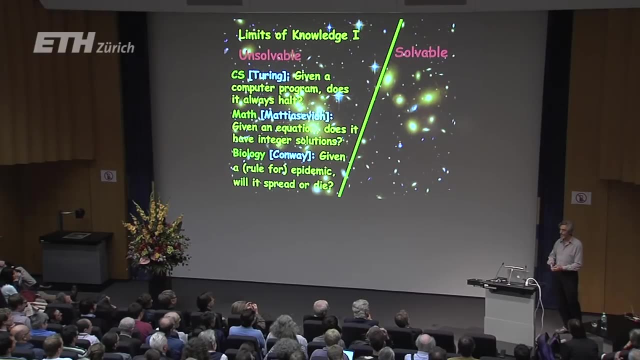 So what are the solvable problems? There are everything on this side, But once people started dividing algorithms that actually work, that always stop and provide the correct answer, they realize that just having a solvable problem is not enough. And it's not enough because 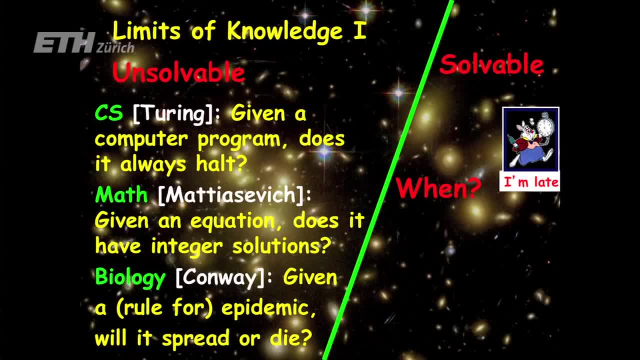 we want to have the answer quickly, Having an algorithm that stops in finite time. finite can be a very long time. you want it to finish quickly, And so that was the birth of computational complexity theory. So computational complexity theory studies how much time. 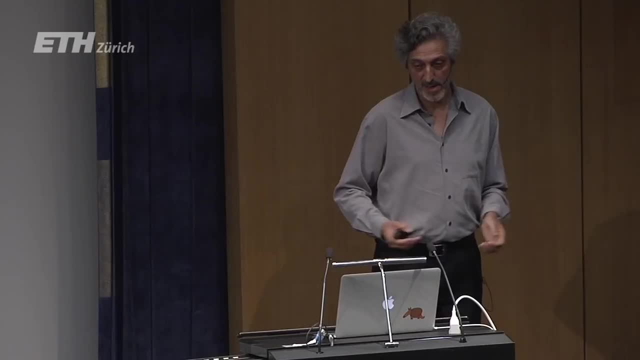 or, more generally, how much resources should go into a computer program that solves a particular problem. Now the definition of exactly what it means is a little. you know. it's more complex than just whether an algorithm exists. So I want to explain it now. 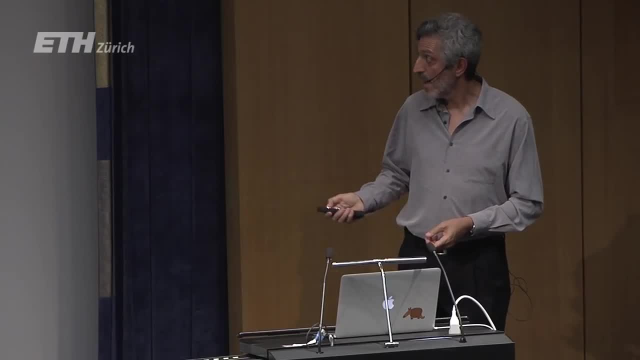 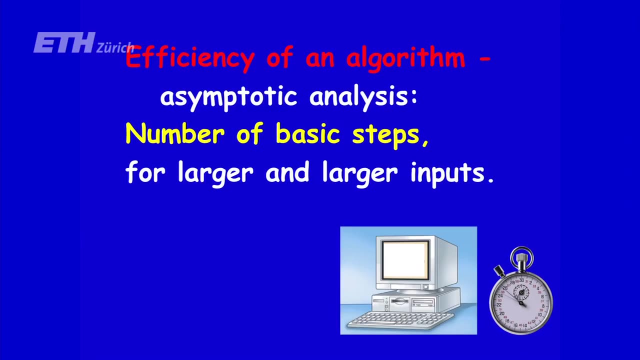 And that's a very important definition. How do you define the complexity of a problem So it's solvable? How do you define how difficult it is? The way you look at it is as follows: You expect- at least if you did any arithmetic in school- 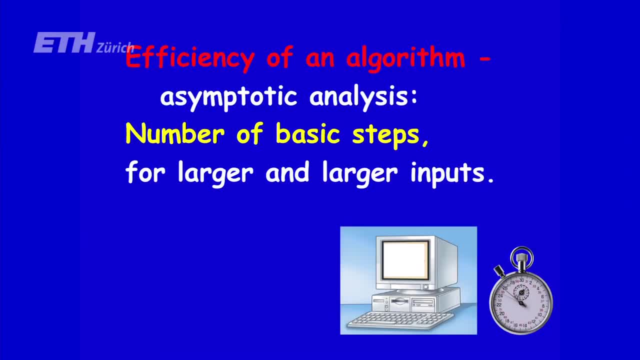 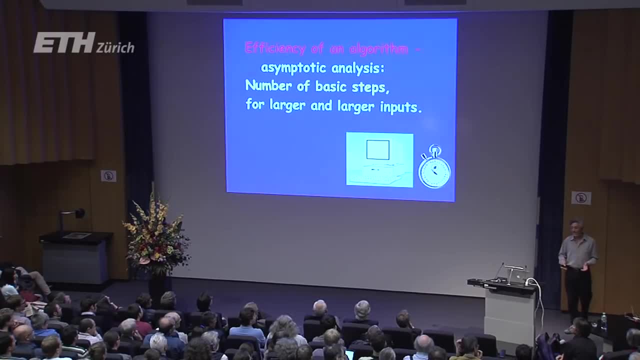 and I'm sure you all did and maybe some of you are still doing it. you know that the more data you have, you expect it, you know, to take longer to compute, even if it's the same problem, even if it's an addition problem. 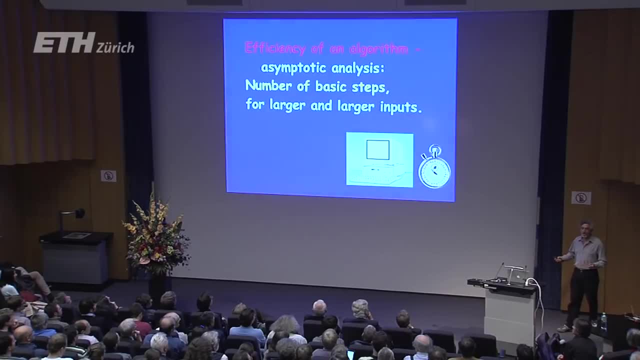 So what you are trying to understand is, as the data to the problem grows, the instance you feed it grows. how much more time should you invest? What is the relationship Between the length of the input and the time it takes? So, and you expect that you know- 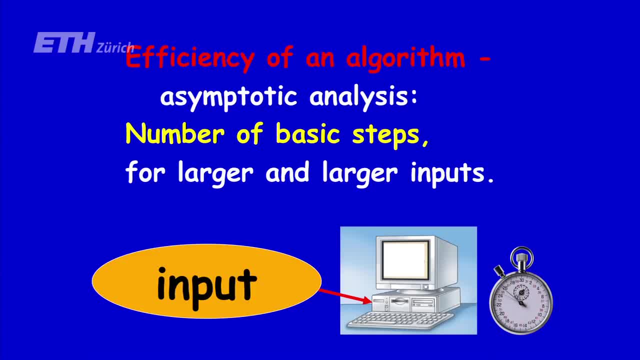 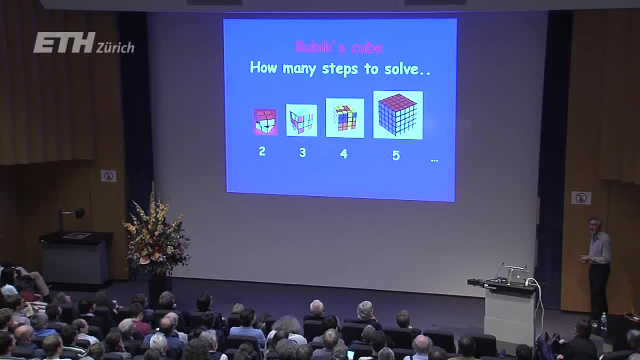 bigger and bigger inputs will take longer and longer time. but the question is, what is the relationship between these, the two growths? So if we were talking about solving Rubik's Cube, then there are the number of, let's say, the maximum number of steps. 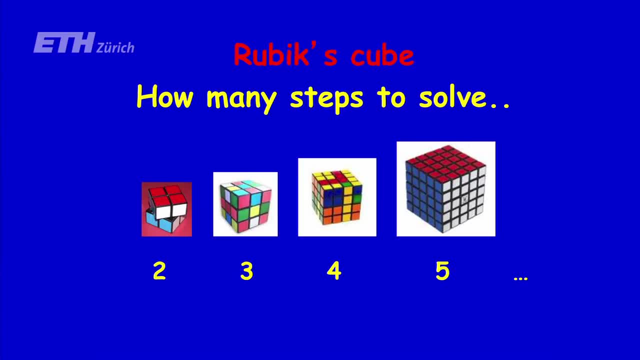 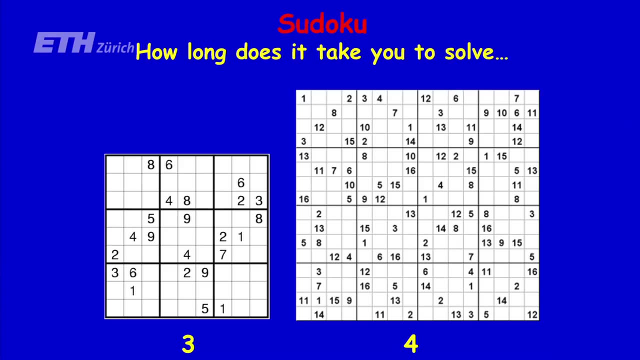 it will take to solve two by two, and then for three by three and four by four, and of course, these grow and the question is: how do they grow? Or if you are, if you like, Sudoku, you know you can think of your method. 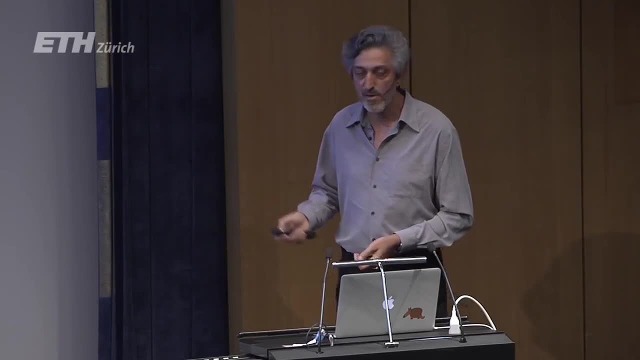 for solving Sudoku puzzles. How long does it take on this three by three type of problems? And then maybe you can try it against the four by four and five by five. So it's an asymptotic approach into understanding the complexity of problems. 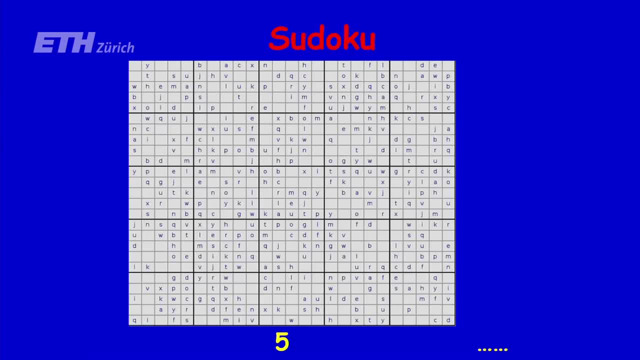 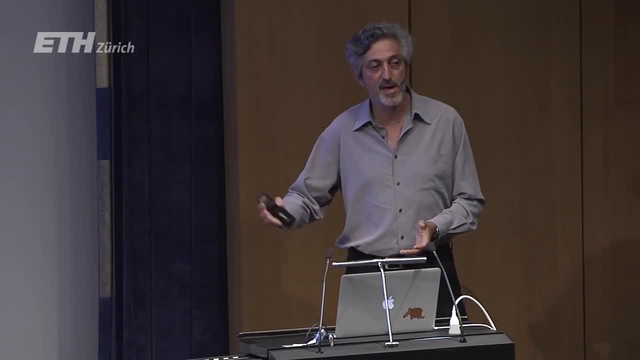 Okay, I hope this is clear. So what we are really trying to understand is not how much it takes to solve, for example, Sudoku on three by three examples. We really want to understand: as the size of the problems increase, how much more time do we need to invest? 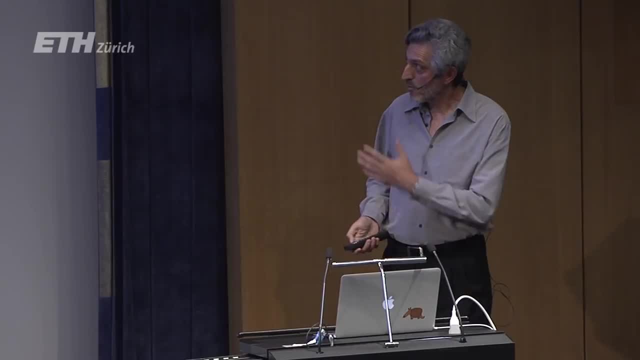 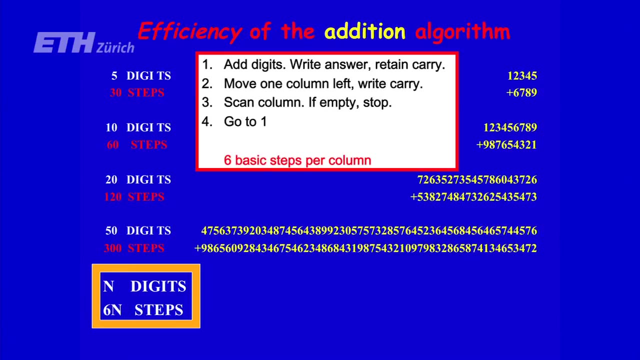 in order to understand it. So I'm not going to analyze these examples because, in particular, we don't know, but I'll give you a few examples that you do know, and just to get some set of terminology. So, for addition, you know. 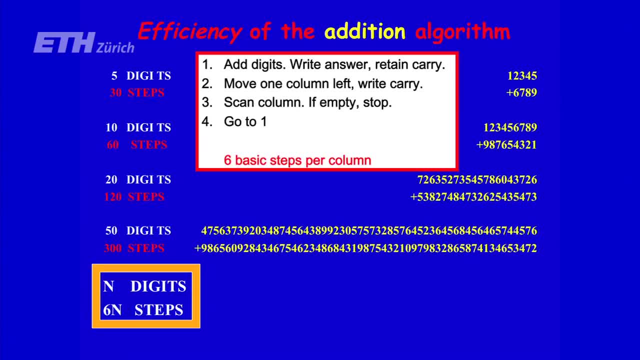 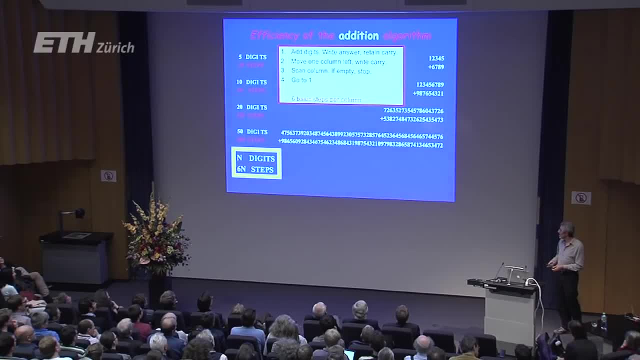 the algorithm before. it basically sort of makes you know three steps down, three steps up in every digit that proceeds, or maybe six basic steps per digit. So if you know we are working on five digit things, then it will take 30 steps. 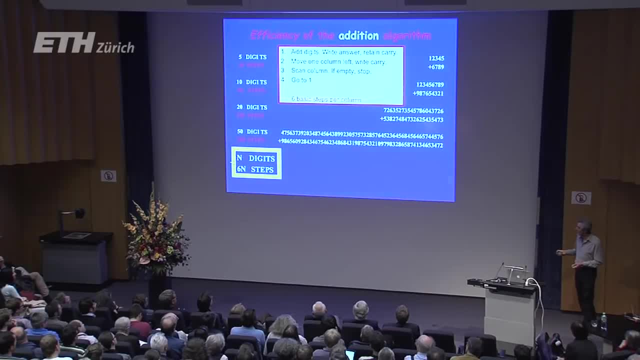 and 10 digits will take 60. And in general if we have n digits it will take about six n steps in this particular algorithm. So what are the questions we are asking about this algorithm and about algorithms in general? Let's say we found one. 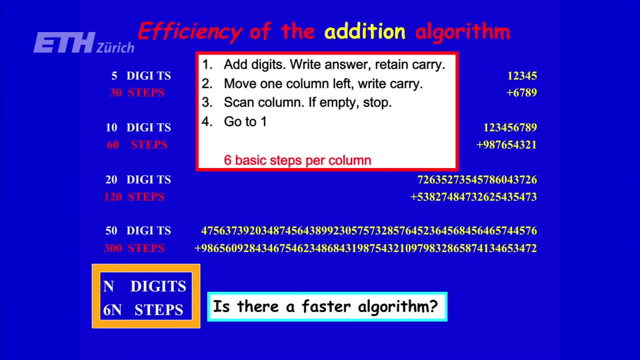 The most important question to ask is: can I do better? This is maybe because you don't have enough time and you are trying to finish homework fast. This is maybe because you have a startup and you want to beat your competitor. There are many reasons, but that's the most basic question. 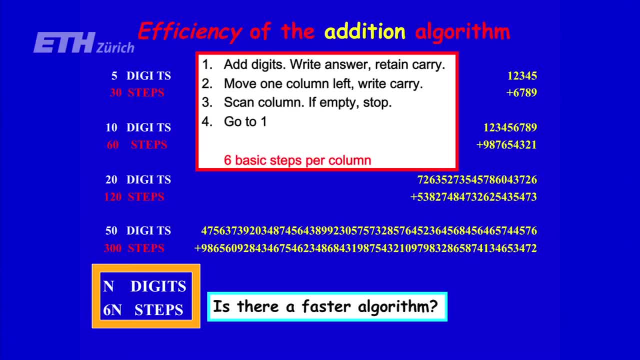 Am I paying the minimal amount of resources in order to solve a problem? And in the case of addition, the answer is obvious. It's basically no. The reason it's: no forget the six. The six doesn't really matter. What this algorithm is doing is saying the following: 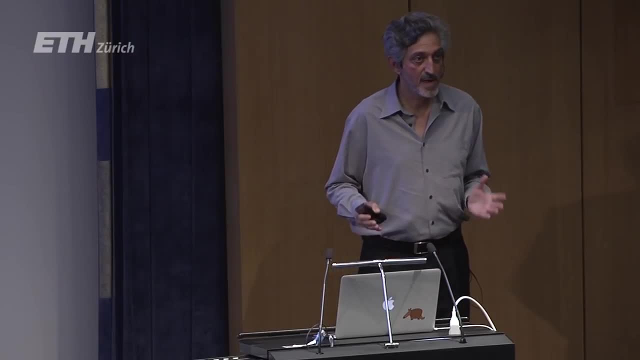 The amount of time you invest on solving addition problems is proportional to the size of the data. Now you have to read the data at least in order to solve the problem. So it's as good as it gets. Maybe the constant will change, but there is no better. 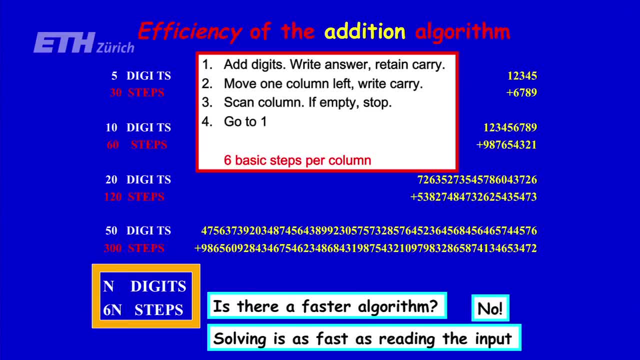 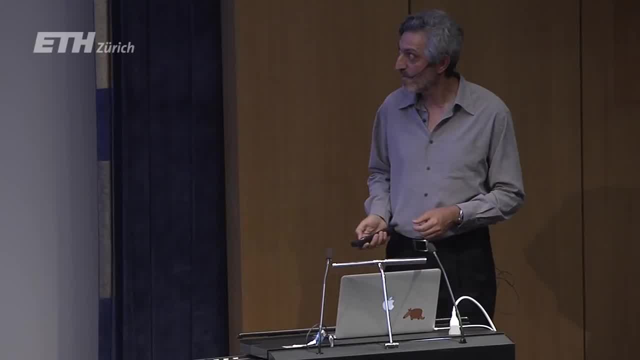 You solve the algorithm. You solve it as fast as you can expect. This is a miracle. The addition problem is a miracle. We don't have too many problems like this. We don't know too many problems like this. Let's look at the. you know that was second grade. 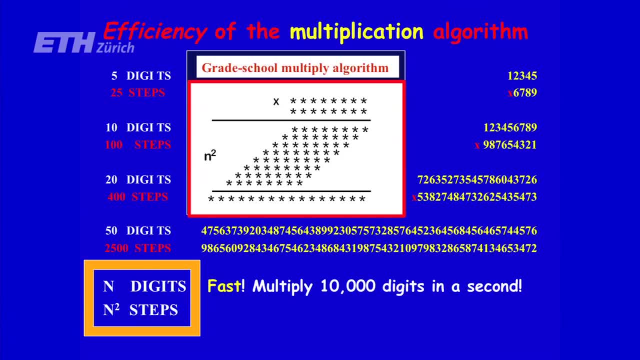 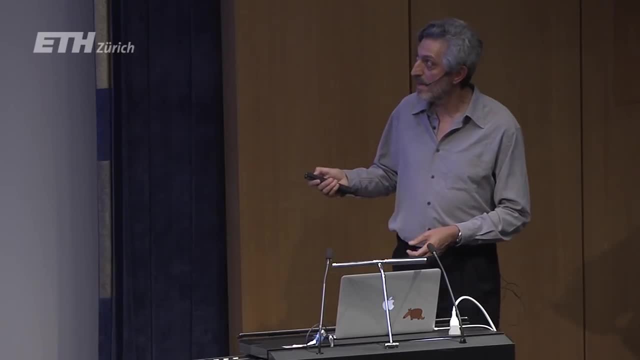 Let's move to third grade. In third grade we learned how to multiply long numbers and I'm not writing down the algorithm, but you remember that it has this form. and this form means that if you have n digits of data in your problem, then roughly the number of steps. 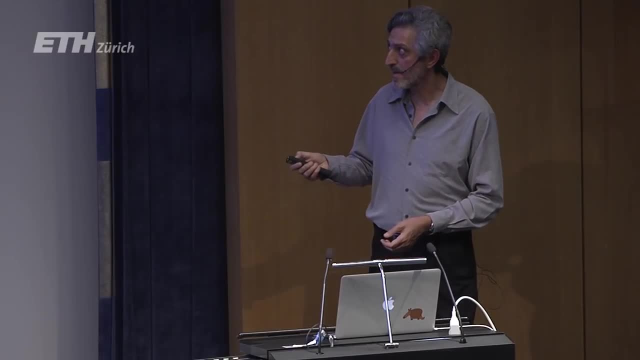 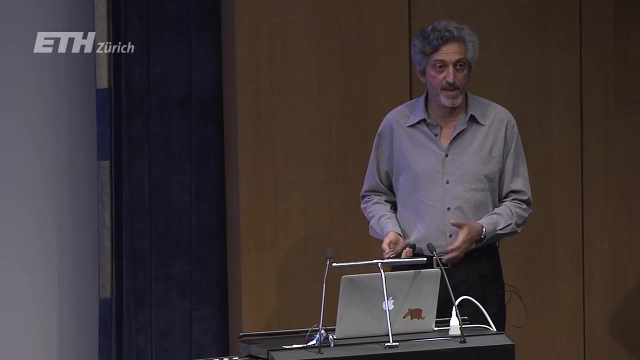 even the space to write down grows something like n squared quadratic in the number of digits. Now, this is still you know. so the relation is n digits of data, n squared steps in this algorithm. So it's still fast in the sense that you can multiply. 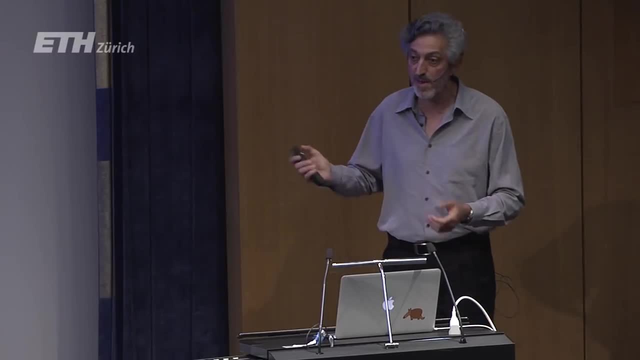 huge numbers like 10,000 digits in a second, or probably less. So it's quite fast. Of course not as fast as before, and again we should ask ourselves the same question as before: Is there a faster algorithm? 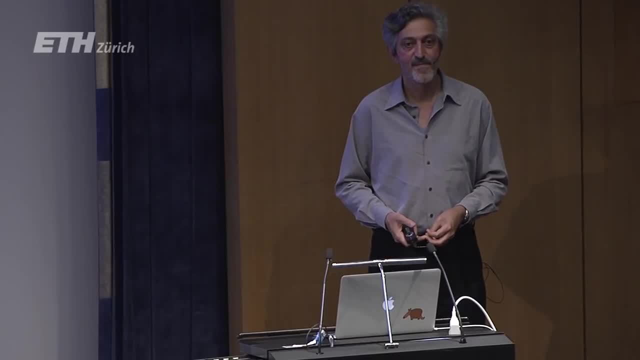 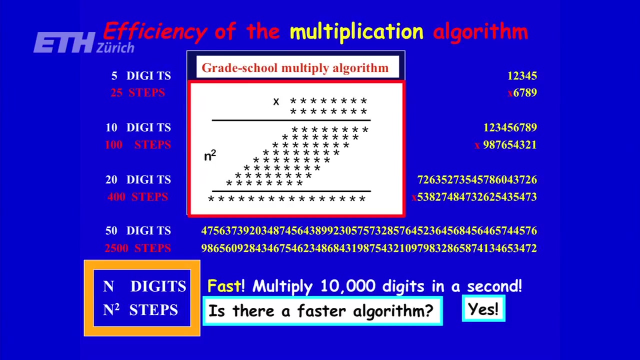 What do you think? Who thinks yes, All right. Who knows a better algorithm? Same people. There is a faster algorithm. Don't teach it in third grade. It's far more complex, But you should know that the best algorithm we know. 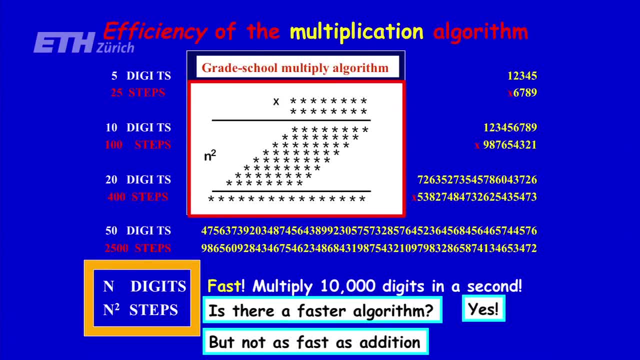 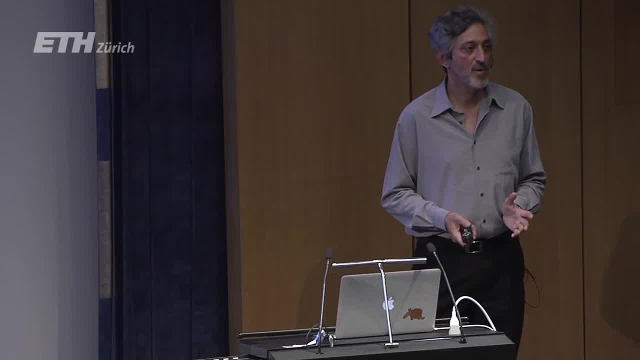 for multiplying numbers is not as fast as the algorithm we know for adding numbers. So the basic question is: multiplication harder than addition? We don't know how to answer today, even though 50 years of research went to in particular trying to prove it. 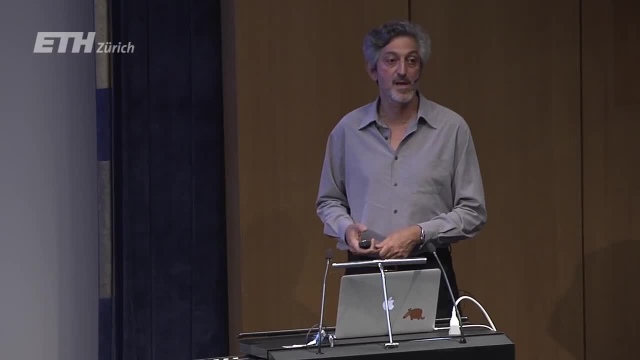 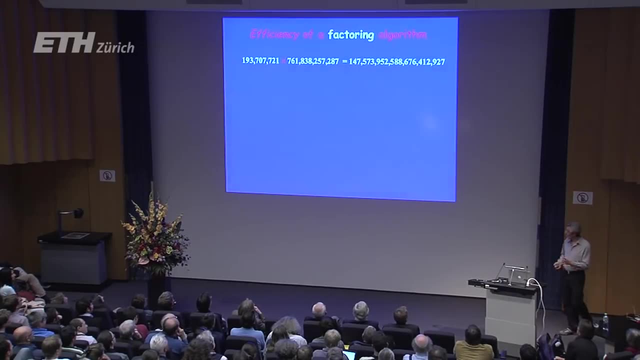 Either way: either get a linear time algorithm or to prove that there is no linear time algorithm, So we don't know. Here's another problem which is actually very important. So remember multiplication. Multiplication is getting these two numbers and producing the product. 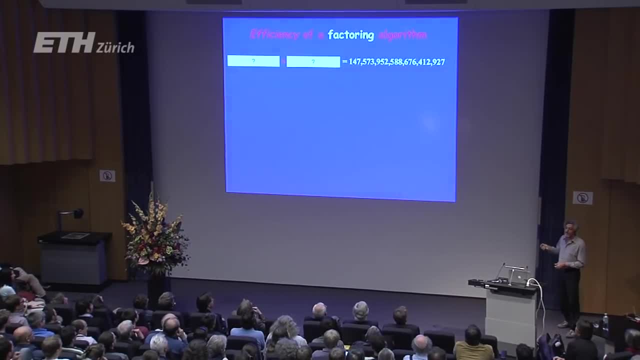 Let's look at the inverse of this problem. I give you the product and I ask you to find out the factors, The two numbers whose product will give you the outcome. This is the factoring, the integer factoring problem. What's the best algorithm? 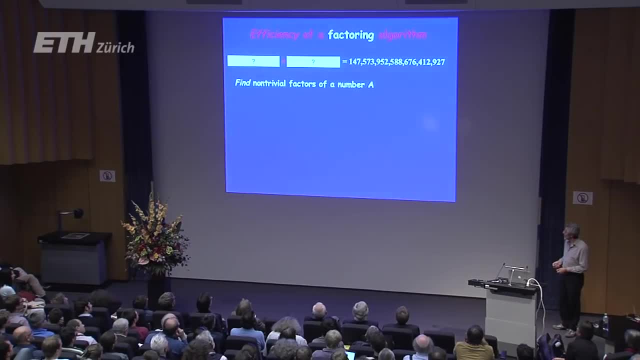 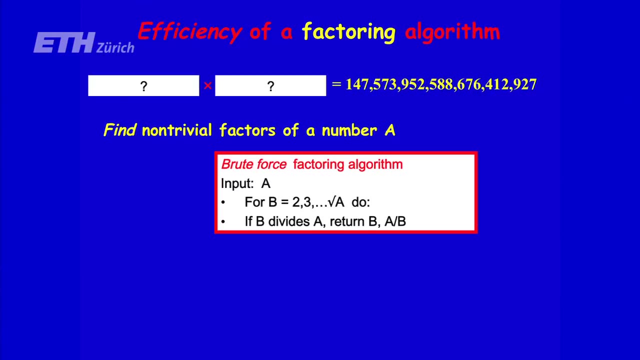 For this? Well, there is definitely a stupid algorithm, which is sort of a brute force algorithm, which says: well, OK, let me try all possible divisors. Let me try, if the input is a, let me try to see if 2 divides a, if 3 divides a, 4 divides a- 5. 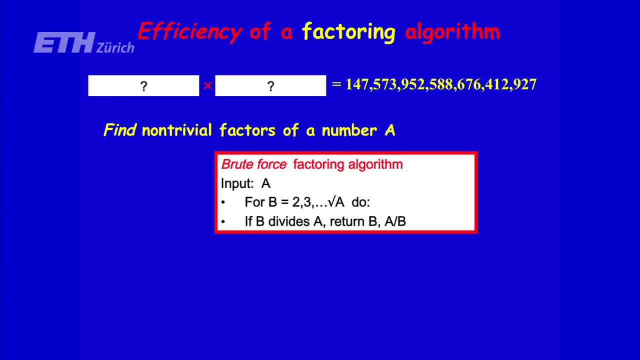 divides a and so on. I have to go probably all of them, but I can stop at square root of a, Because if there's some divisor, a non-trivial one, then there's one below square root a And I try them. 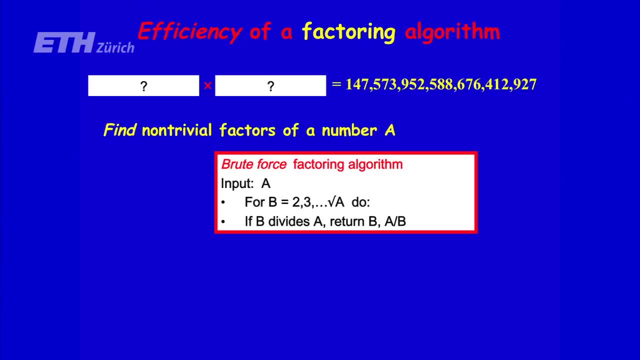 If I find one. good, Because for each of them I can try. division is an efficient procedure, not just multiplication. How good is this algorithm? It's really terrible. It's really terrible- I mean this algorithm- if the input is n digits. 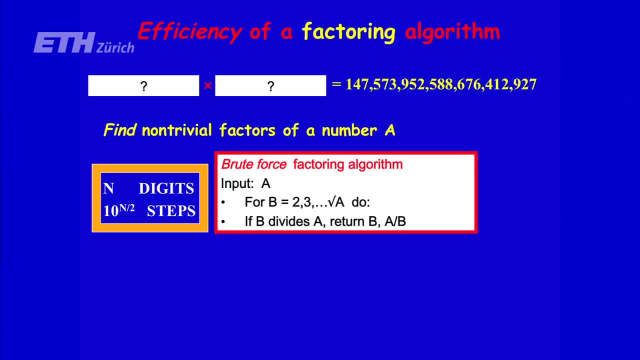 the runtime is roughly 10 to the n. Well, it's not 10 to the n because it's a square root, so it's 10 to the n over 2.. But it's exponential. It's exponential in the amount of data you have. 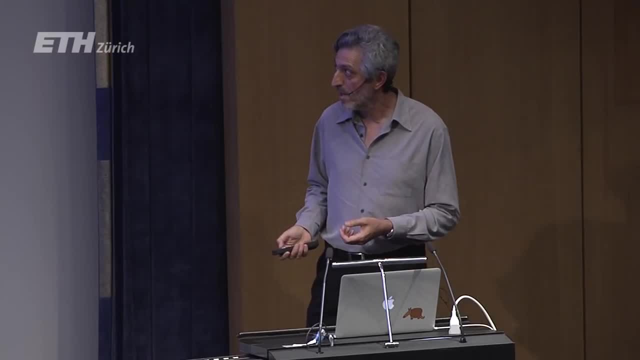 So, in contrast to multiplication here, if you have even 1,000 digits and you want to factor them this way, 500 billion years of the energy of the sun would not be enough. So this exponential time is terrible. It's something completely. 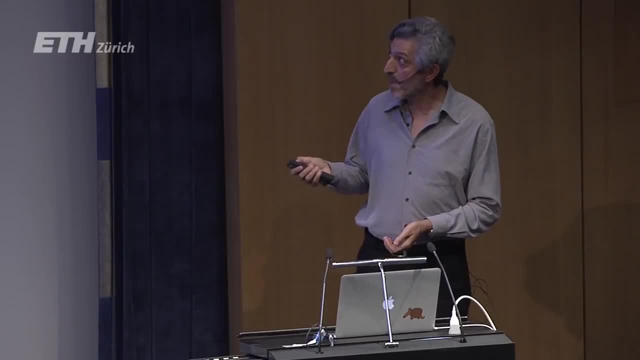 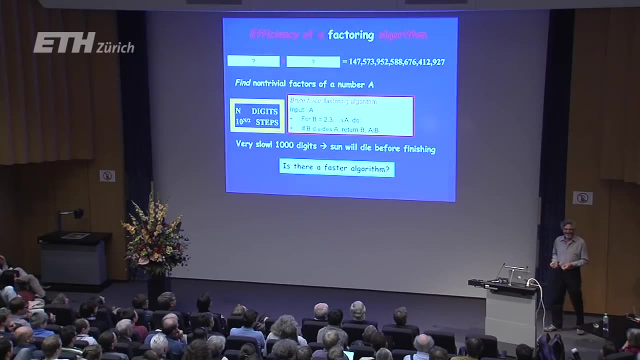 It's completely impractical, something we cannot live with. So if this was the best algorithm, we can ask ourselves the same question: Is there a better algorithm? Yeah, The answer is yes, but it's still exponential, So we don't know. 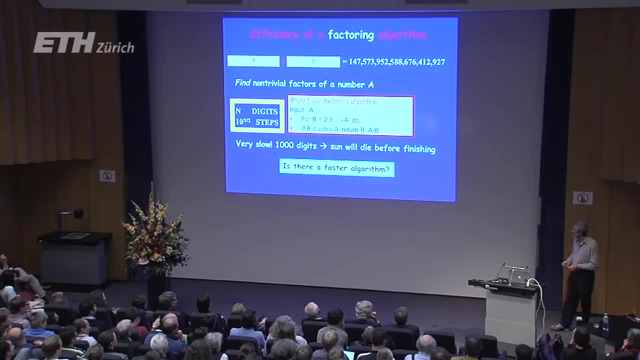 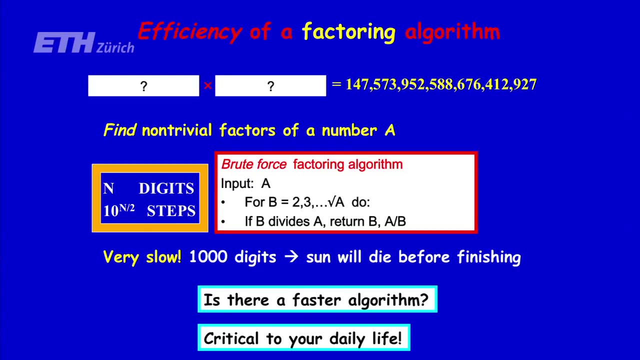 I mean, it's significantly better than this, but still terrible. So, as it turns out here, we also don't know the answer. But this problem is important, because this, this is not an easy problem. The difficulty of this particular problem affects your daily life. 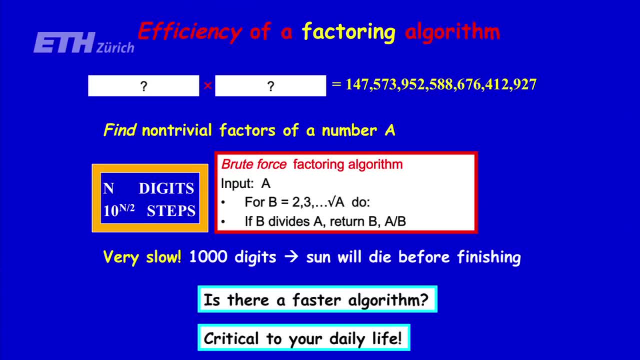 Some of you know it and some of you don't. I'll mention later why. But the complexity of problems, even if they seem abstract and number-theoretic, and you know you shouldn't care if you are doing something else. 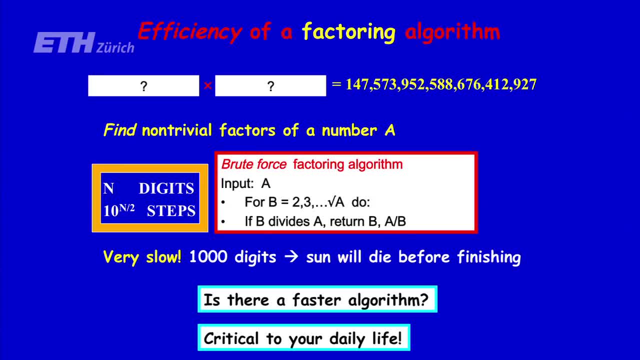 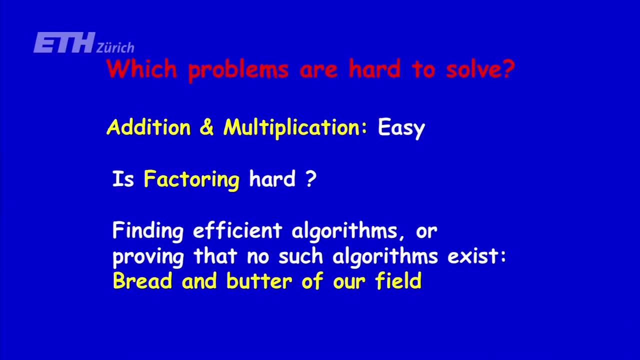 well, you should care about this one. It's really important And we'll see. OK, So we understand. we saw some examples of the complexity of what we know about, the complexity of some problems. So we have a language to talk about. 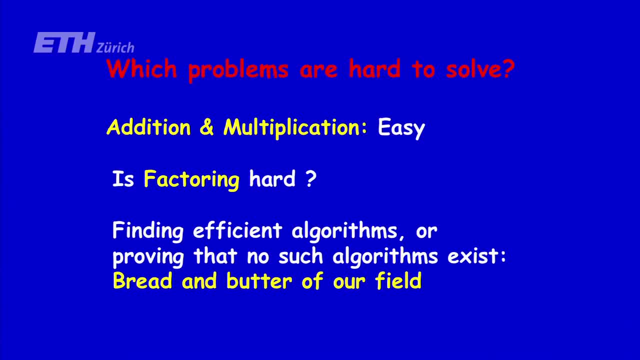 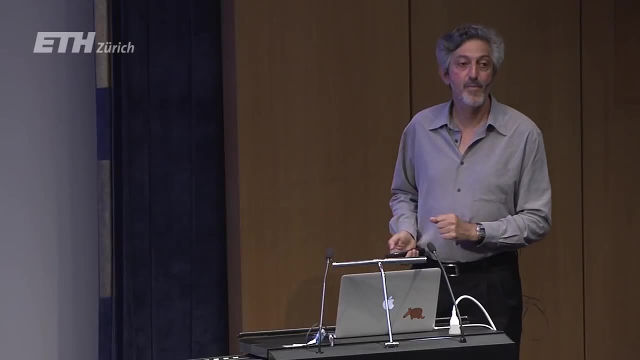 And now it's a- yeah, it's a good time in the middle of the talk to I'm taking an hour from after all, the introductions Talk about basically propaganda for the field. So efficient algorithms are really important, You know. 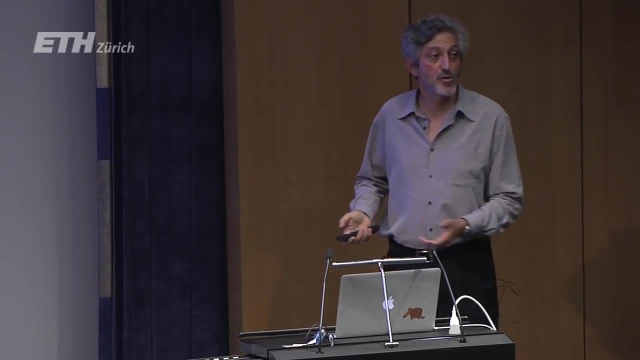 We saw that these two problems are easy about factoring: we don't know. It seems difficult but we don't know. And the question of finding algorithms, efficient algorithms, is absolutely fundamental to computer science And not only computer science, technology in general. 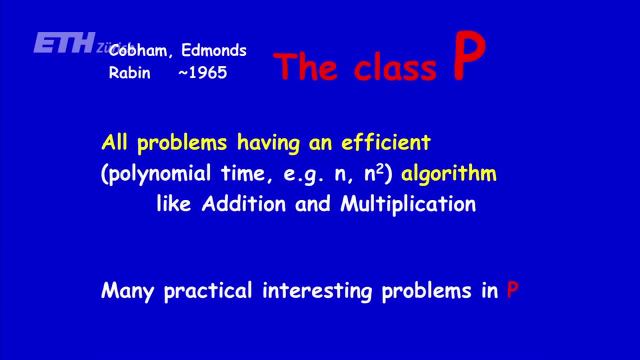 So let me just do this propaganda in. OK, let me just define first. We saw I want to collect the the problems that we called easy, like additions and addition and multiplication in a class, So all the problems that we can solve efficiently. 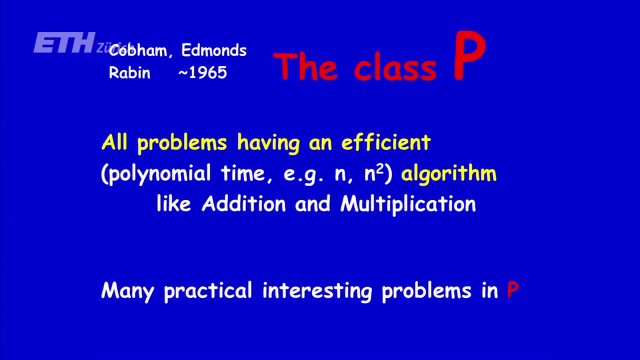 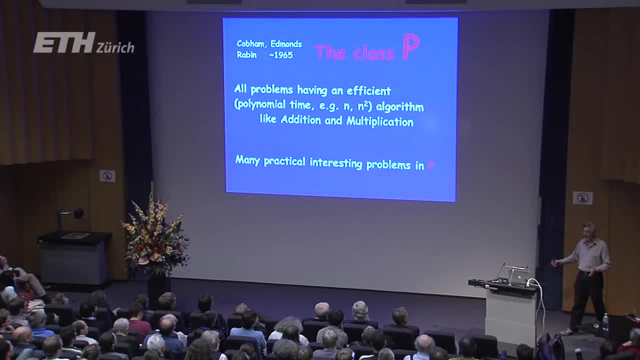 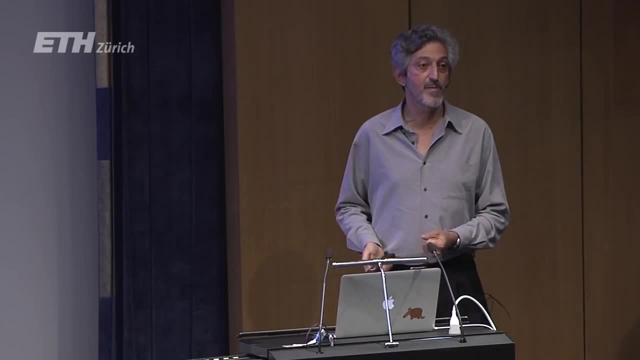 And for us efficiently, will be in for with algorithms that run in time, which is polynomial in the size of the data, So n m squared, m cubed, but not exponential. And these problems are problems in P, And I'll just give a few examples of some problems. 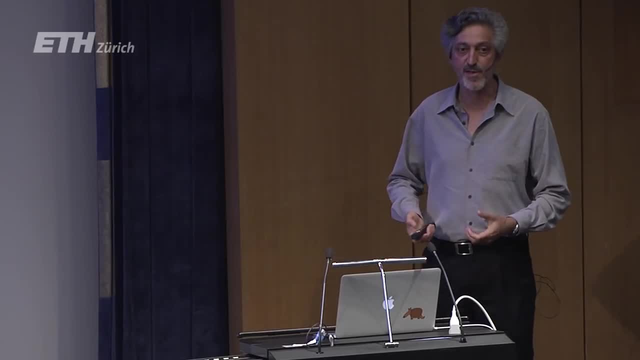 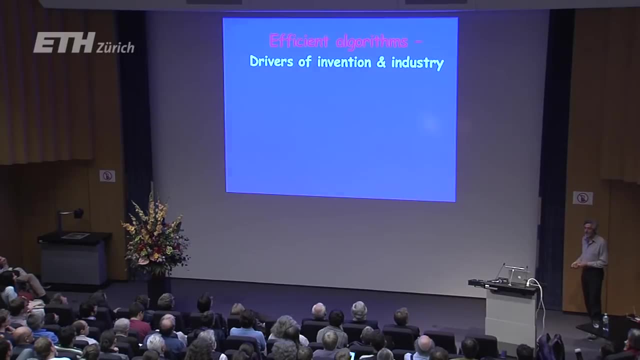 in P. that really you know. you notice that they are in P in the sense, you notice that they have efficient algorithms And yeah, OK, And the way to do it is. let me ask another question: How many people heard on, heard about these guys? 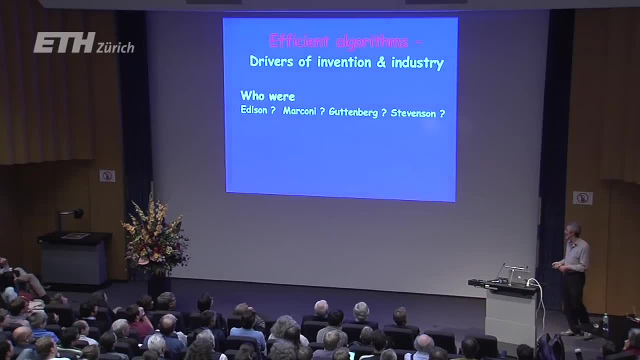 Yeah, OK, I shouldn't have asked who never heard? yeah, of course everybody. But how many people heard about these guys, The computer scientists? very good, Yeah, So so I mean they're all inventors, right? 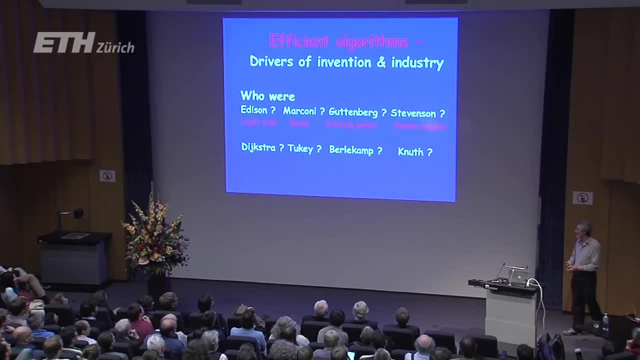 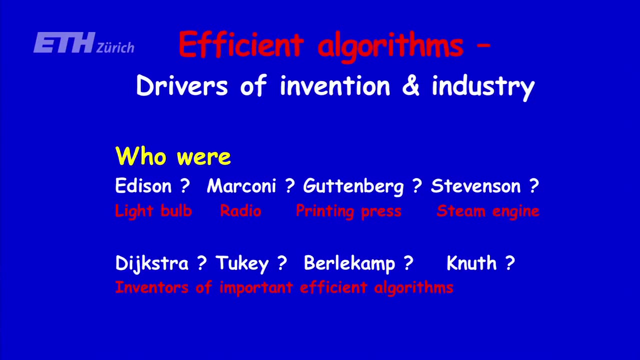 So these guys invented, invented things that affected, you know, Civilization in a big way. And same with these guys, They invented algorithms. So they didn't invent physical objects, They invented these white boxes, And these white boxes then become technology. that that, you know, is really amazing. 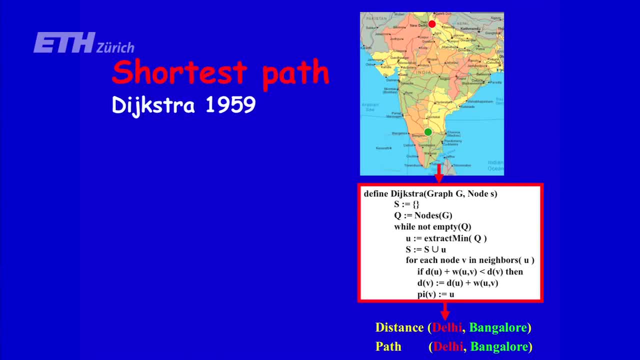 So let me just mention some. Dijkstra developed the shortest path algorithm that you all use when you are. you know you're a computer scientist. Yeah, You know, trying to get from point A to point B, Although in India I would recommend flying. 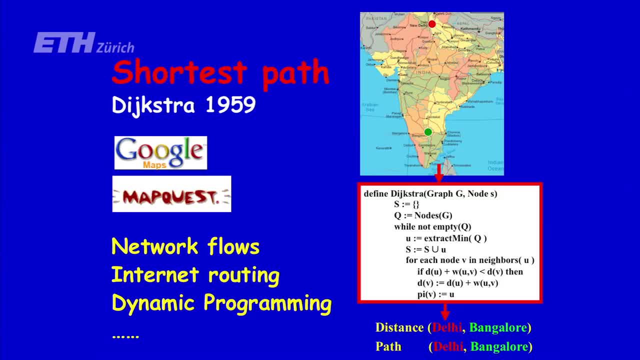 because This is behind all these amazing, you know, split-second answers to to this type of queries or finding the shortest route in in a network and, of course, has an impact on on internet routing, for example. Another basic problem is the problem of finding patterns in text. 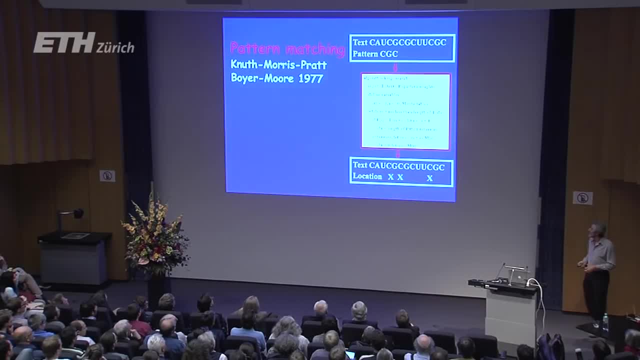 In particular in biological text, but not just. You get a, a long pattern and then another shorter pattern maybe, and you ask: where? where does it occur? And for example, in this example, you know it occurs in these three places. 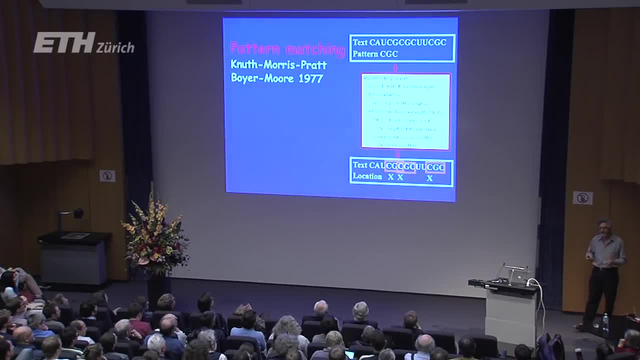 So here's the white box. It's very simple, So I should really stress. most algorithms look like this. They are just a a few lines to describe and to write down as code. They are usually easy. Finding them is a problem. 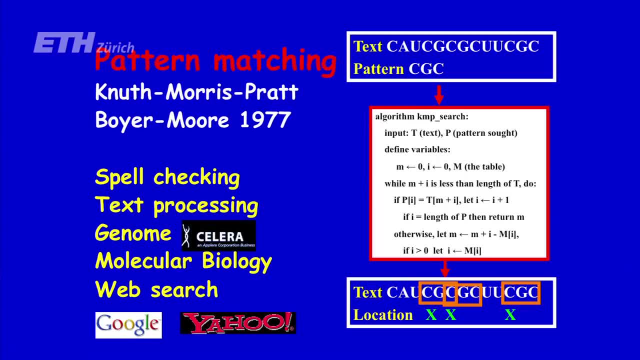 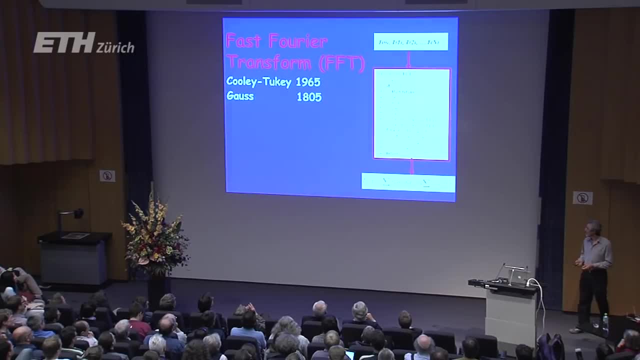 And this again has huge impact on lots of things You know, both on text processing of various kinds, but also on molecular biology and web search, and more and more. Here's another algorithm that many people here, many many here- know, at the hub being 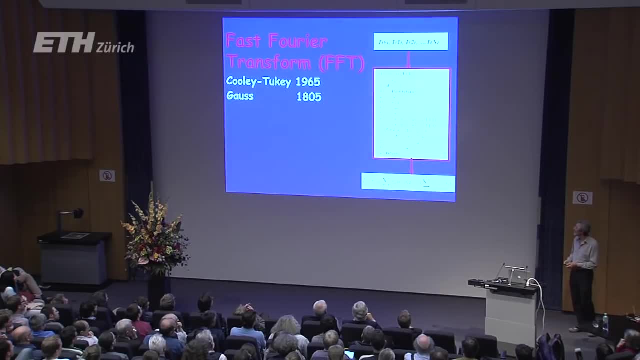 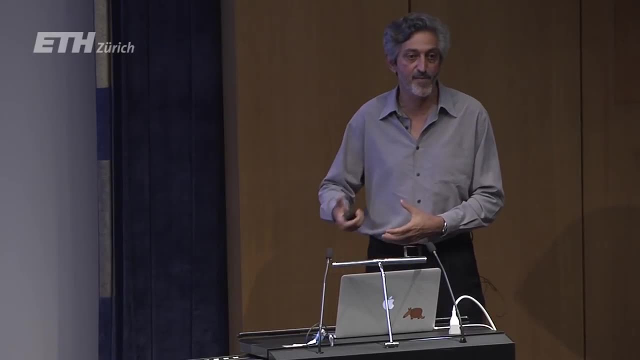 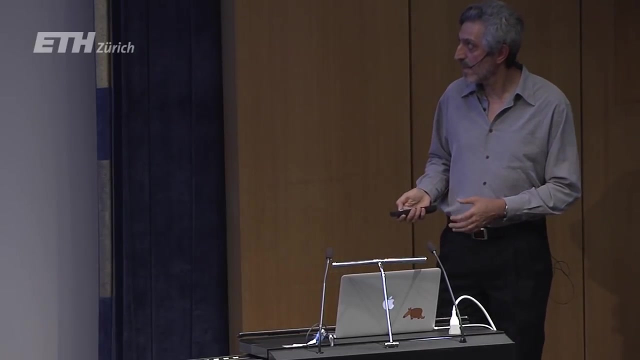 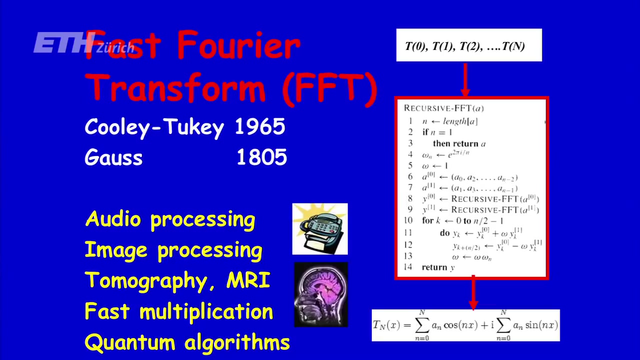 such a famous engineering school, The fast transform, where I will not explain it. but you turn a sequence of numbers into another sequence of numbers In another basis, in another, from another viewpoint, and this turns out to be behind essentially all signal processing applications in audio and image and tomography. 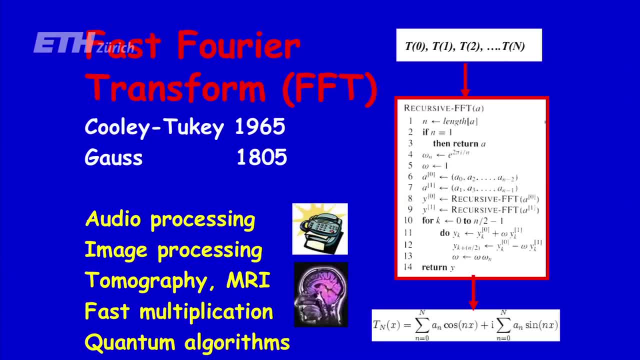 And, moreover, this idea is also behind the fast algorithm that we mentioned before And some of you know of fast multiplication, and it's also very important quantum algorithms and so on. So This is a very short idea that actually Gauss knew about. That is very powerful in applications. 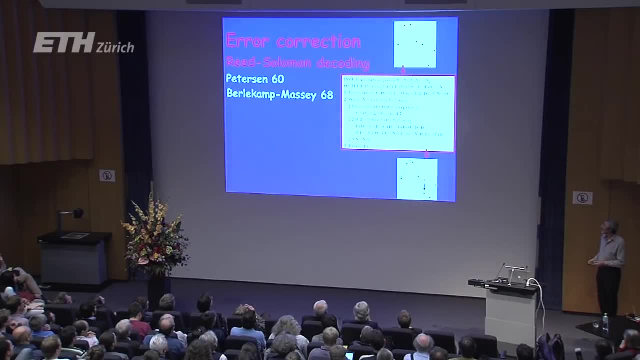 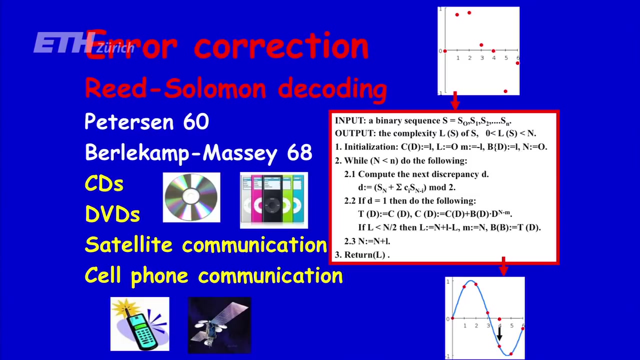 And the last one I want to mention is this algorithm for correcting errors, which another way of writing it, explaining it, is just taking a sequence of points and passing a curve that goes well through most of them, And that's behind the fact that if you take a CD and scratch it, you can still listen. 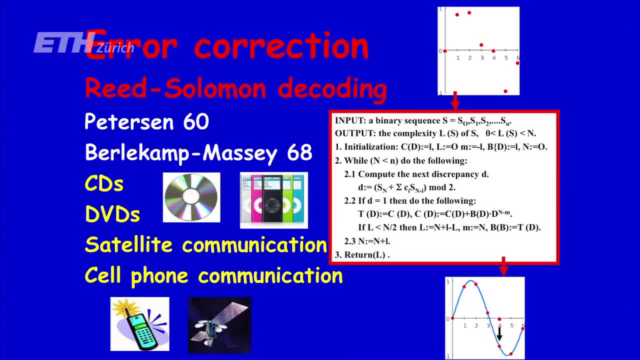 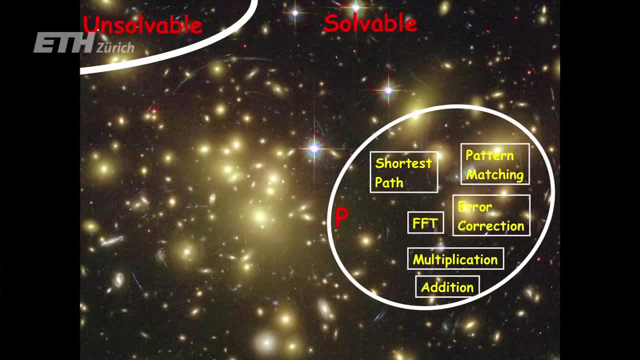 to the music or or see the movement. You can watch a movie without you know noticing, Okay, So There are lots and lots of these efficient algorithms. We all, we put them all in the class B of the problems that we can solve the problems. 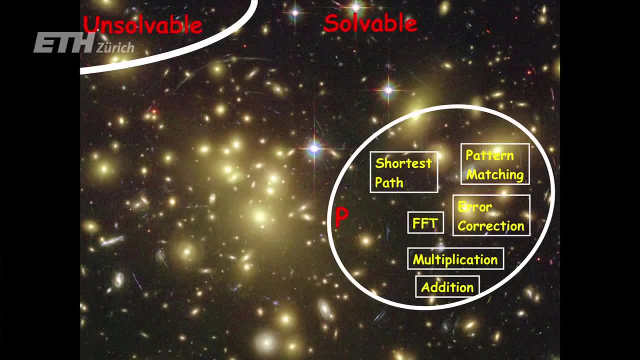 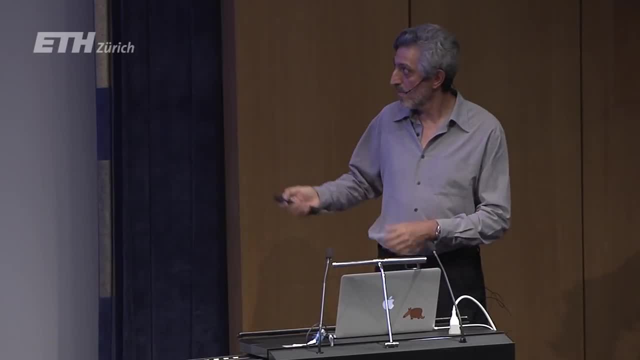 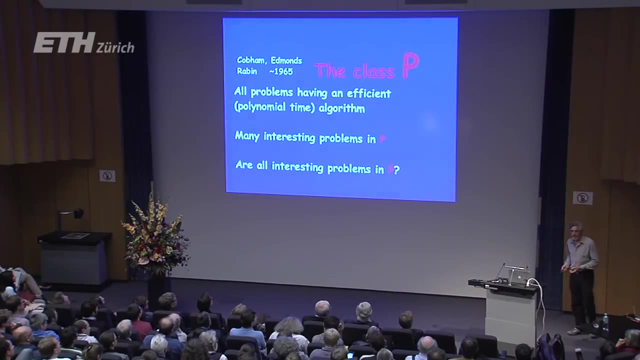 for which we have efficient algorithms. So we understand some small part of the solvable side of the system And, as we said. so we just noted that there are many interesting problems in P. Okay, And the basic question is: are all problems, all interesting problems in P? 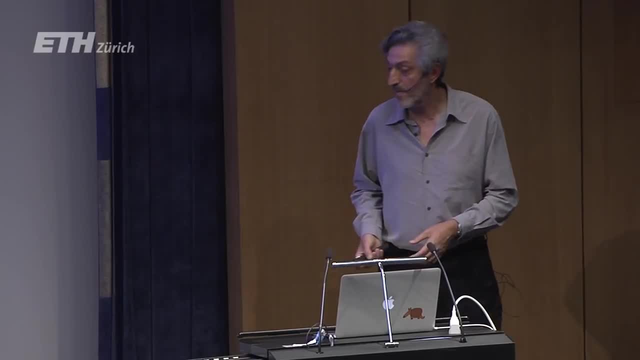 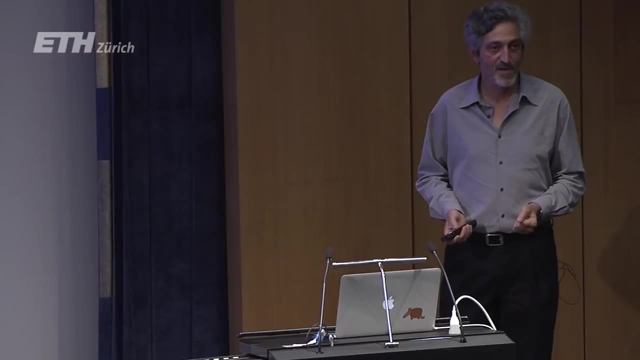 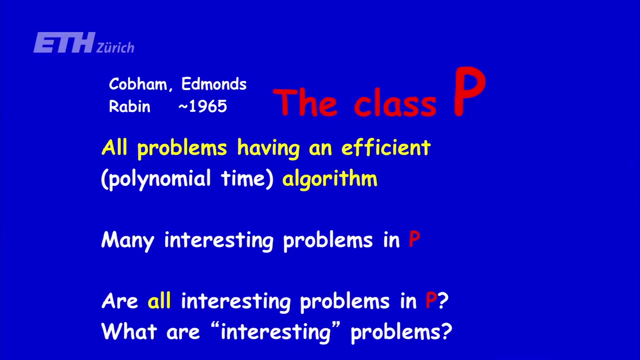 We know that not all problems are there, because there are some unsolvable problems. So at least the problems we can hope to solve are in P. So this brings a really really basic and interesting problem. What are interesting problems? You know? can we even? you know how? how can we answer this question? 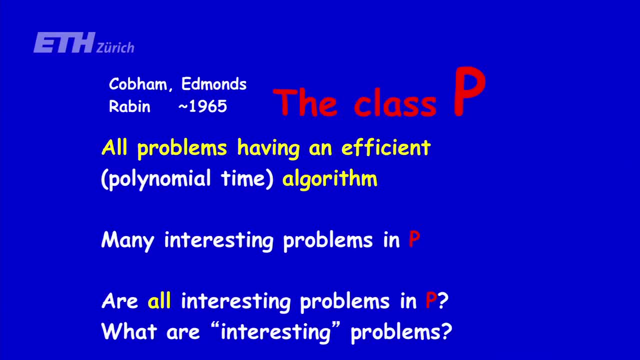 And again, it seems that this point philosophical- What is interesting to you may not be interesting to me, and so on, But I want to convince you that there is an objective answer to the question: what are interesting problems? and to actually give you a mathematical definition of all interesting. 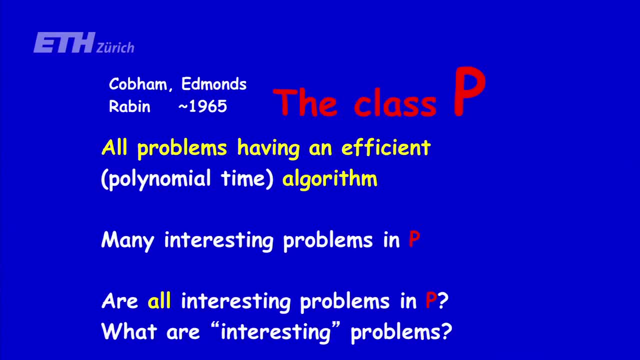 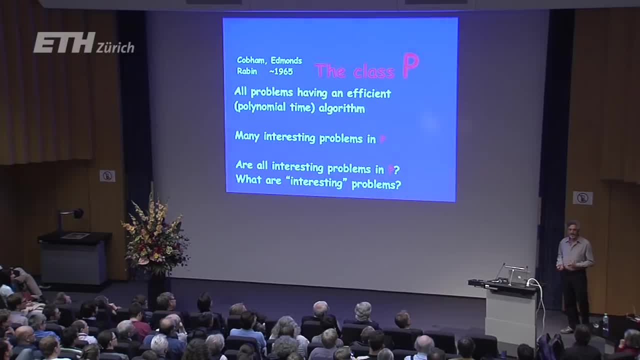 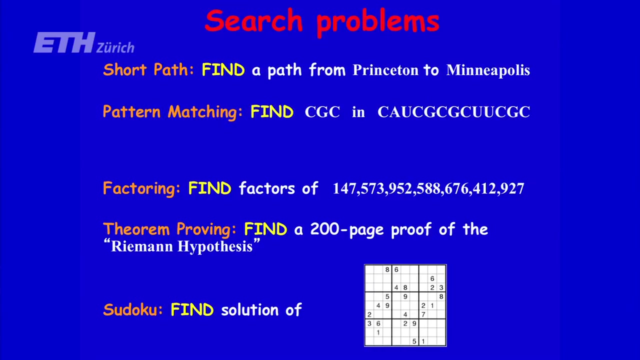 problems. This, of course, would be the class NP. Okay, So let's see how we can arrive at the definition. Let me actually stop any. any, did I lose anyone yet? Okay, Okay, Okay. Very polite people, the Swiss. 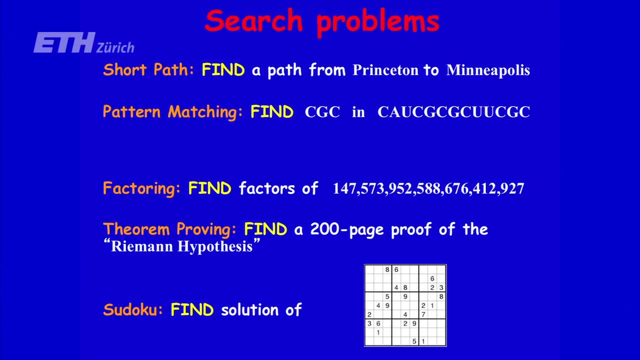 Let me restrict myself to search problems, problems in which we are finding, we are looking for something, And most problems can be cast in this way. So here's a collection of problems that we mentioned. I think all of them Shortest path. you know, I give you a network: find the short path between two points. 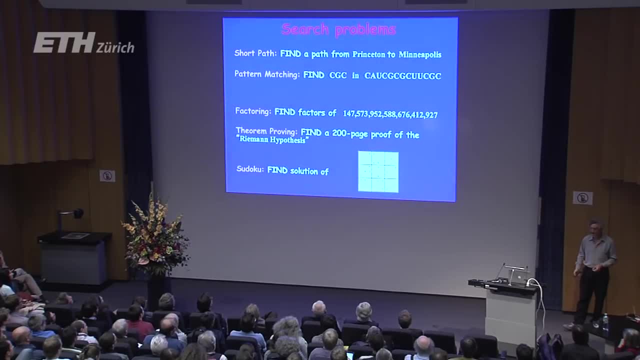 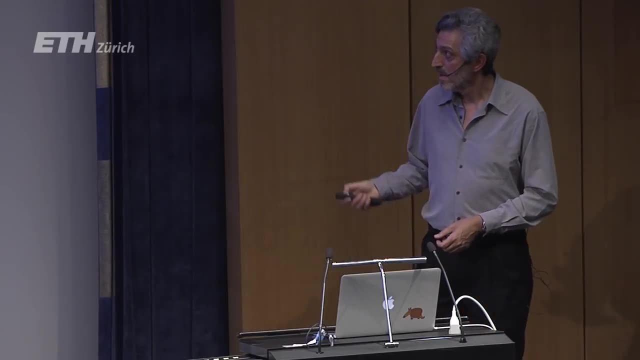 Pattern matching: I give you this pattern and text. Find the pattern in the text. Integer factoring: I give you a number. find the factors. I give you a statement like Fermat's last theorem, find the short proof that proves it. but do it for a new, something we don't know, like the Riemann hypothesis maybe. 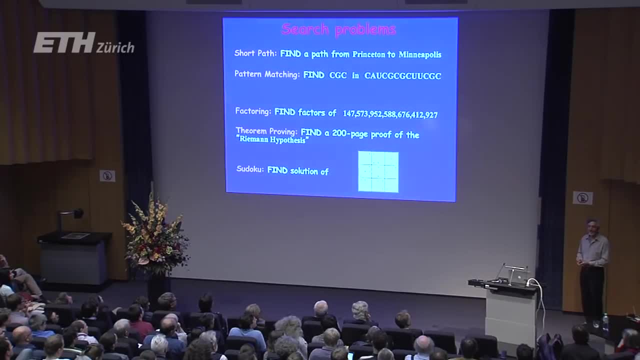 And the Sudoku problem. I give you a Sudoku puzzle. you know, find the solution. So what is common to all this? There are five problems there. What is common to them, And the most obvious thing, is that they are not the same complexity-wise, because these 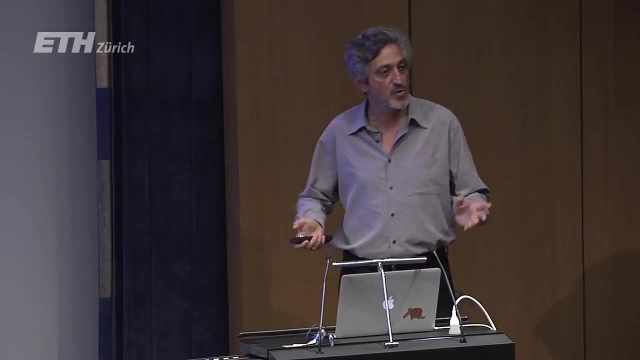 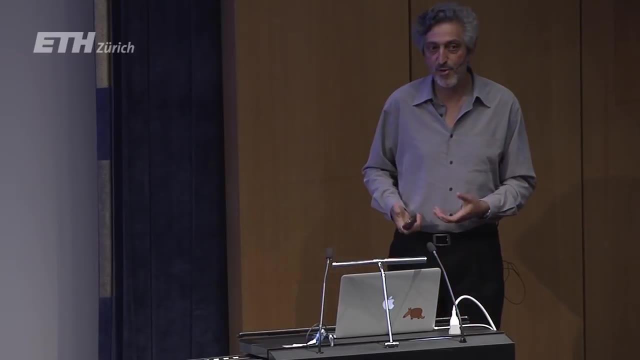 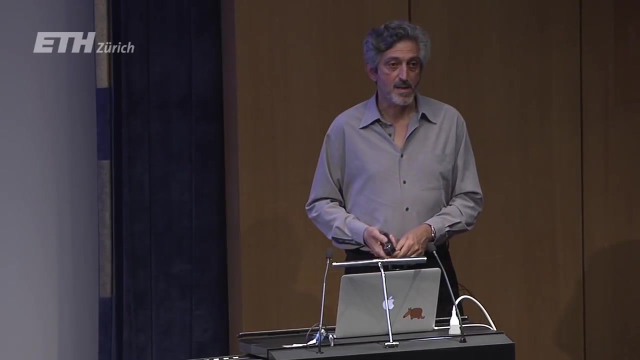 we saw are easy, and the other three, at least we have some intuition that they are difficult, maybe in qualitatively different way, but at least they don't seem to have very efficient methods to be solved. But there's something else which is. 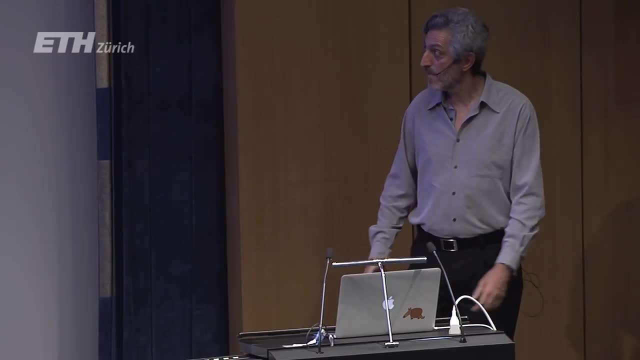 So that's not common, not the complexity, at least as far as we know today. But what is common to all of them is that in all of them, if you have a solution, or if your friend has a solution, they can convince you of it very quickly. 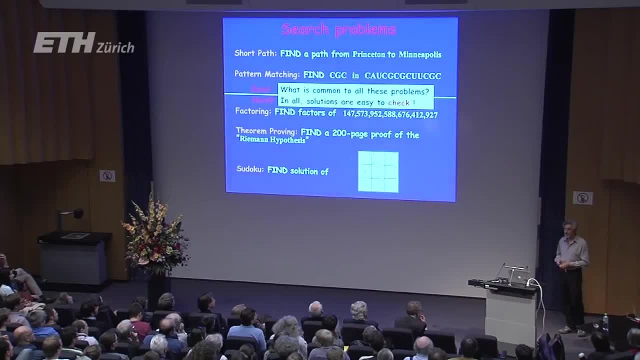 Once a solution was found, it was very easy to check, And that's a key property of all the five problems there. So for the two above, you know they are easy to find, so of course they are easy to check. But what about these guys? 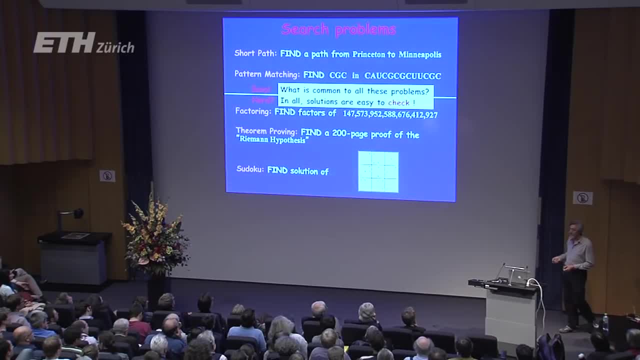 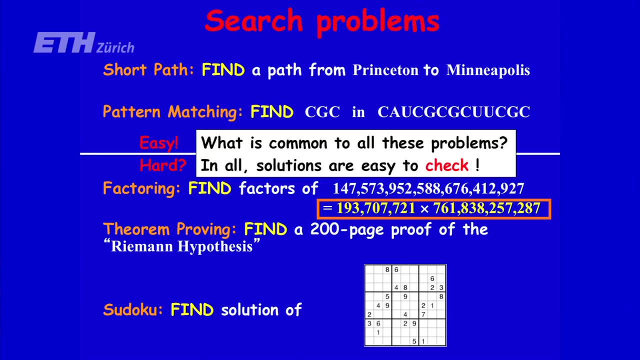 Let's check With the factoring problem. if I knew the factors I would give them to you and then you just run the multiplication algorithm. So that's easy to check. If I had the proof of the Riemann hypothesis big, if I would go to Mark and you know, 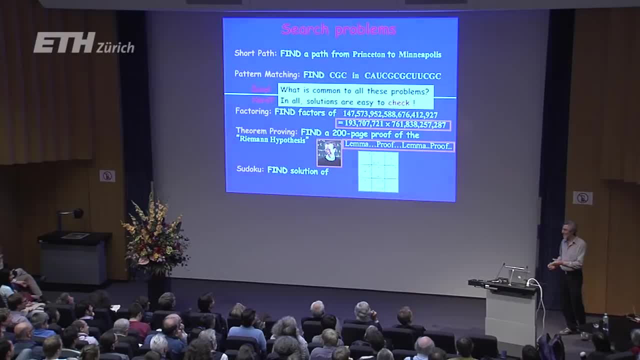 I think that's better. Andrew Wiles would go to Mark and show him the manuscript and then he will study it, maybe for a year. But you know, after all it's a sequence of, you know, small steps in some proof system. 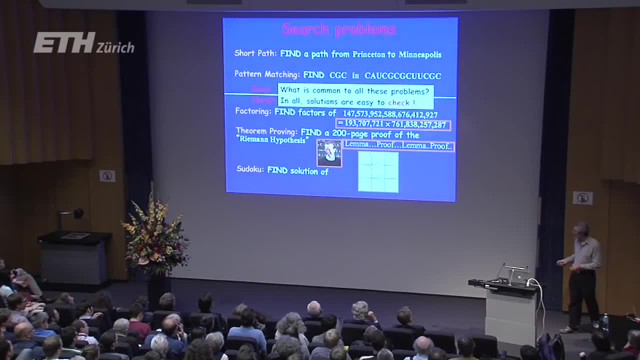 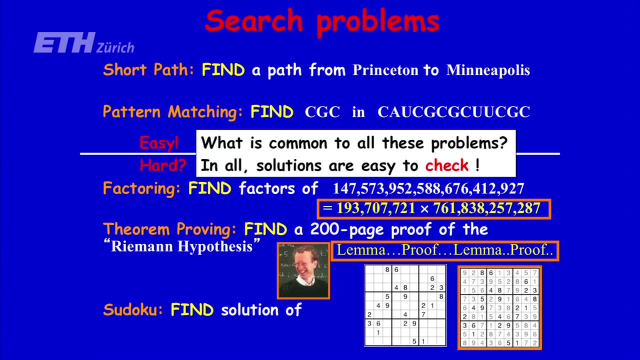 and can be verified efficiently even by a computer. And if I knew how to solve this Sudoku puzzle, of course I'll show it to you and you'll just check the obvious things that you know. the rules of Sudoku are satisfied. 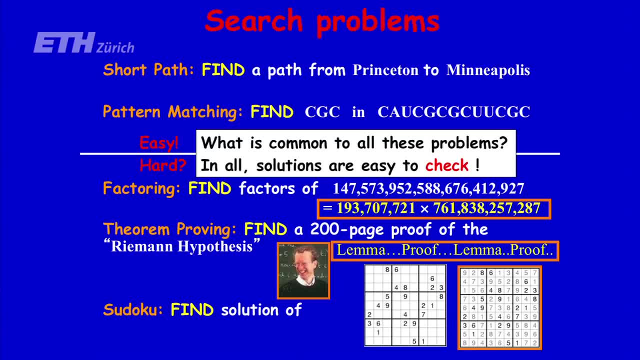 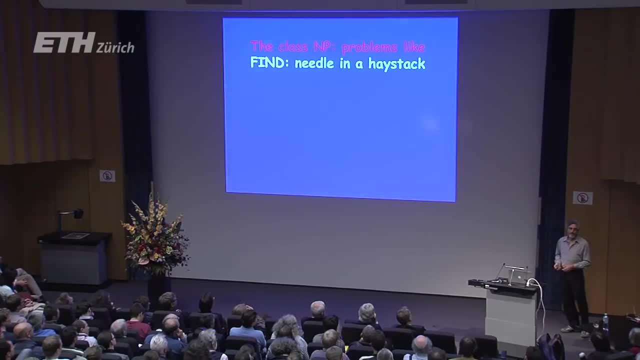 So all of them. you know, whether easy or hard, once you have a solution it's really easy to verify that the solution is correct. So verification has an efficiency, Thank you. So that's the class NP. So in some sense you can view it as a problem of finding a needle in a haystack in the 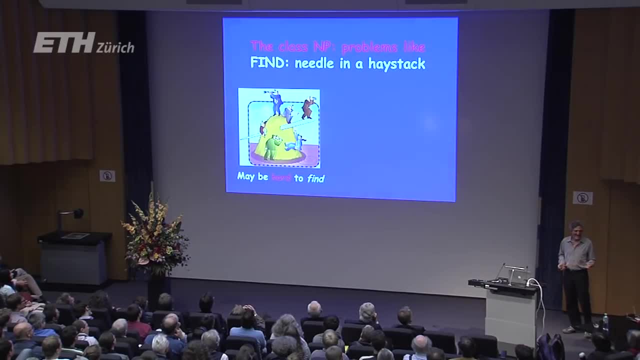 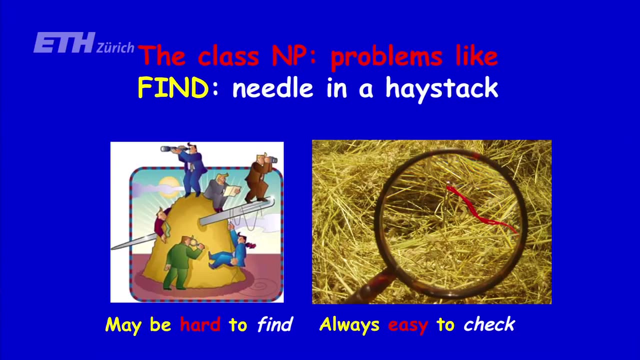 sense that you know, maybe the needle is hard to find, But once I you know, I point to it and I give you a magnifying glass and you know you see it okay. So once you have a solution, it's very easy to convince others that it's a correct solution. 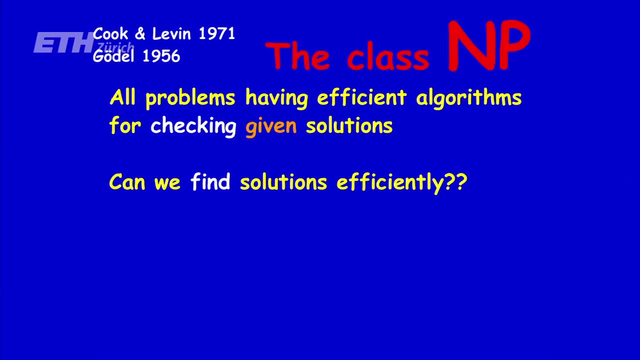 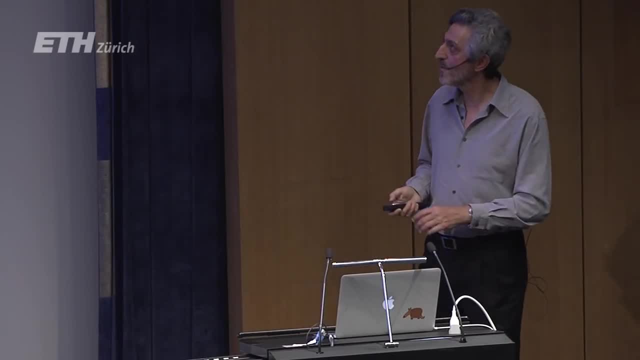 So that's the class NP and the class NP was introduced in the early 70s, although Gader sort of knew about it. as we understand today is all the problems that have efficient algorithms to verify, to check that solutions are correct. 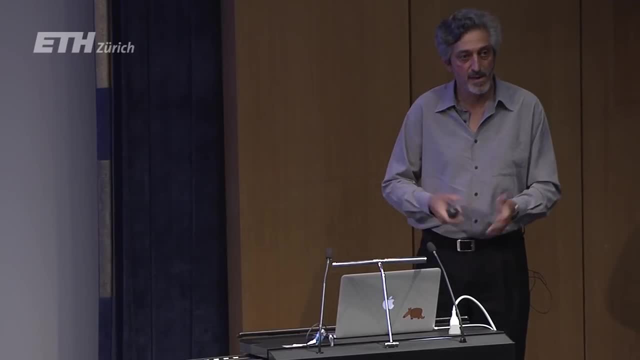 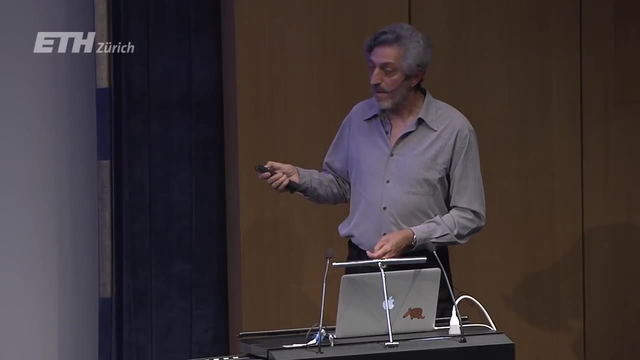 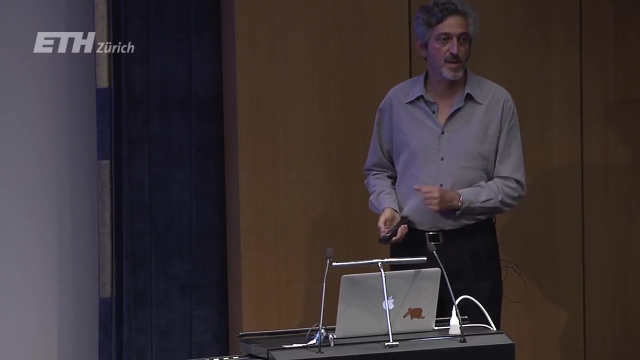 Maybe not to find them, but once they were found and fell from the sky, we can check if they are correct or not. And the question is …. Yes, For these problems, just these problems, can we find solutions efficiently? These are the interesting problems, and we ask whether they are easy. 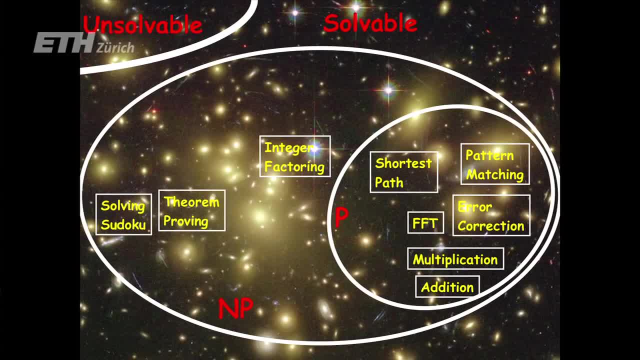 We can draw the class NP in our night sky and it certainly contains P, because everything that we can find easily we can verify easily, but not necessarily the converse, And we know some problems that we mentioned: factoring and solving Sudoku and proving theorems. 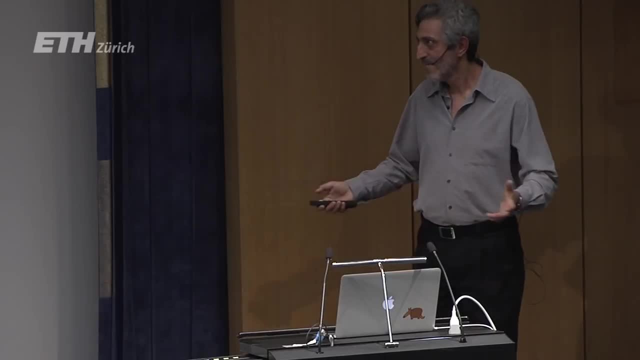 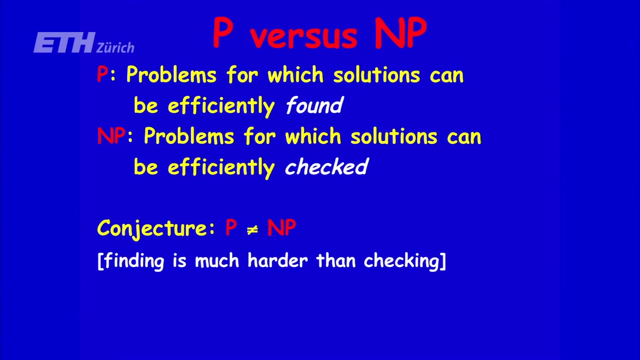 and you may know others, like traveling salesman and Boolean satisfiability and lots of other problems. they lie in NP And these are what I want to call the interesting problems. Now I have to justify this. Let me repeat the definition, just so that everybody is with me. 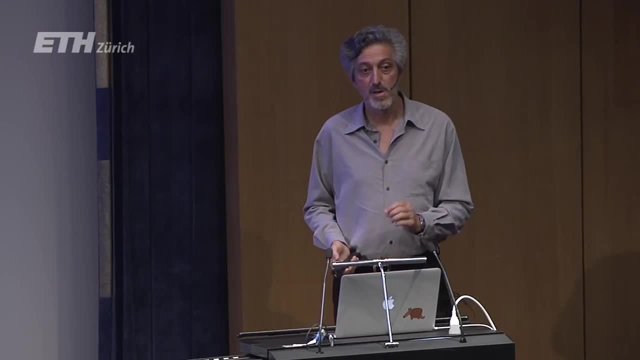 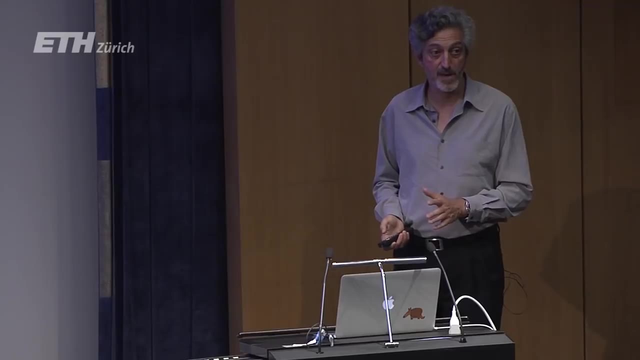 So P is a class of problems for which solutions can be efficiently found and NP is a class of problems for which solutions can be efficiently verified. Check, And here is what most people believe. P is different than NP. Sounds almost obvious. 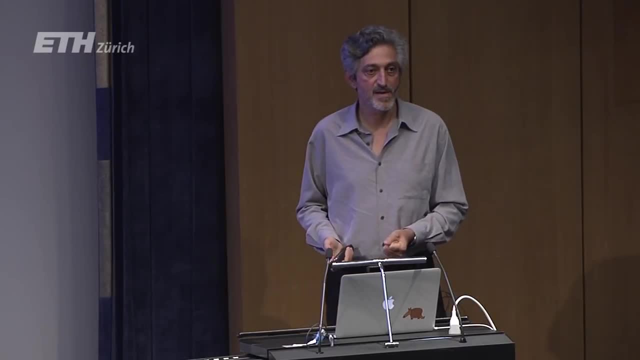 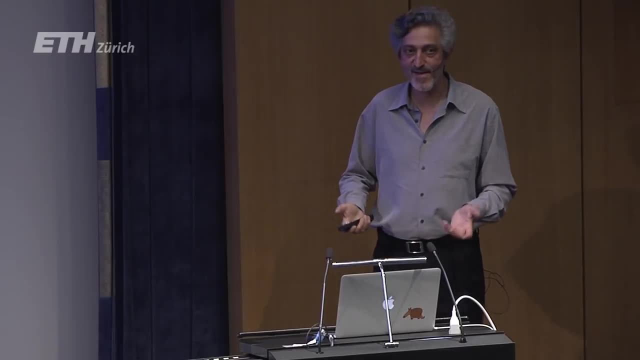 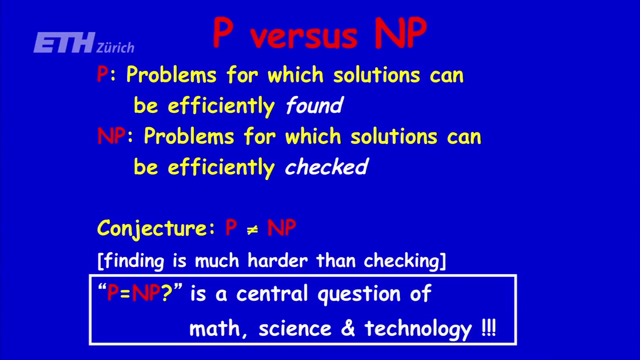 Checking is easier than finding. Finding is harder than checking. As obvious as So why don't we have a proof of this yet? It's a good question, So we don't know why, we don't know whether it's true and we are not quite sure why it's so hard to solve yet. 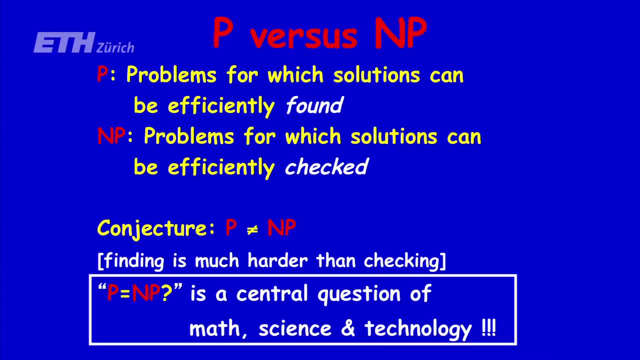 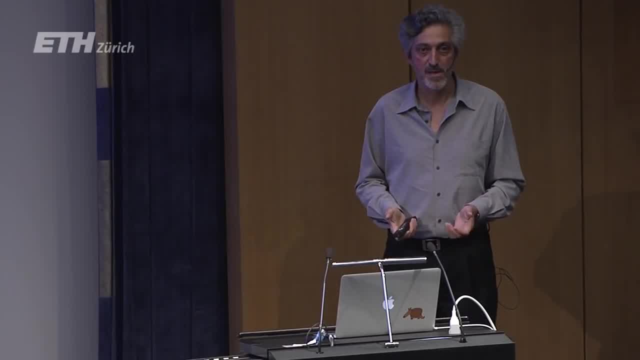 but what I want to convince you is what I promised in the beginning- is that this is a fundamental problem that everybody should be interested in. In fact, we are hoping that you'll join us in trying to solve it. So I want to claim that it's a central question in mathematics. 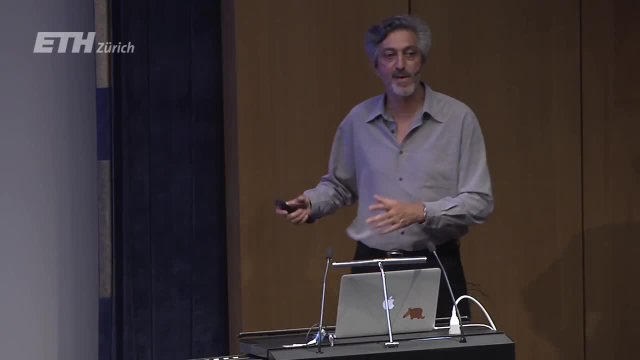 in science, in technology, So you don't have to trust the clay people that are giving a million dollars for it. You'll see that you'll be very happy to know. if it's true, Almost doesn't matter what you do. So let me, in order to prove this, let me sort of 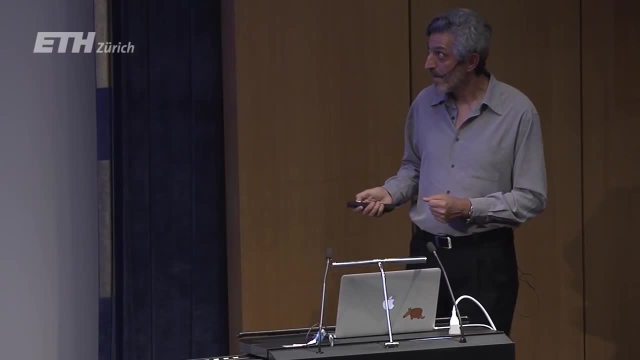 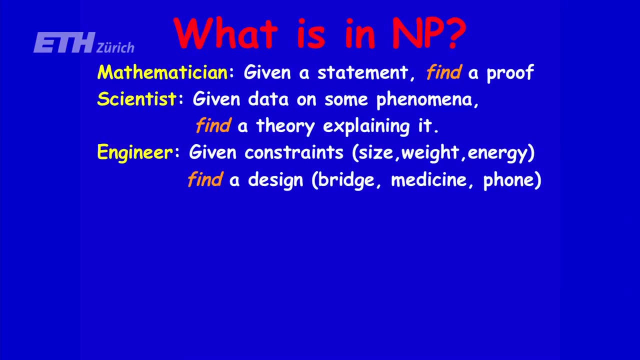 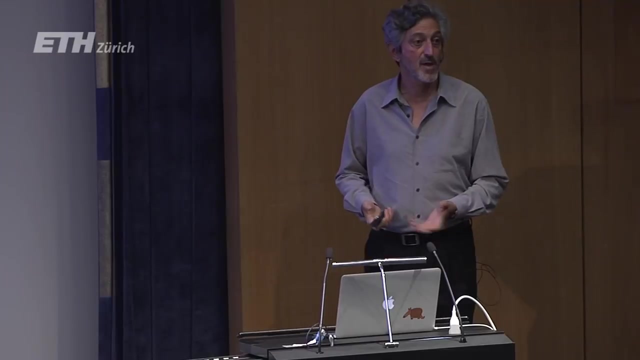 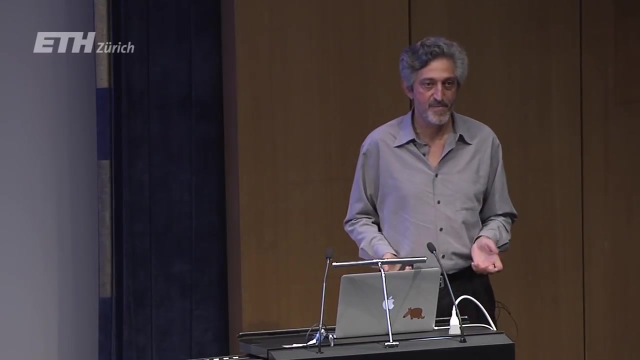 play a caricature of several very important professions that are probably represented well in this audience- Mathematicians, scientists and engineers- And let's try to understand what they are doing when they go in the morning to work. I claim they are just trying to solve some search problem. 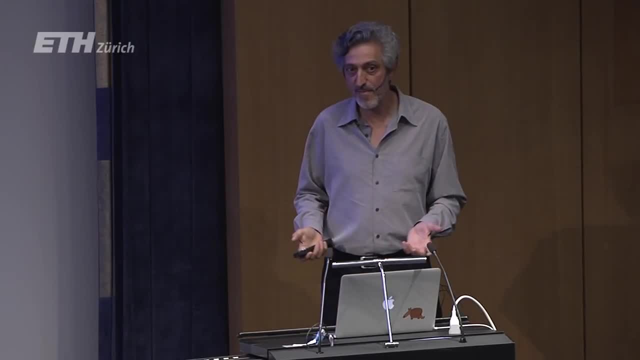 So it's somewhat caricaturistic, but it is if you think about it. that's what they are doing. A mathematician usually is faced with some statement. mathematical statement is trying to find a proof. Scientists usually, you know, is facing some collection of data. 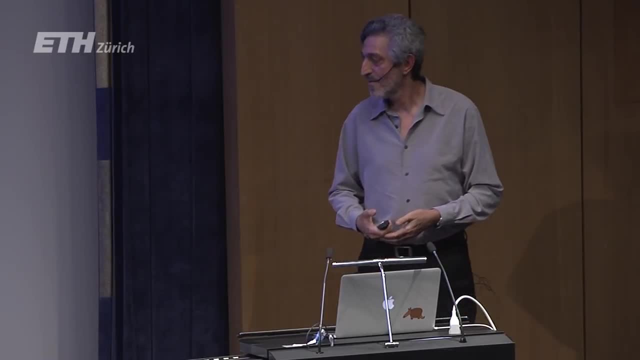 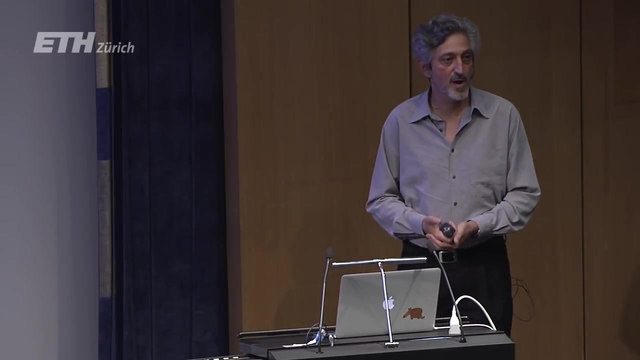 whatever field, from astronomy to biology to whatever you want- and is trying to find a theory that explains this. data And engineers typically are given some. you know they are going to build a bridge or find a drug to cure cancer, or you know are designing some gadgets, a new iPhone or something. 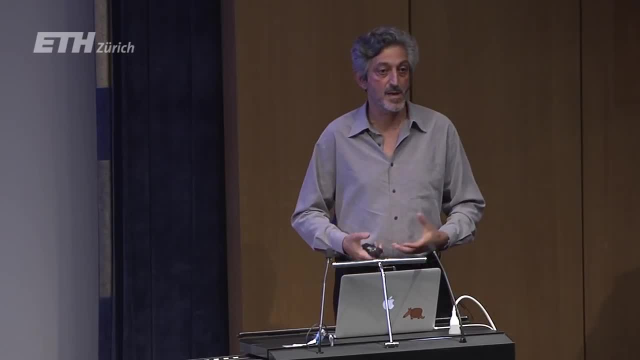 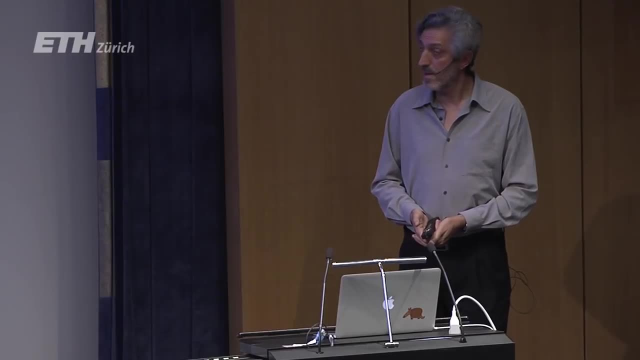 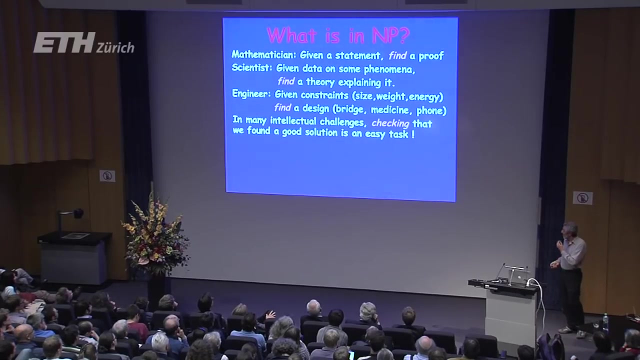 And they have some goals and they have some constraints, and they are trying to find a design that fits all of them, that satisfies all of them. Now, what is common to all these professions, besides trying to solve search problems? I claim that in all of these, in many, not just in these- 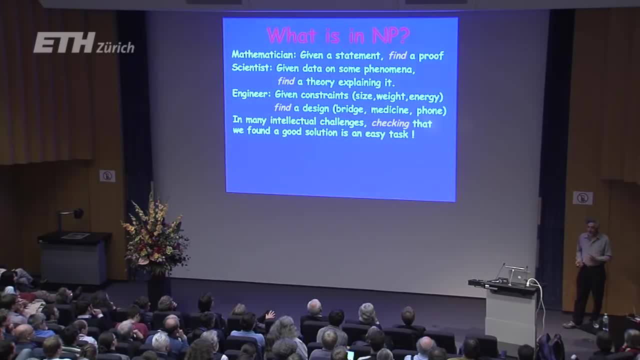 in many, many intellectual challenges. maybe the problem each of them is trying to solve is really difficult, But somehow checking once you've found the solution, once your colleague found the solution, it should be, it must be easy to check that it's the solution. 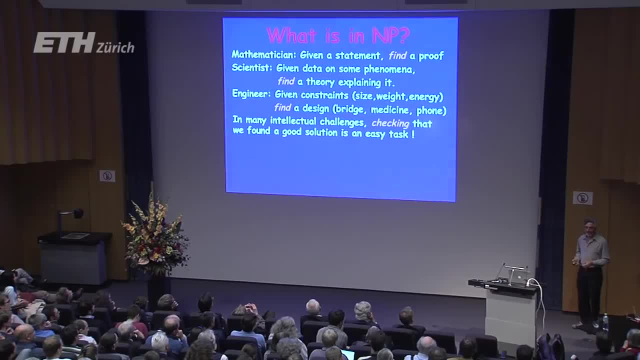 Why is this so? That's a claim, that's my claim. You may not believe me, but here the answer is almost as obvious as this. You know, I claim that. if it was not the case, that it's easy to check. 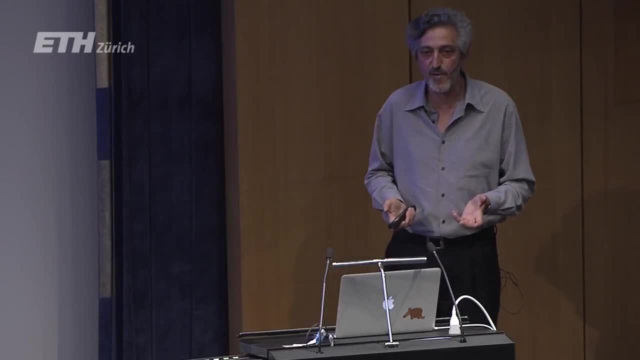 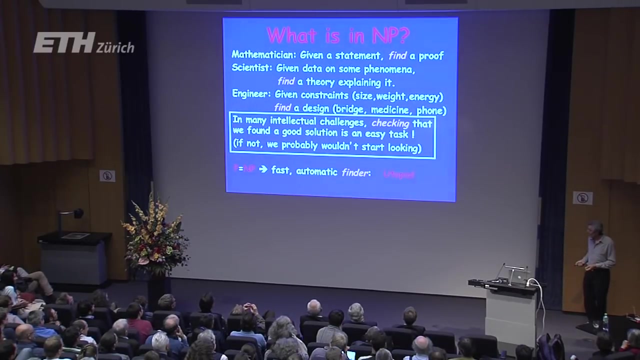 none of these guys would even start looking. I mean, when are you looking for something that you wouldn't know when you found it? What's the point? So all these problems basically are NP problems. They are all problems in NP by our definition. 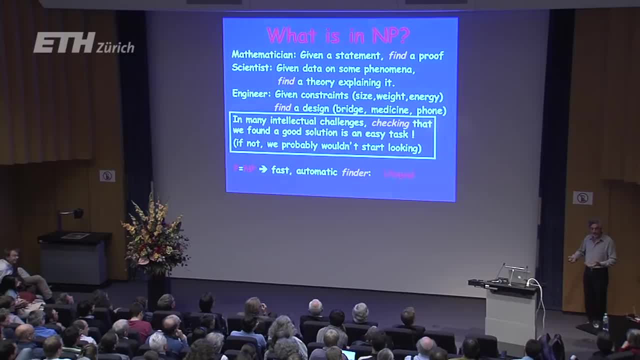 Of course I am stretching. you have to formalize it in each case. but suppose you formalize it, then these are NP problems. Yes, The이가or. 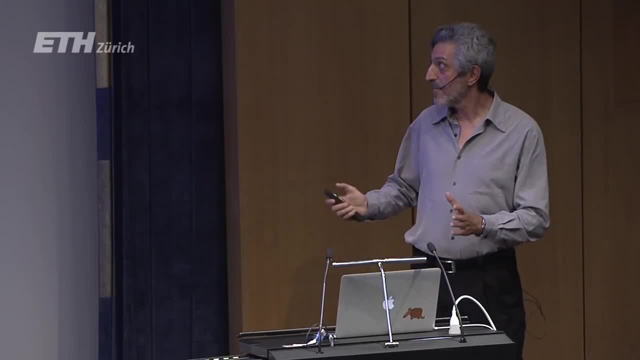 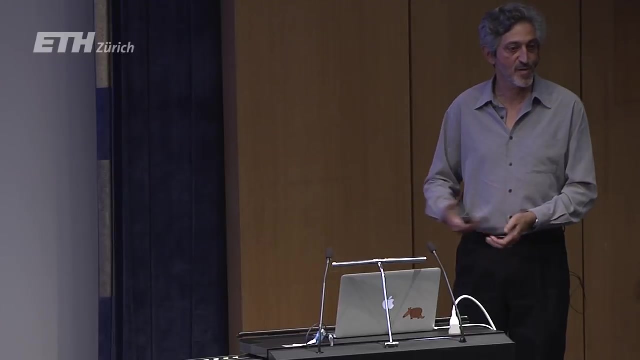 That's a very good question, So let me defer this. So it's like I said, it's a characteristic picture and the question was about where does the asymptotic point of view that I used for defining computational complexity of problems come in here? 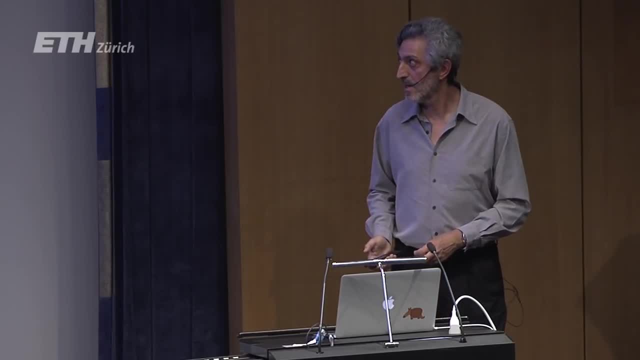 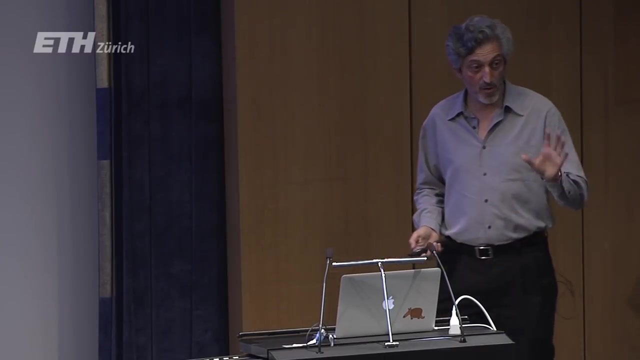 So in many of them you can work it into the problem. it captures a huge number of problems that are actually attempted by various, let's say, scientists, And we'll see examples that are better than this one, although also this one can be cast there. 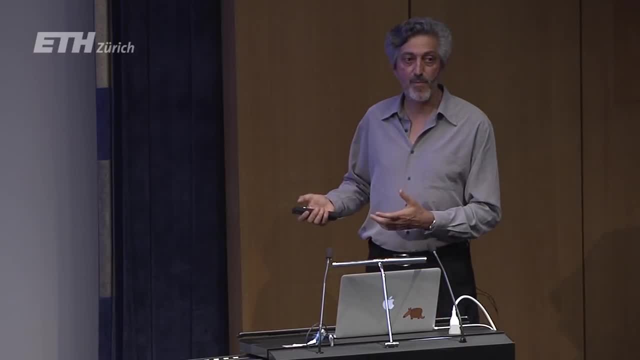 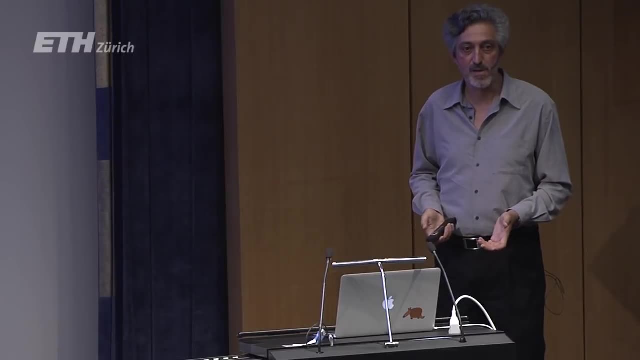 but I don't want to get into it now. So if these are problems in NP and if P equals NP, then all of these problems have fast solutions, right? This is what P is. P means that you can find efficiently anything. 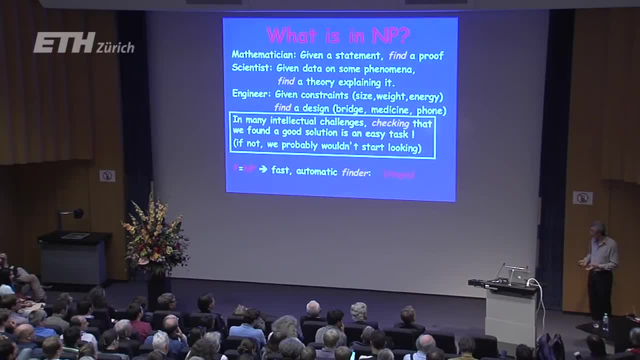 You can solve your problems fast. If P equals NP, then every problem for which you can check efficiently a solution, you can also find it efficiently. So if P equals NP, it's sort of utopia: We can solve every problem that we are interested in. 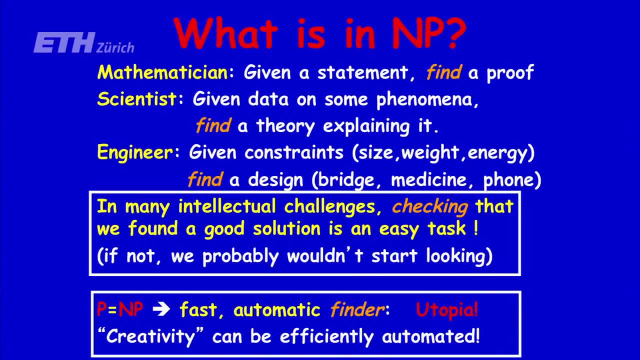 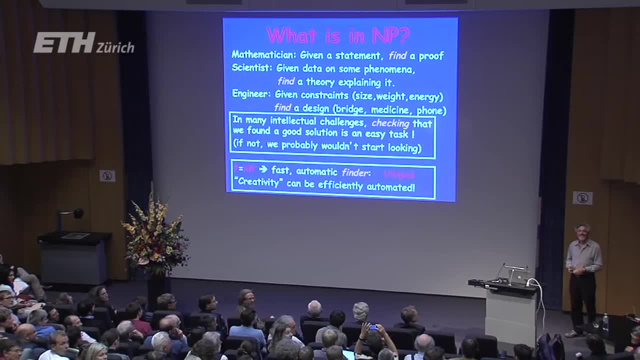 So somehow this kind of creativity, at least the creativity we assign to scientists or mathematicians, would be efficiently automated. We could. all our jobs can be replaced. Yes, I know of a problem which is interesting, but I'm not sure it's not NP. 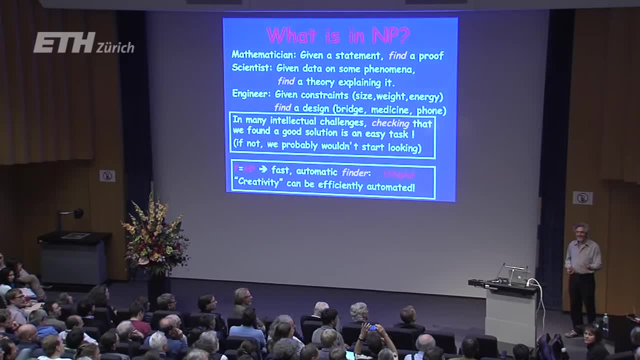 That's the problem of chess. Very good, Yes, I have to find an algorithm to solve a certain game. I'm very much interested. I'm very interested in having that, even though it's not trivial- to prove that this really is a solution. 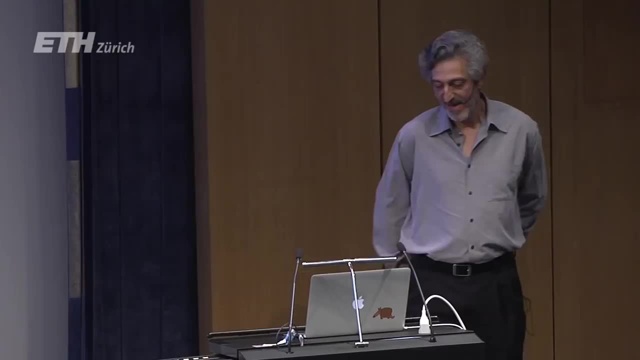 That's another excellent question. So the question was about the complexity of chess and playing chess. Verification of winning strategy in chess does not seem to be easy to check. I have a good answer for that and we can also deal with it in the question. 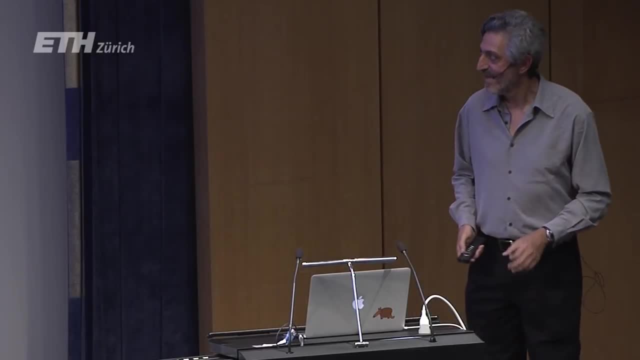 So it's a great. I love your questions and we can go into them. It's very good. So we saw some exceptions to the rule, so it must be a rule, right? So let me tell you how we try to understand this P versus NP question. 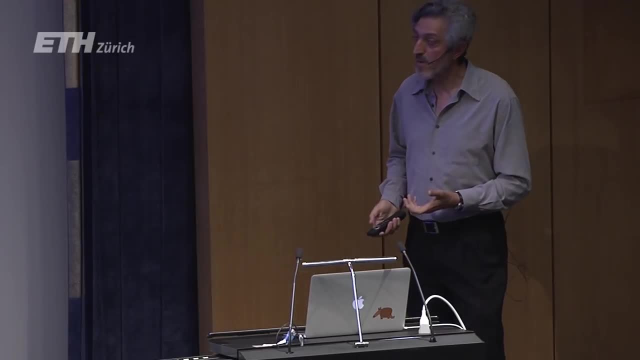 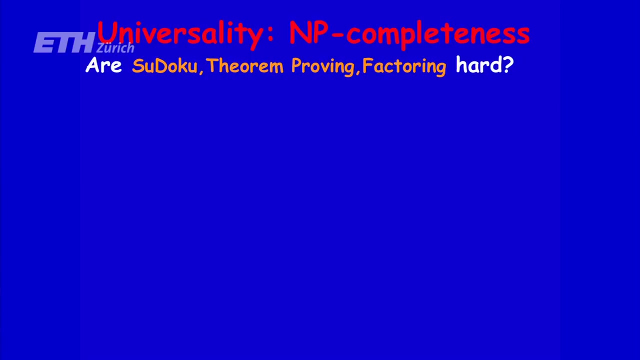 as we cannot resolve it yet- And this is universality. There is a phenomenon, this universality, this NP completeness, that imposes a a surprising structure, I would say, on this class of problems in NP, And let me tell you by example, then we'll talk about it in more generality. 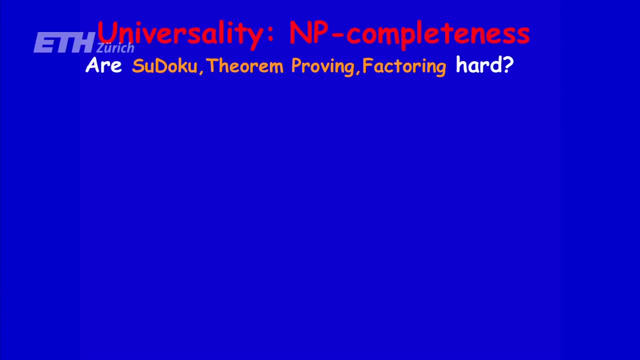 So we want to know. you know, we don't believe that P equals NP, really. So these problems we talked about, these examples that I gave, are they hard, as they seem to be, In all these cases, the best algorithms we have. 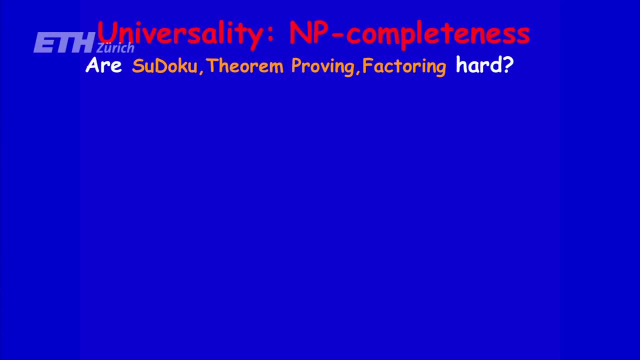 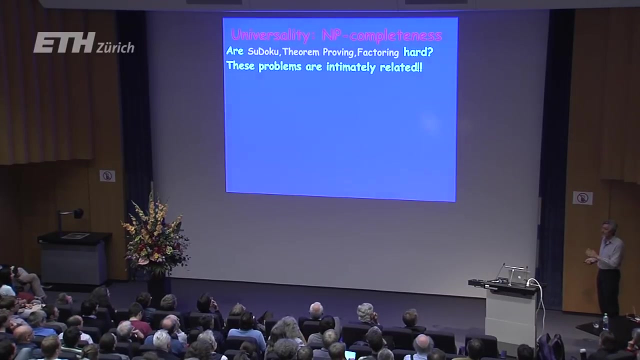 are something like brute force exponential time. So here is. you know what's the relationship between them? If you've never seen it, then you should be surprised by the following. So they are really intimately related, and they are related in the following way. 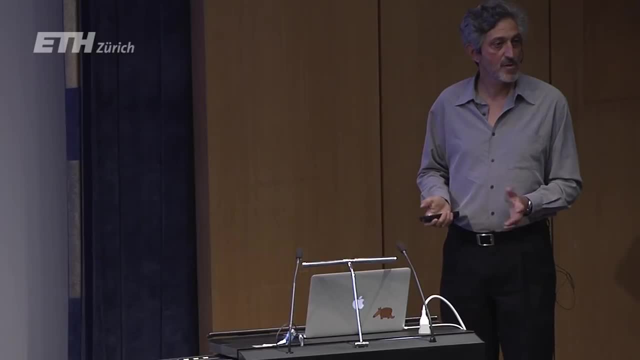 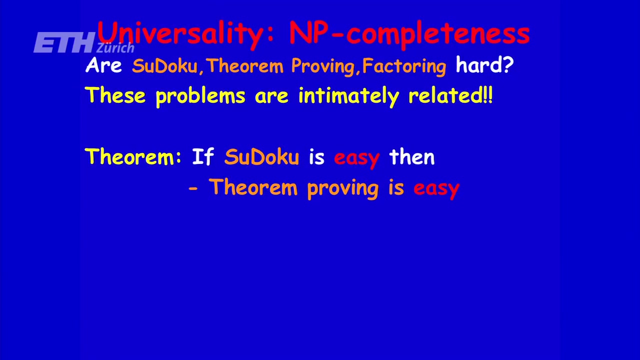 Suppose you found an efficient algorithm to solve Sudoku problems, larger and larger Sudoku problems, as easy as addition or multiplication. Would it be good for anything? And the answer is yes, big time. If you have an algorithm that would do that, then you would have an algorithm that would solve efficiently. 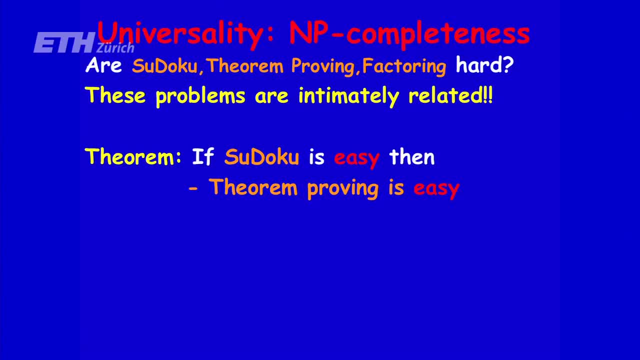 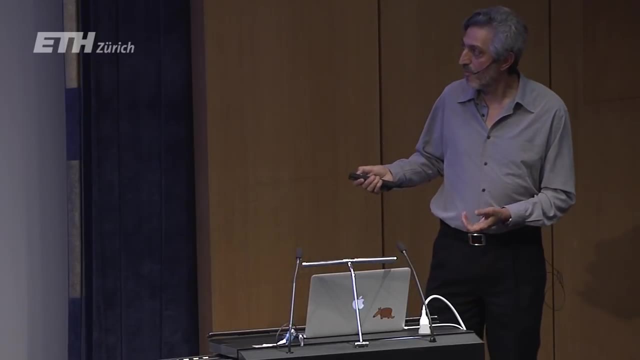 that will prove efficiently, theorems will replace mathematicians, And it will also factor integers and break all cryptographic systems. So, somehow, Sudoku. how do you prove it? Well, you prove it. the proof is, I'm not giving it to you. 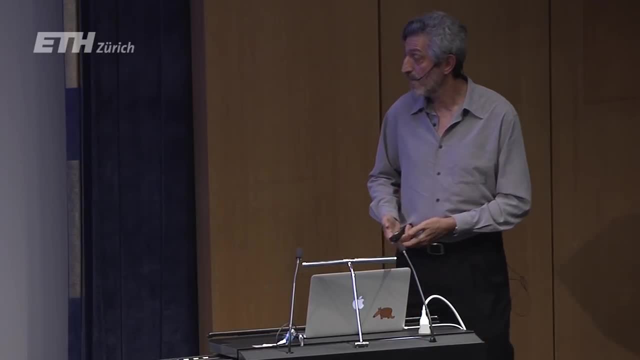 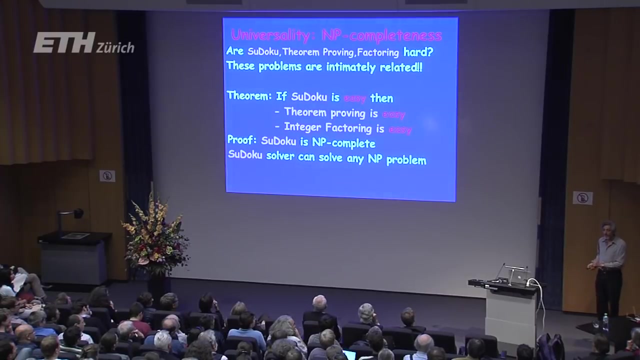 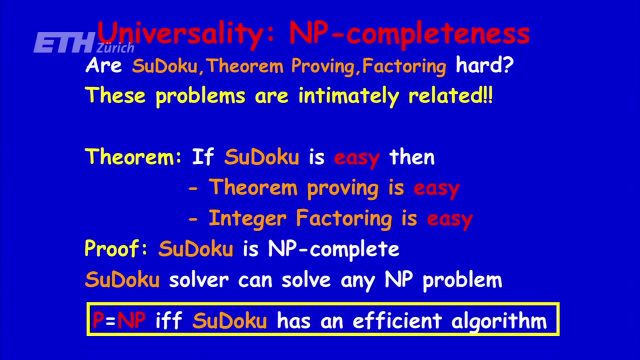 it's actually not difficult once you understand the framework. It's one of these universal problems. Sudoku is as hard as any problem in NP. If you have a Sudoku solver, then it solves every problem in NP, And so I promised you a mathematical definition for the P versus NP problem. 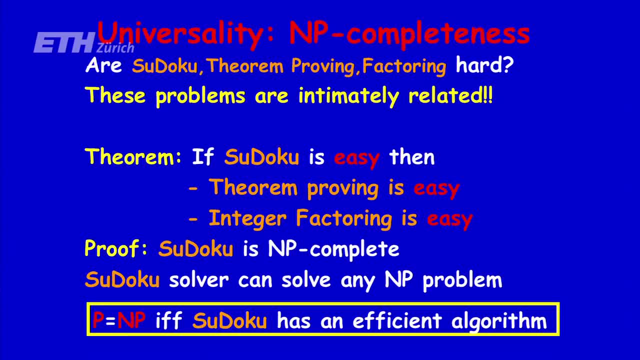 Here it is: P equals NP if, and only if, There is a framework, There is a fast algorithm to solve Sudoku. Sudoku, you understand, computer programs, you understand. so that's the question, that's the mathematical formulation of this problem, And it's sort of surprising, I mean, it's really, maybe amazing. 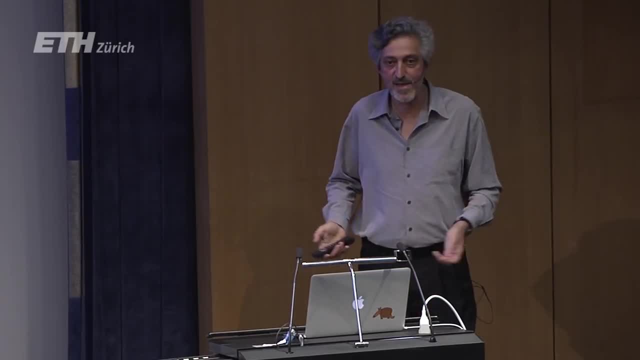 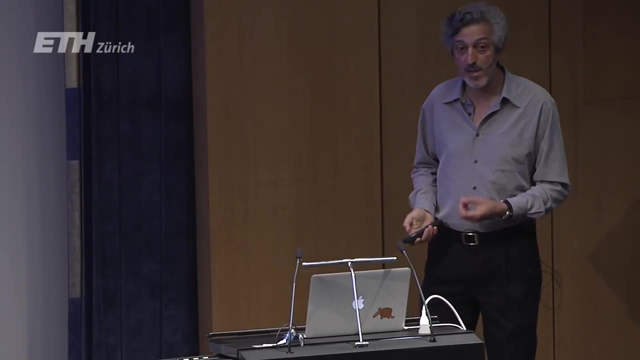 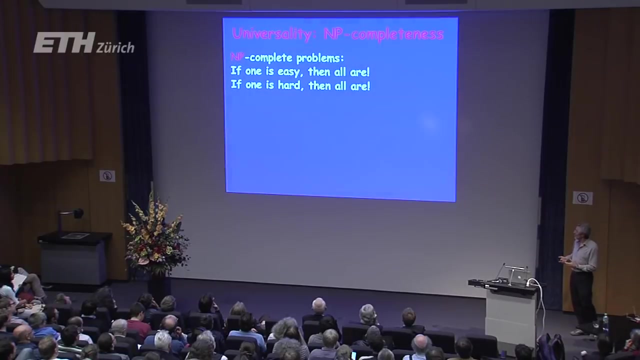 that a problem that everybody thinks is nice entertainment when you are flying from Newark to Zurich. but you know it's as fundamental as proving theorems. So this let me repeat what it means to be NP-complete, like Sudoku NP-complete problem. so it's a subset of all problems in NP. 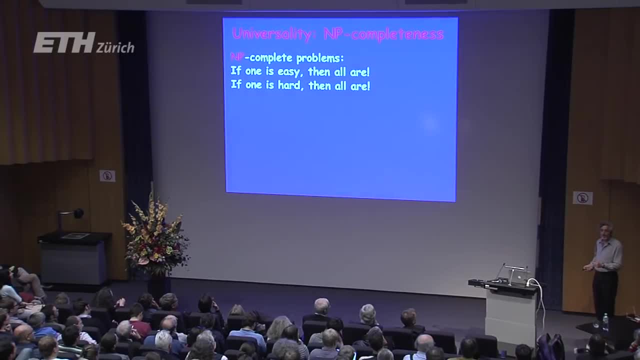 and if you have such a problem and it turns out to be easy to have a fast algorithm, then you've automatically found an algorithm, an efficient algorithm, for every problem in NP, for every one and one of these problems. And if you could prove that it is hard. 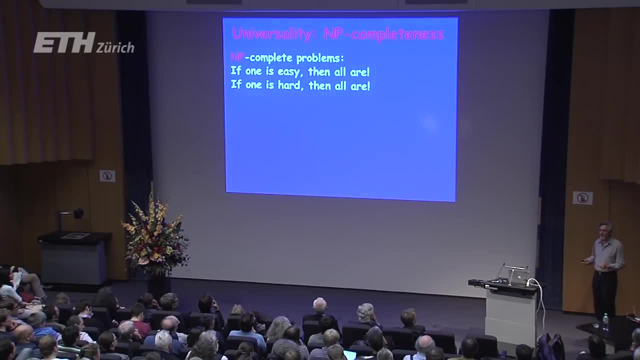 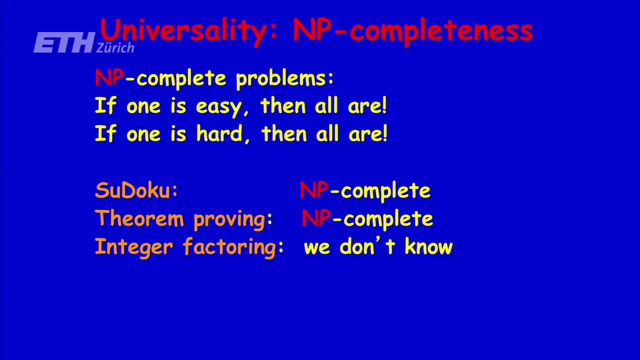 then all of them are automatically hard, NP-complete problems. carry on their shoulders the difficulty of the NP class together. And I just told you Sudoku is NP-complete. I didn't tell you, I'm telling you now. also, theorem proving is NP-complete. 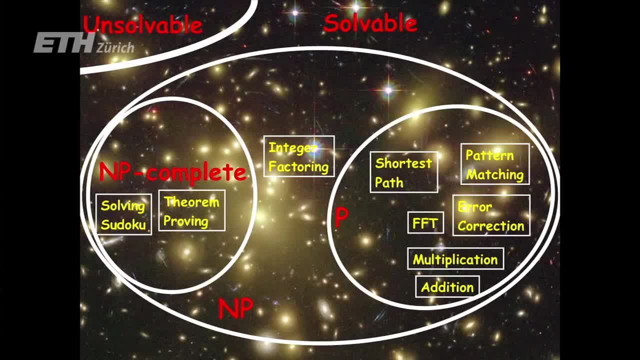 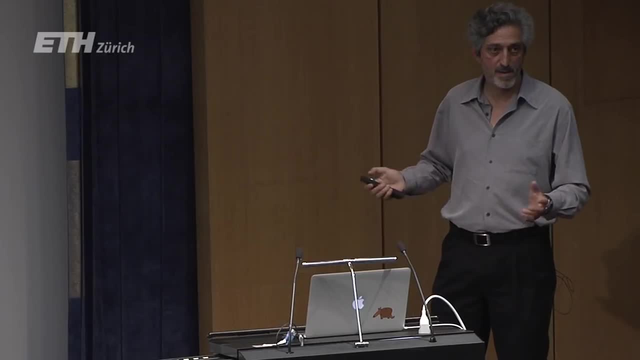 And about factoring. we don't know actually. So if we look now at the map of the sky, we see that in NP we have the easy problems and somehow we have the hardest problems, the NP-complete problems, And if any one of them falls here, then P equals NP. 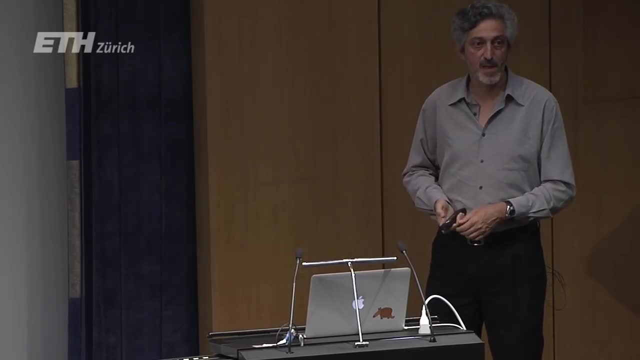 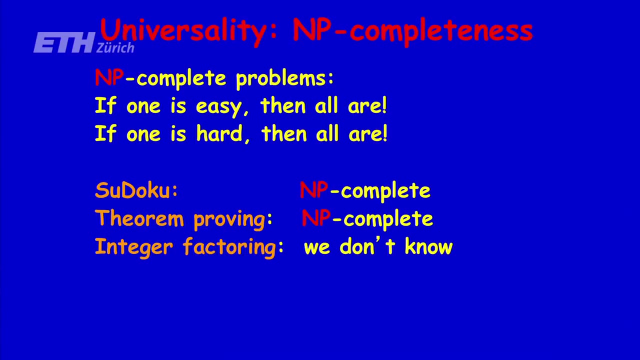 If any one of them does not fall here, then P is different than NP, So we are getting a better and better picture of it. Now here's a maybe more remarkable thing about NP-complete problems. So we saw one or two such problems. 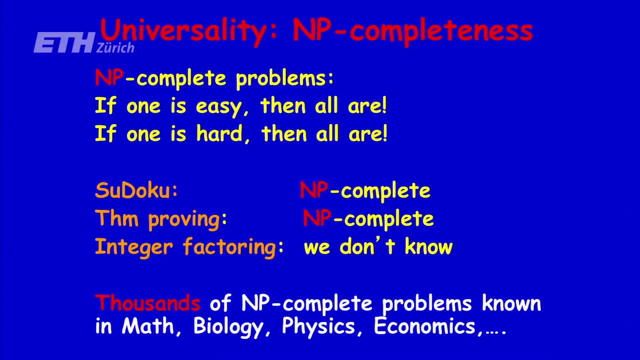 and you wonder how rare or common this phenomena is. How many such universal problems should you have? And it turns out. it took time to understand, but by now we know that there are thousands of them, And not only in computer science. There are problems like this all over science. 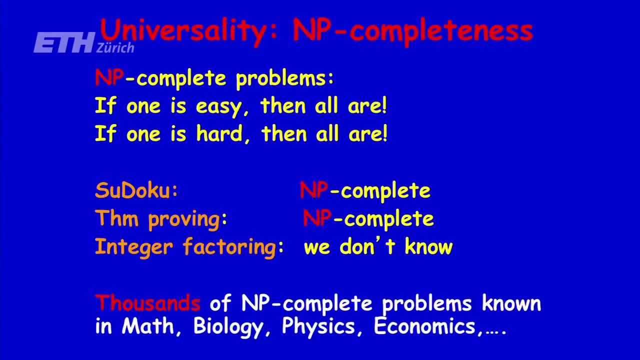 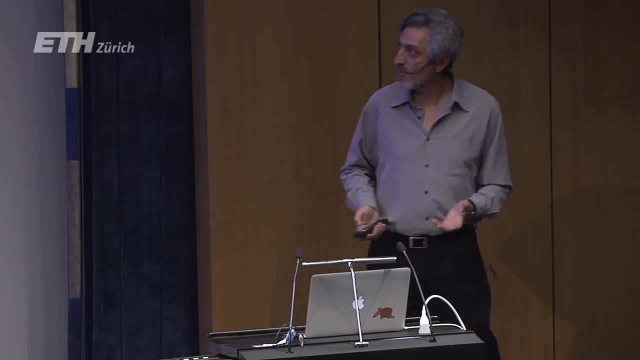 in mathematics, biology, physics, whatever you want, economics. And just to prove it, you know you. just To prove anything right, You go to Google, and in this case Google Scholar, and you say: find me papers with titles containing NP-complete. 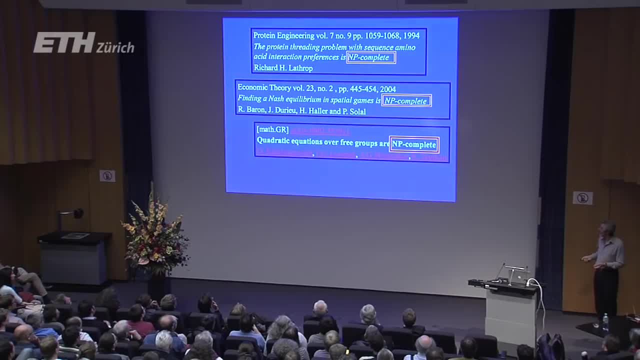 And you find such papers in any journal you want. you know, in economics and what is this? Physics? I can't read like this. But anyway, in every discipline of science you will find. not just find, there are hundreds of them. 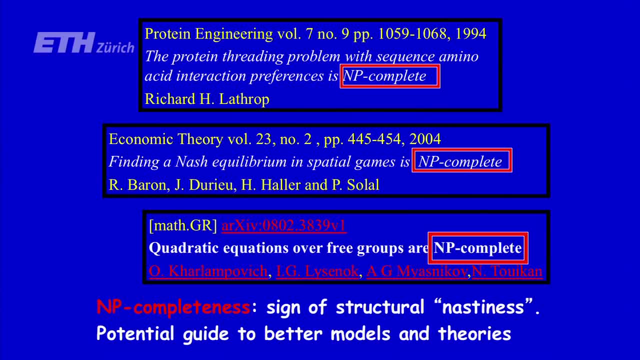 There are hundreds of such problems in every discipline. So why should these sciences be interested in this computational aspect of a problem? Why should they even bother to learn a concept that was born in computer science? Well, because, as it turns out, NP-completeness, even in fields which don't talk about computation per se. 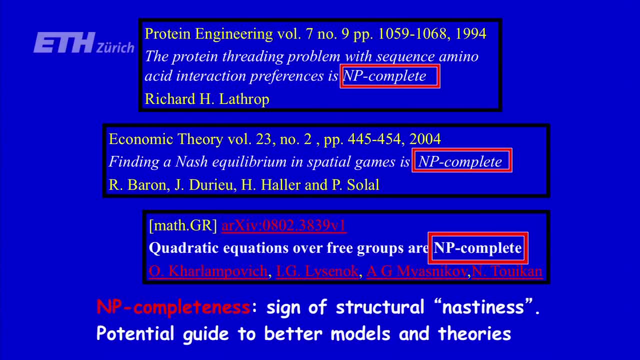 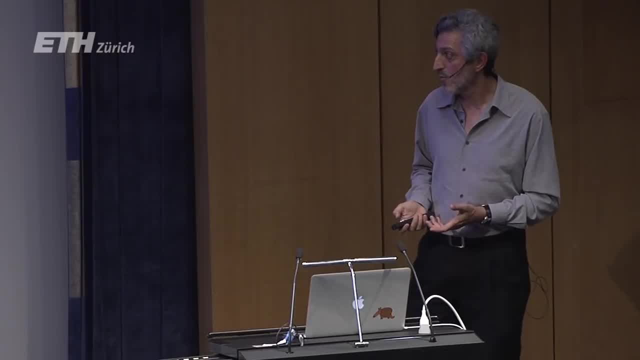 it captures some sign of complexity or nastiness of problems, And actually knowing that the problem is NP-complete offers guidance to understanding better models and theories about this, whatever natural system you're looking at, So, for example. so here are some three examples in which I want to explain. 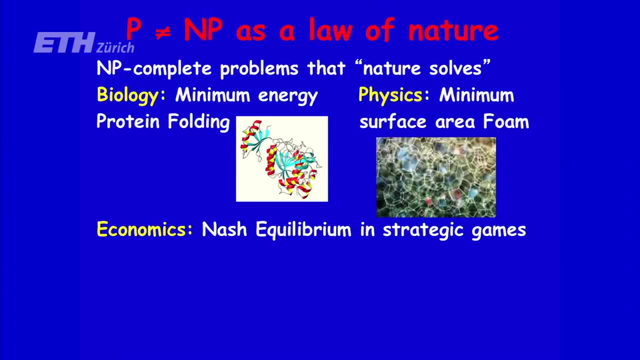 why it would be good for all scientists to add to the things we know about the world, these laws of you know, the conservation of energy and second law of thermodynamics, to add also the axiom that P is different than NP, And the reason is the following: 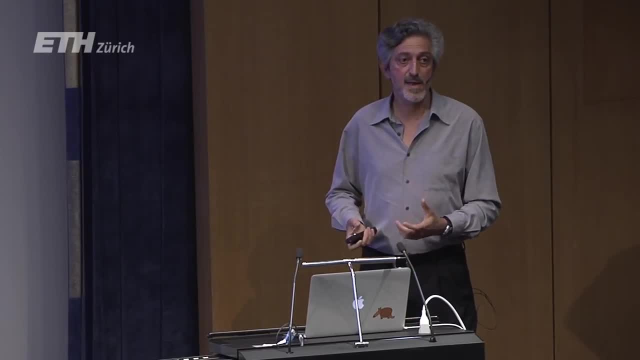 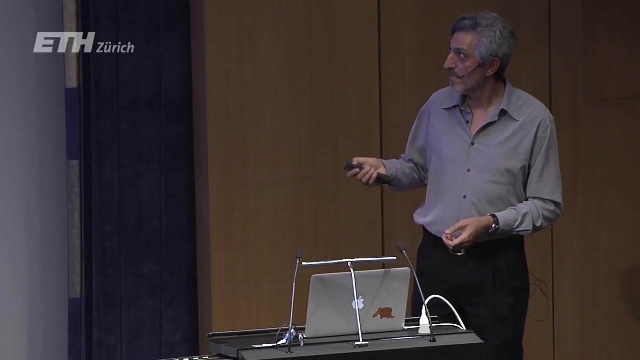 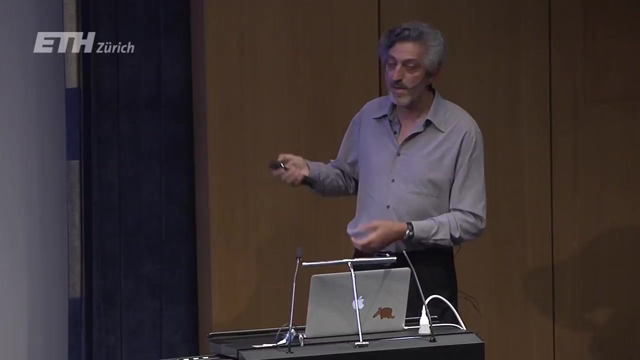 So there are systems for which the models that exist seem to suggest, if nature is efficient, that they solve some problems that are NP-complete. like nature folds protein. However, protein folding is an NP-complete problem. Nature, you know, finds maybe minimal surface area. 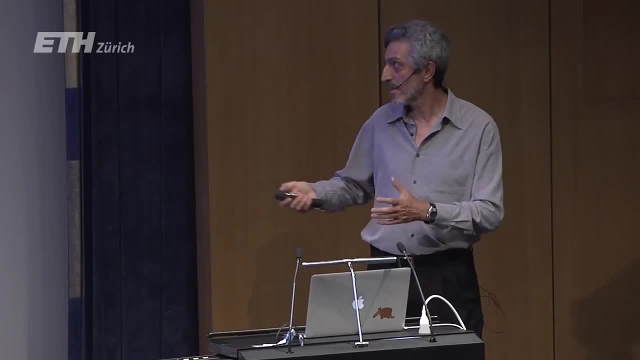 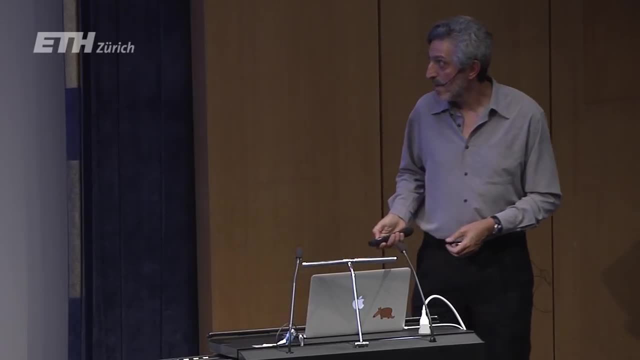 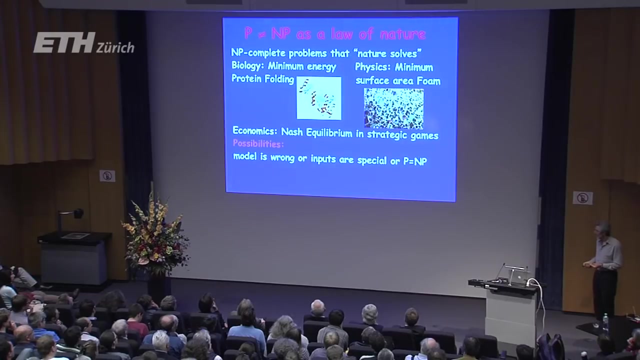 It's NP-complete And nature. well, these societies may find equilibria in various strategic games and so on. So what does it mean? Well, I claim that there are just a few possibilities, And all of them are interesting. One is that maybe the model is wrong. 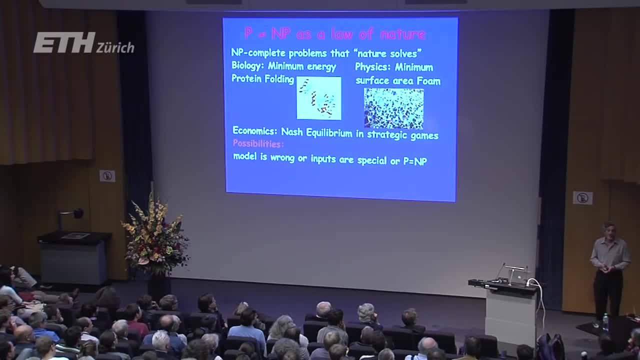 because it suggests that you have an efficient algorithm for a problem that you shouldn't have An efficient algorithm for, Or maybe, which is quite common in many of these situations, the inputs that are faced by nature are not as hard as the worst-case inputs. 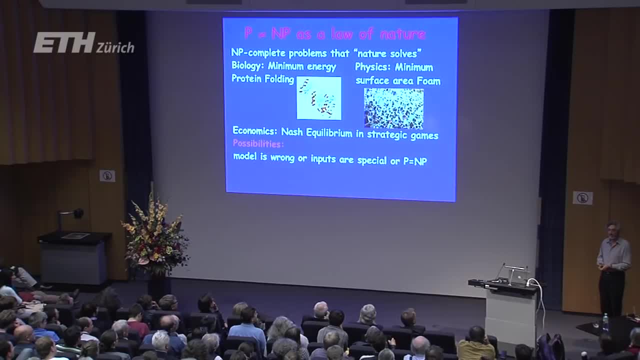 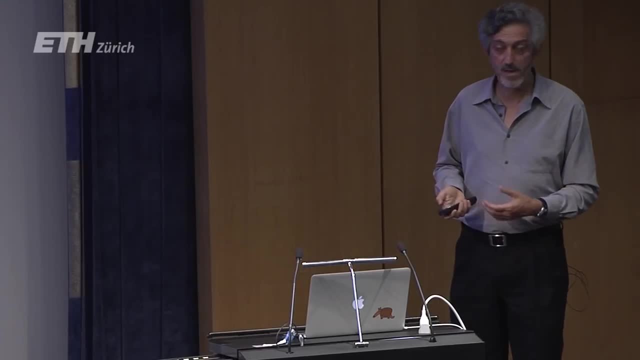 So somehow the inputs are special and you better understand the special structure that allows them to have an efficient algorithm. And the third possibility is that, yeah, this actually suggests that, yeah, there's an efficient algorithm for an NP-complete problem. This means you should improve. 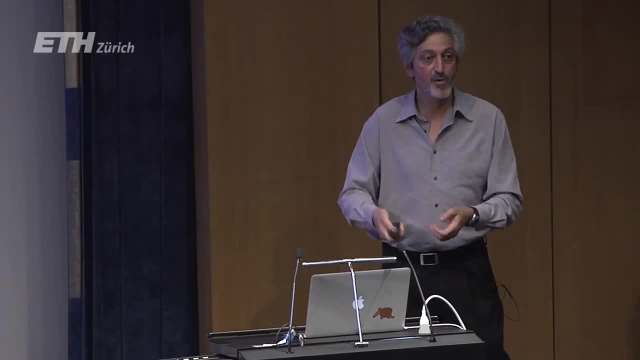 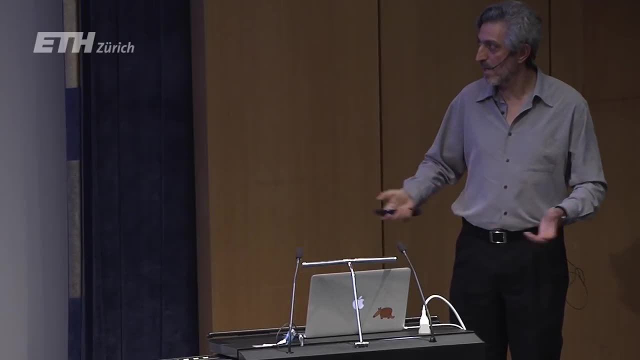 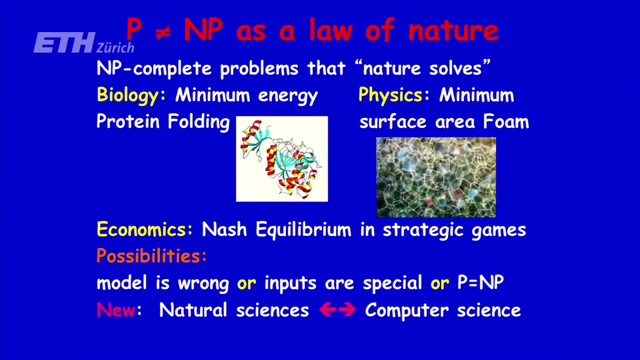 whatever natural system you have into the laptop and it will solve for you many other problems like factor integers. So this starts an interaction between the natural sciences and computer science which is extremely rich, and these boundaries are developing between essentially almost every science and computer science. 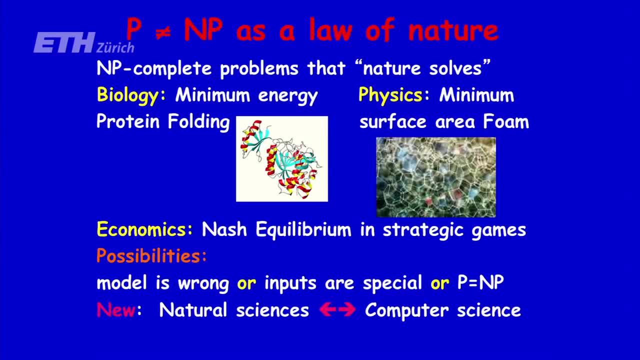 And notice that it's a different interaction than a scientist asking you writing a programmer, please write a program for me. It's much deeper. It's about the science. It's about the modeling of a particular phenomena that integrates computation into it. 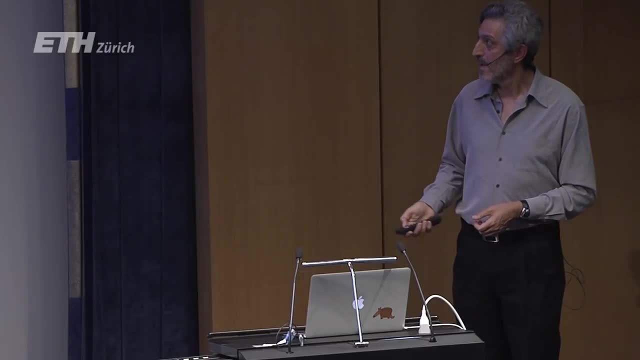 integrates a computational complexity of this phenomena. Okay, so I have to close, So I just want to, as a last slide, talk about the very real possibility that P is different than NP, which I think most people, most computer science, believe. 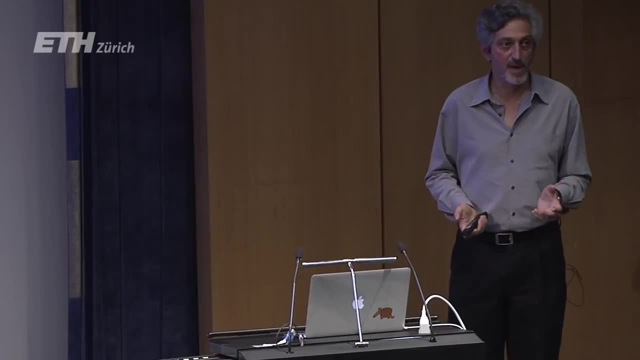 and want to tell you that the fact that they are different is not also bad. Of course it means that lots of problems we cannot solve. but actually it's another remarkable thing: Hard problems, sort of a bad news. we cannot solve this problem. 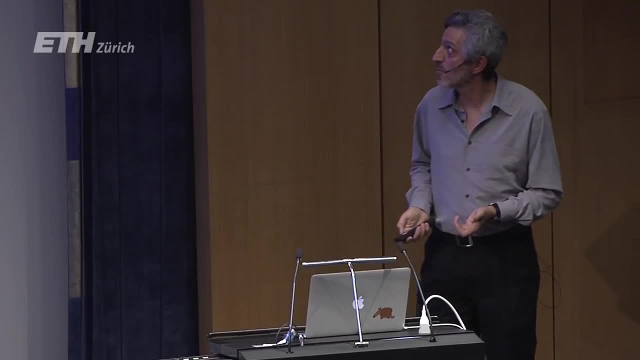 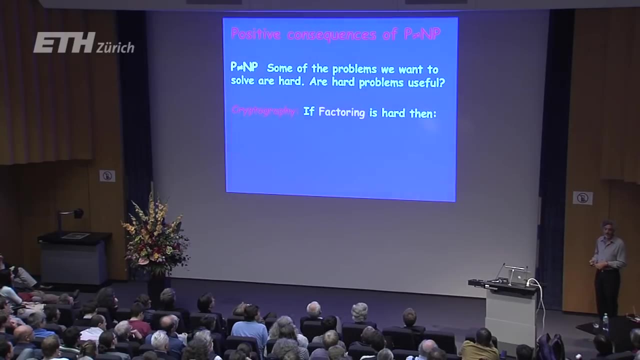 but actually hard problems can be positive news, can be good news. How can it be good news? It can be good news because if particular problems are hard- and factoring is an example- then the fact that they are hard means that we can do magic.